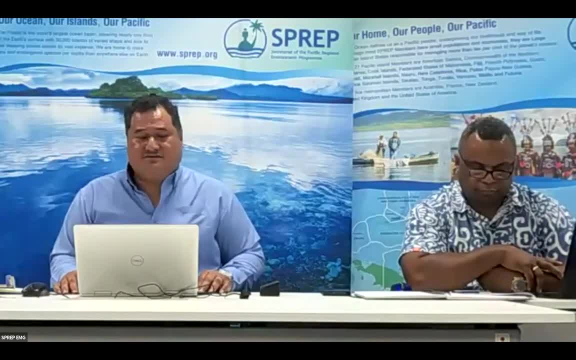 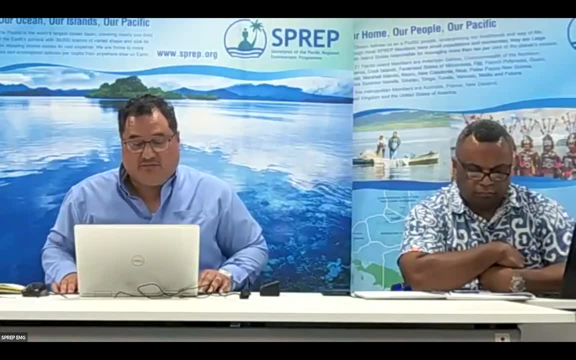 We will attempt to answer two questions. The first is how to prepare responsible terms of reference for EIA studies And, secondly, providing you with guidance tips on the selection and management of consultants. Before I start, I want to acknowledge the President. 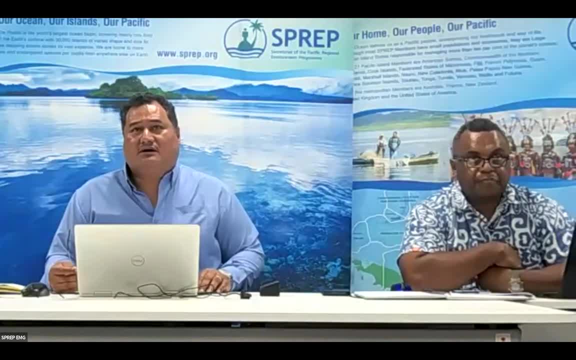 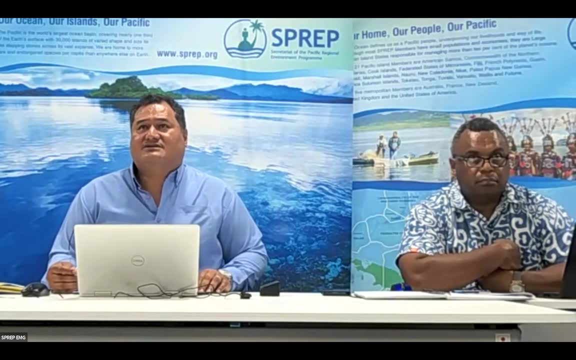 the Vice President of the Acting Director of Environmental and Monitoring Governance in SPREP, Ratu Jopita Manetevalu, and I also want to acknowledge my team leader, Ms Rachel Marburg, who joins us from Sydney, from her home in Sydney. 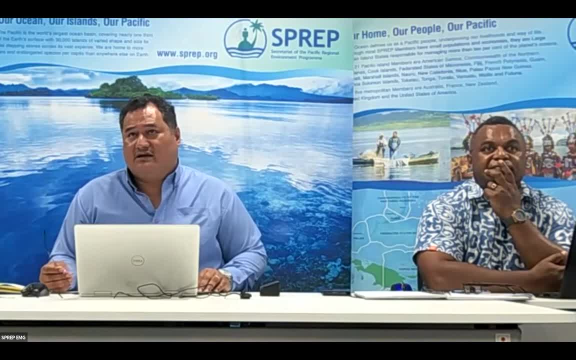 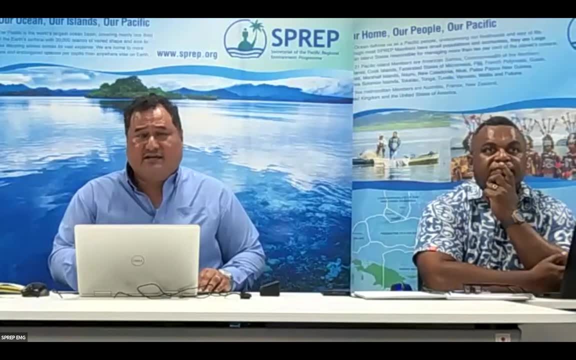 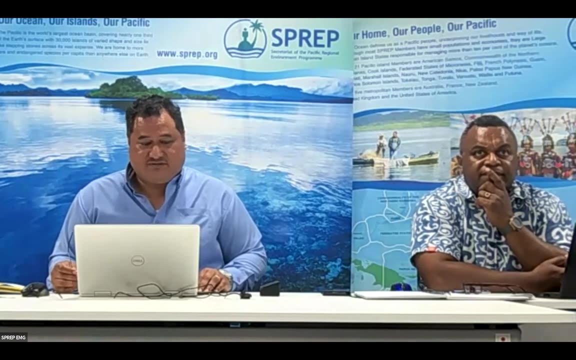 Welcome. Like I said yesterday, every topic that we've designed from the evaluation, there is a narrative behind it underpinning that topic, And so I'll read again out what that is and give you an understanding why we've designed this topic for today. 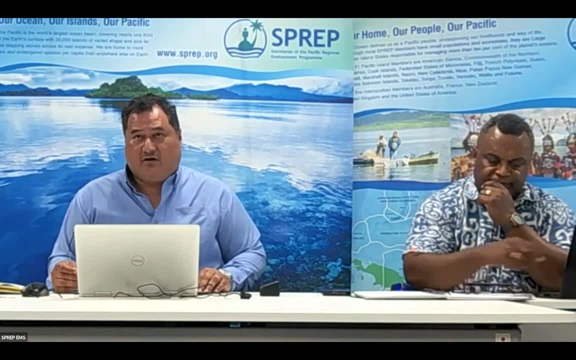 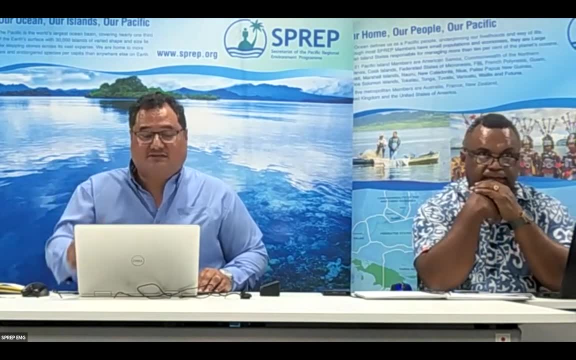 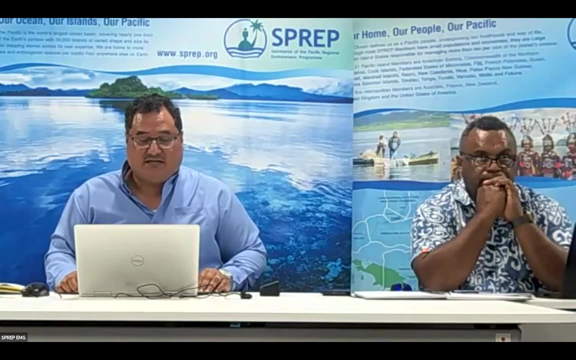 So EIA regulatory agencies in the Pacific often request capacity-building support for developing terms of reference for EIA studies. In most cases, the quality of the EIA report is directly influenced by the constraints of limited qualified and experienced professionals to implement an effective EIA process. So, while screening applications can be a challenge, the EIA report can also be a challenge. So, while screening applications can be a challenge, the EIA report can also be a challenge. So, while screening applications can be a challenge, the EIA report can also be a challenge. 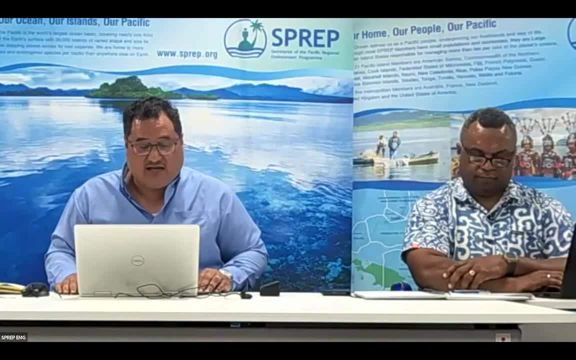 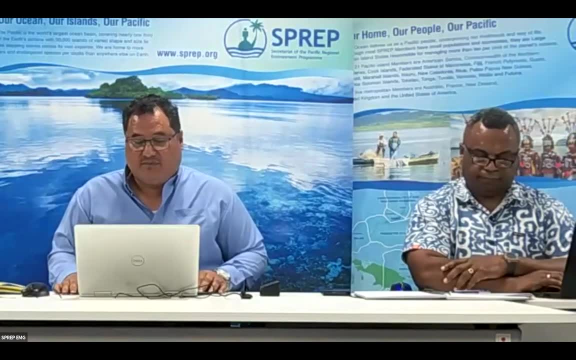 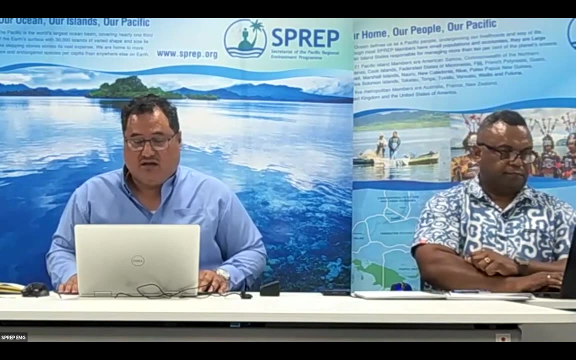 The application for development consent is a critical starting point. Countries do apply different approaches with various struggles. However, both experience and documented requests to spread have shown that many EIA regulators across the Pacific region are requesting assistance for preparing terms of reference for EIA consultants. 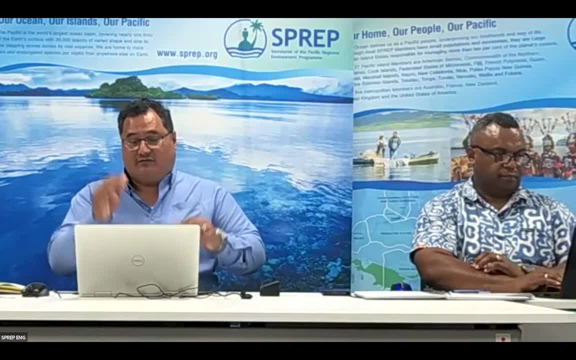 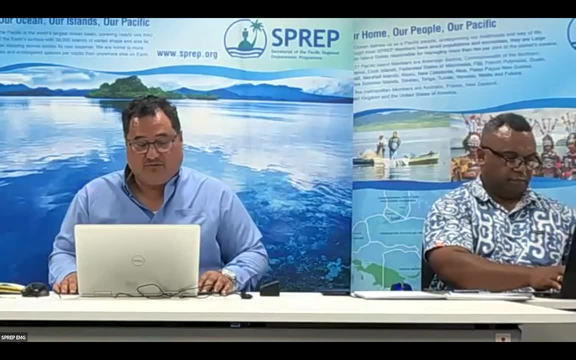 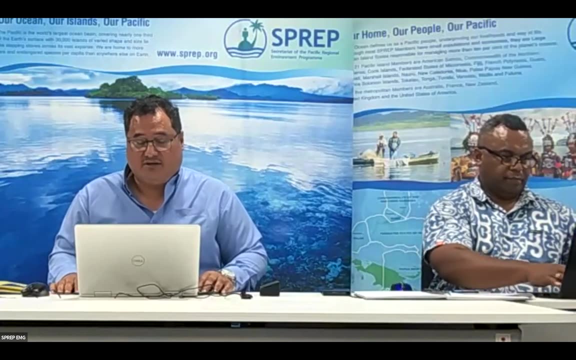 including the structure and format of the EIA report to be aligned with best practice. region and best practice meaning the spread regional eia guidelines that we are promoting in the plp partnership now to address this. this training, this module number 10, will target improvement of your knowledge and skills of staff across eia, regulators and, potentially, 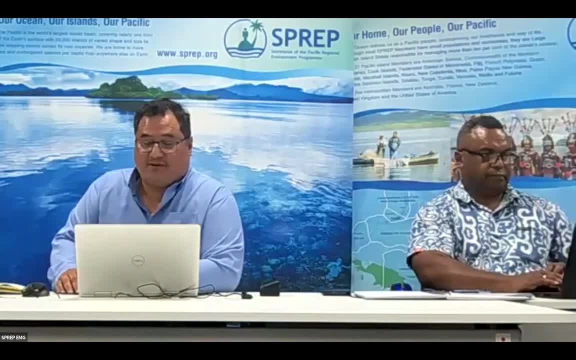 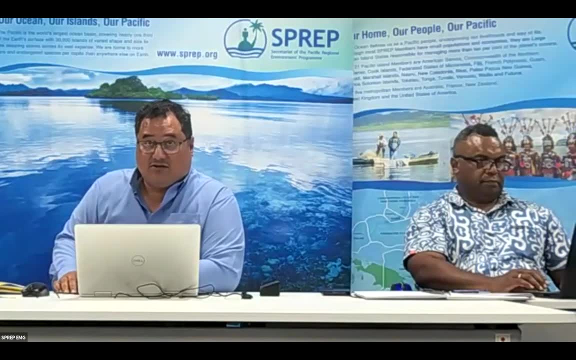 consultants from their private sectors who are engaged to prepare eia studies. we have about three learning objectives, so we hopefully, at the end of this, you will be able to introduce you- uh, you participants- to the key steps of preparing terms of reference for a consultant to carry out. 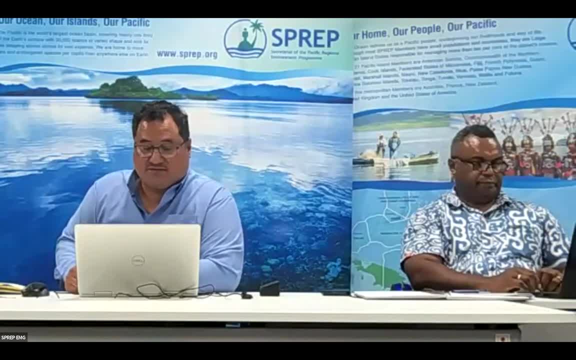 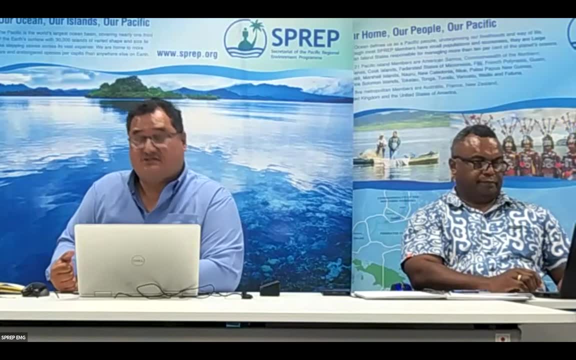 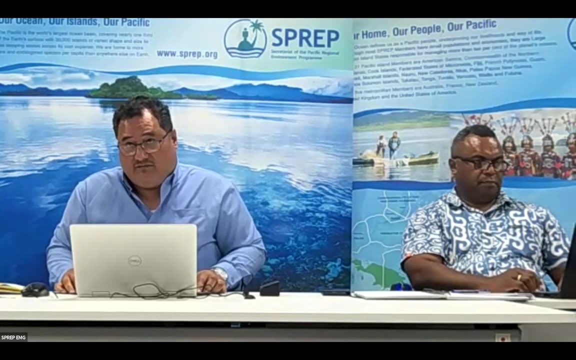 an eia study, we will hopefully explore the usefulness of adopting script's eia report template and, finally, providing advice on how to select consultants with the right set of skills and experience, including managing contracts throughout the eia process. so, without any further ado, i'll hand it over to dr babara, but just before i do that, please use the chat box. 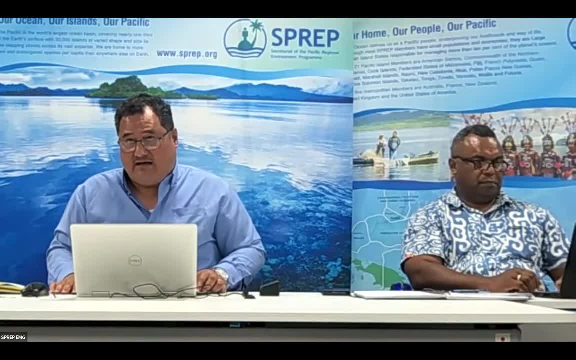 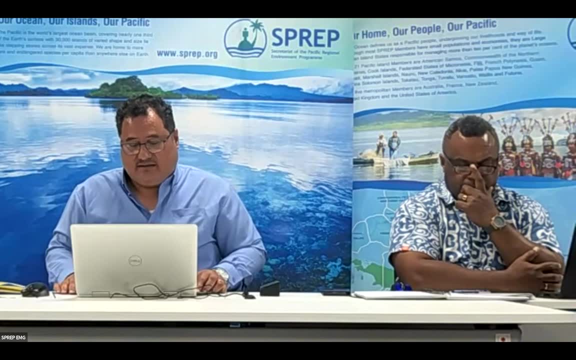 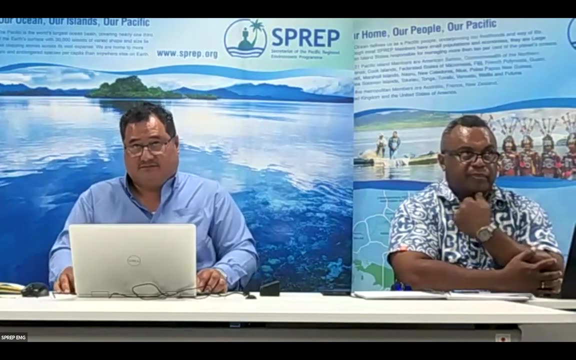 or the raise your hand, would be great to have folks, um, join in with their cameras, uh, to ask questions and then, um, then you know they will, uh, we'll respond to that. so, dr babara, thank you for joining us over to you. thank you, mr maya, and uh, yeah, my pillow, you're looking good there backing. 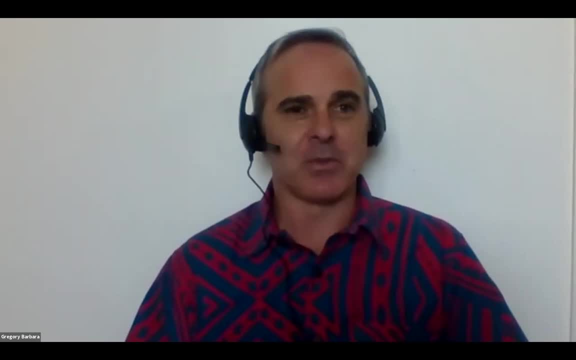 up here. um, i'm actually in brisbane in quarantine, but, uh yeah, sydney, brisbane, it's all good. um, thank you everyone for joining us today. um, as, as my pillow has has explained, we're going to have three main objectives that we're going to look at um. the first one is basically what is scoping and 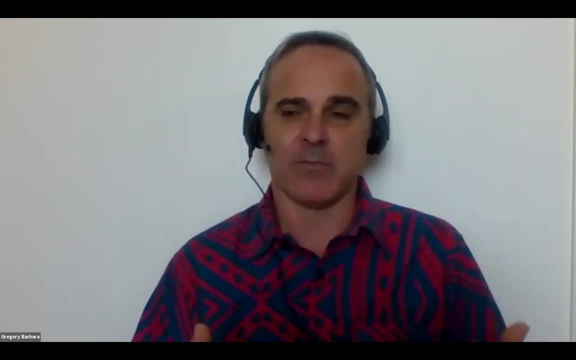 how to do it, the basics of it gonna go. my other panelists will join in and we'll explain more about selecting the right type of consultant team: um for the scoping or for for your project, because that's that's a critical element here. often, um, even if you get 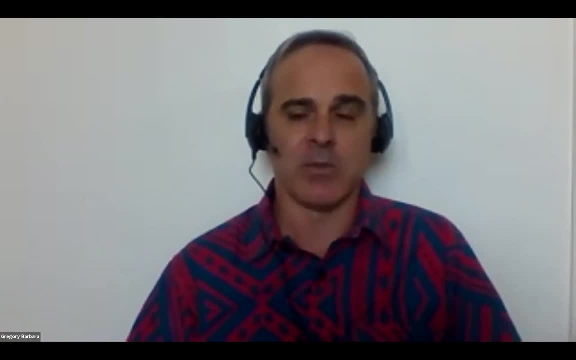 the scoping right. if you get the wrong consultant in the eia is not going to be very good. so bear with me. for those of you who know a lot about scoping and have gone through some sort of scoping capacity building that we've done before, this may seem all same same or very familiar to you. 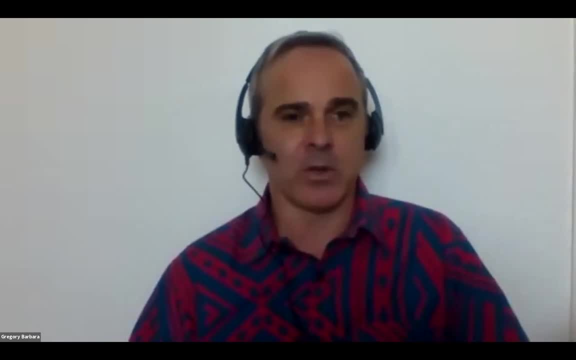 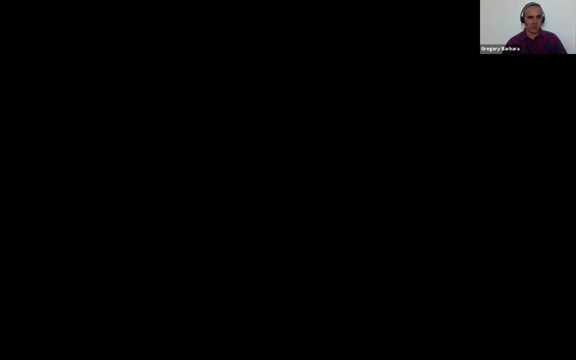 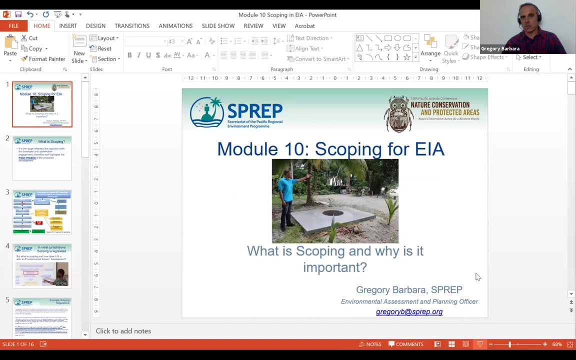 but for those of you who haven't, hopefully this, you pick some stuff up, but we'll be expanding upon it and we're going to be having some talanoas as we go through. so just bear with me while i load up my slides. okay, so if you could just let me know if you can all see those, i'll just take that down. 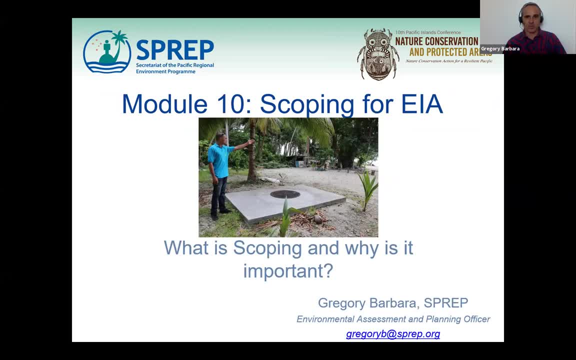 can everybody see my slides? just a thumbs up or something. yep, good, that's all being seen on the screen. um, yeah, apologies if sometimes, um, that, the uh, if you've got your, minimize the video feed, um, if it's obscuring any of the text or any of the information on the slide or dragging the video feed to a corner of the. 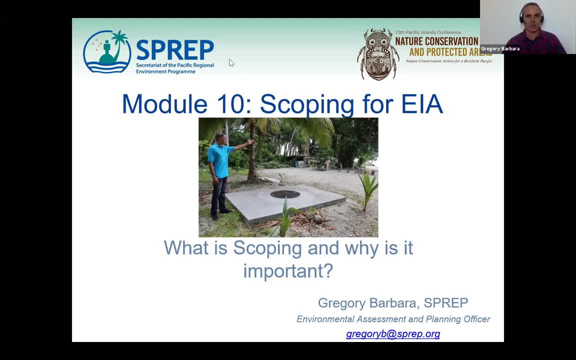 slides. that it's, so it doesn't obscure any of the information, okay, um, without further ado, i'll i'll launch into the presentation. so this is module 10, so okay, or environmental impacts. so uh, uh, uh, uh, uh, uh is is what is coping and um. 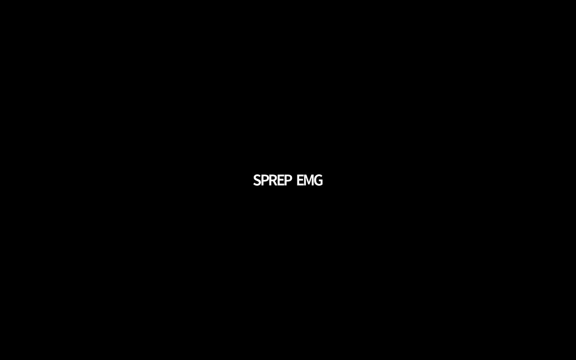 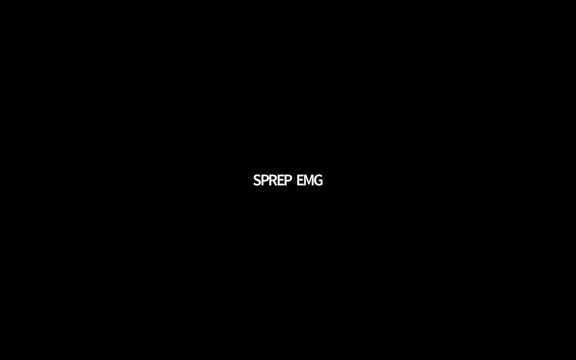 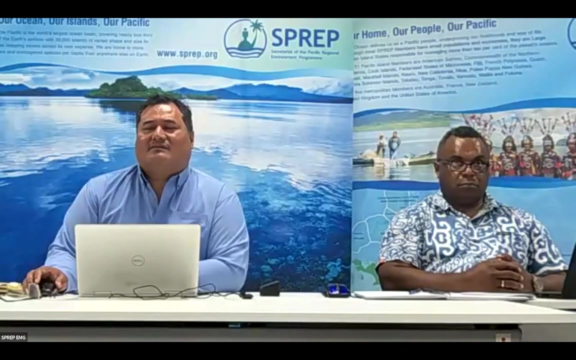 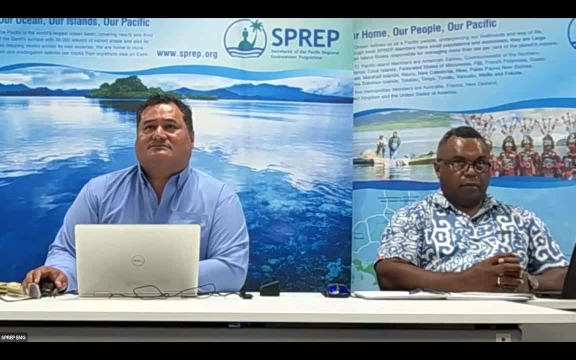 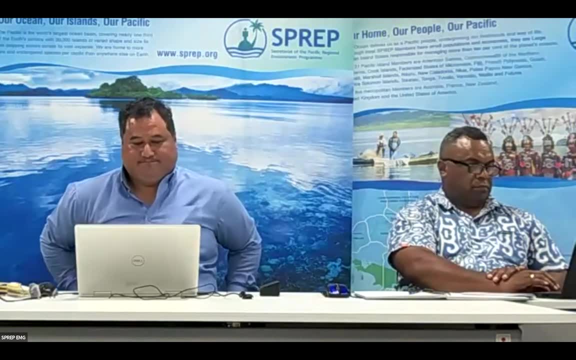 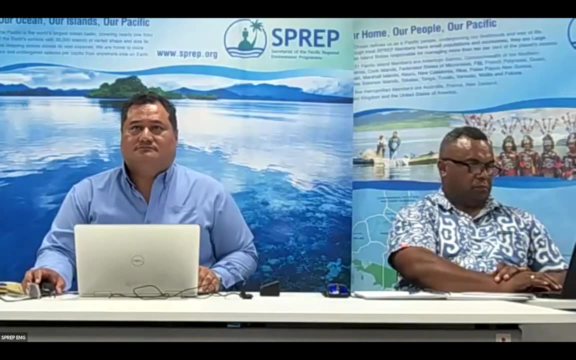 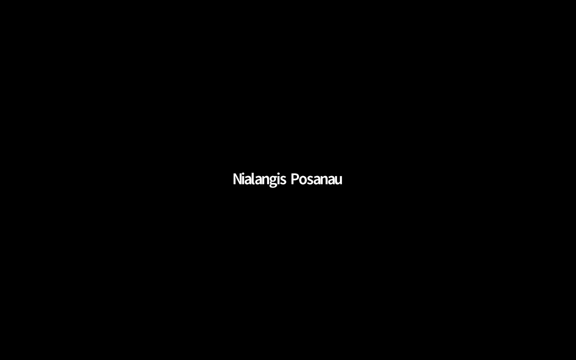 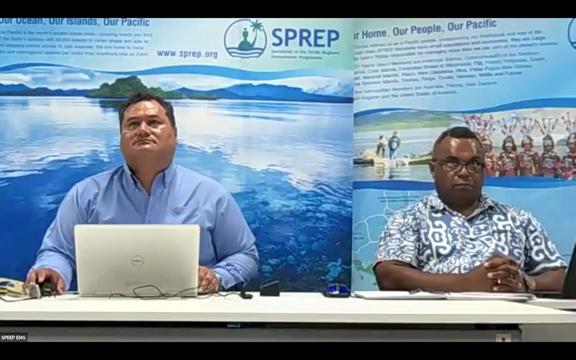 if you can just uh give him a few seconds, ladies and gentlemen, if you can just uh give him a few seconds, ladies and gentlemen, hopefully he'll manage to get on. gentlemen, hopefully he'll manage to get on. just bear with us, i think. um, he's trying to probably connect to. 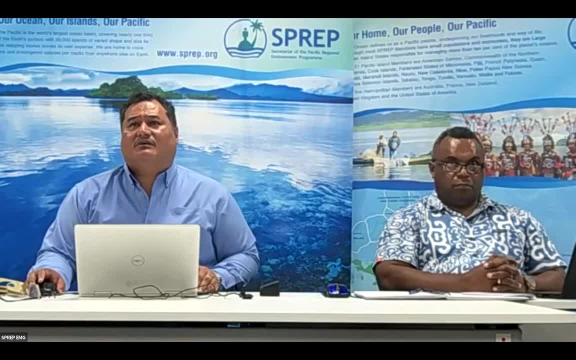 just bear with us. i think, um, he's trying to probably connect to just bear with us. i think, um, he's trying to probably connect to wi-fi. he's uh beaming in uh live from uh wi-fi. he's uh beaming in uh live from uh. 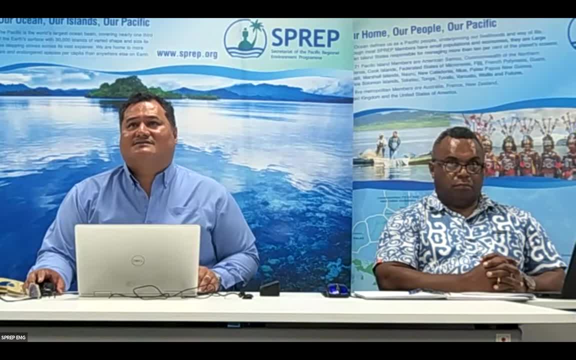 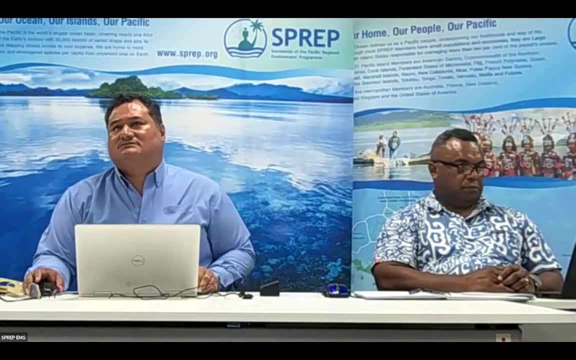 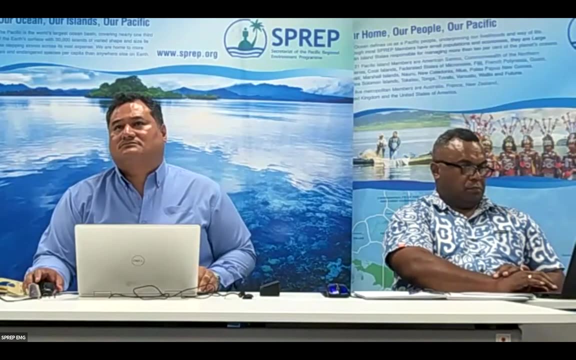 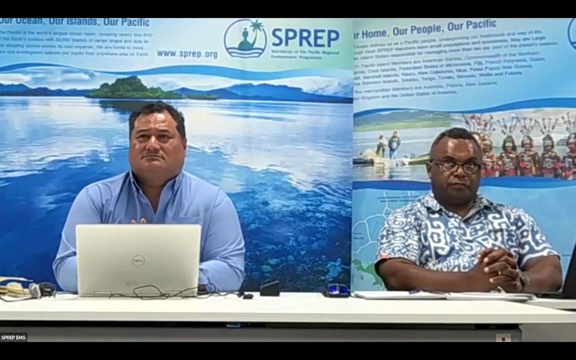 wi-fi. he's uh beaming in, uh live from uh brisbane um brisbane um brisbane, um so, so, so it should be on soon. it should be on soon. it should be on soon. well, while we're ready for greg to, to, to. 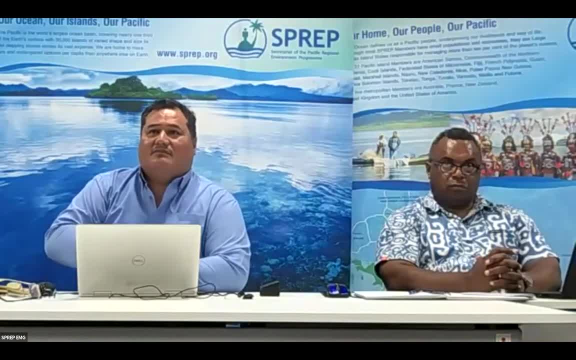 well, while we're ready for greg to to to. well, while we're ready for greg to to to jump in, could i just jump in? could i just jump in? could i just sort of uh, sort of uh, sort of uh. have um, have a um. 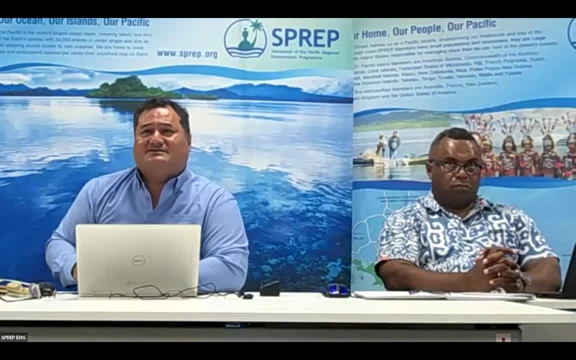 have um, have a um, have um, have a um. few of you guys sort of uh click on. few of you guys sort of uh click on. few of you guys sort of uh click on the uh the hand, but just to see how many the uh the hand, but just to see how many. 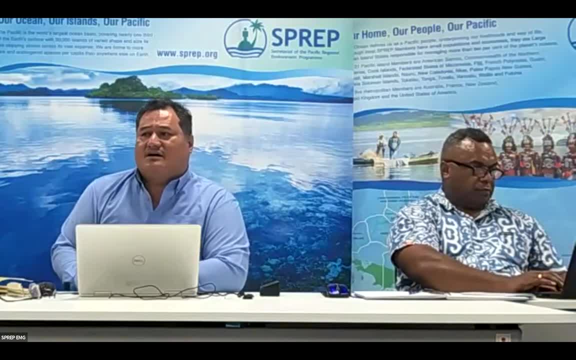 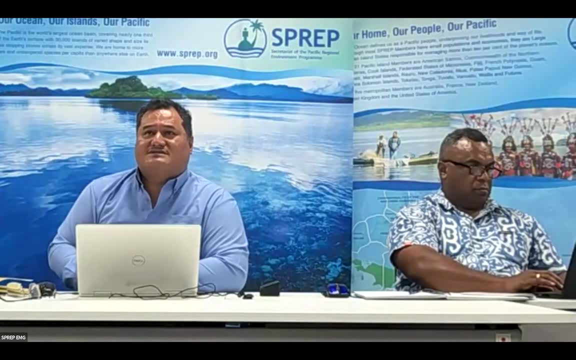 the uh, the hand, but just to see how many of you of you, of you, are actually in a position that is, are actually in a position that is, are actually in a position that is: um, um, um, uh, uh, uh, implementing um, implementing um, implementing um, that is, preparing terms of reference for 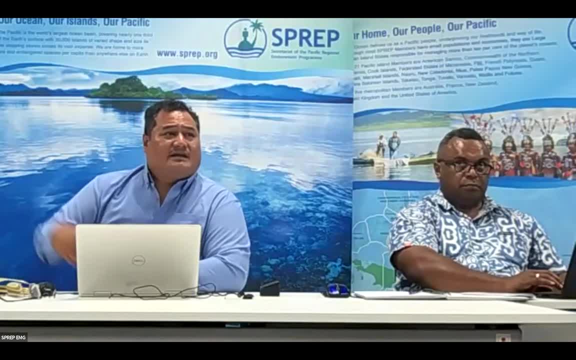 that is preparing terms of reference for that is preparing terms of reference for eia. can you, can you put on your? can you put? can you, can you put on your? can you put? can you, can you put on your? can you put on your video camera while we wait for? 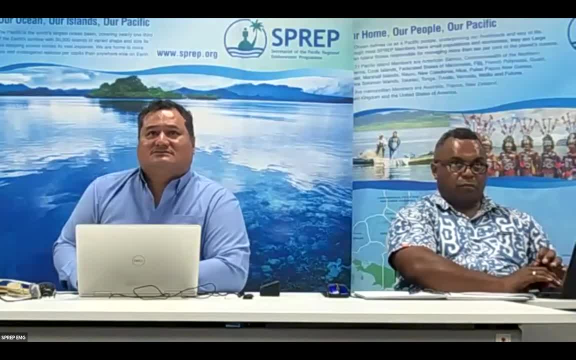 on your video camera while we wait for on your video camera, while we wait for for greg. so we could just have a bit of for for greg. so we could just have a bit of for for greg, so we could just have a bit of a discussion. 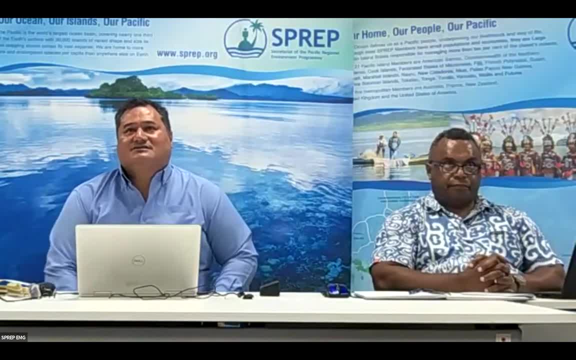 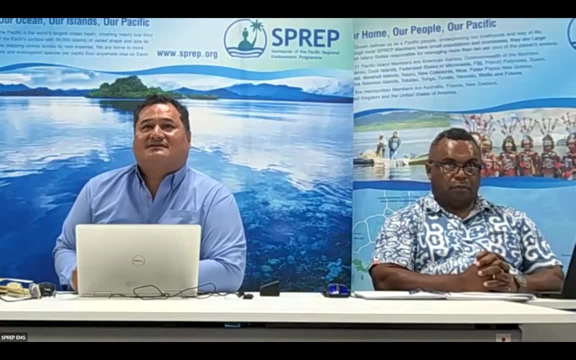 oh nice, so just have your videos, uh, click on, be so, just have your videos, uh, click on, be so, just have your videos, uh, click on, be nice to see all your nice, to see all your nice, to see all your, your lovely faces, your lovely faces, your lovely faces, perhaps. 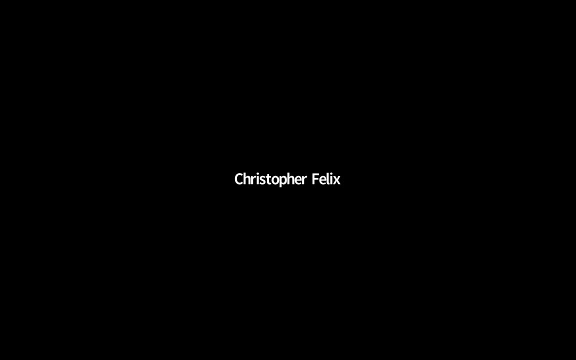 hi everybody, it's very lovely, wow, it's very lovely. wow, it's very lovely. wow, yesterday we had about 60, so right now i. yesterday we had about 60, so right now i. yesterday we had about 60, so right now i can see we have about. 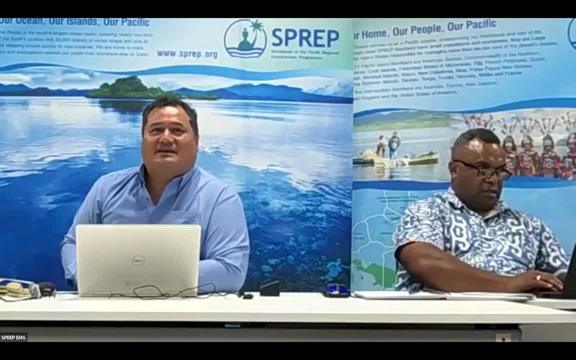 can see we have about. can see we have about 50.. so hopefully we've got an extra 10- 50.. so hopefully we've got an extra 10- 50.. so hopefully we've got an extra 10 or 11, even if it's just one more, just to. 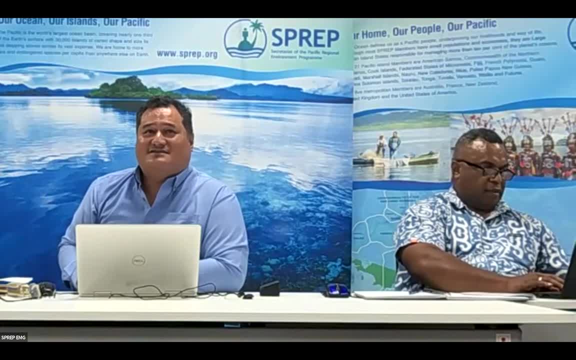 or 11, even if it's just one more just to, or 11, even if it's just one more, just to get us over the 60 mark. get us over the 60 mark, get us over the 60 mark, that'll be great. you know, this is a you. 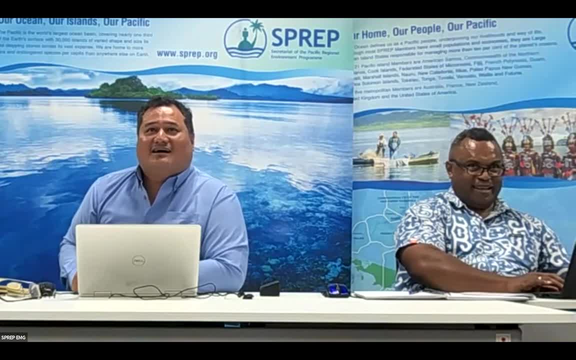 that'll be great. you know this is a you. that'll be great. you know this is a you. know we're competing from one session to know we're competing from one session to know we're competing from one session to another, another, another. so i think we might need to talk. we ask: 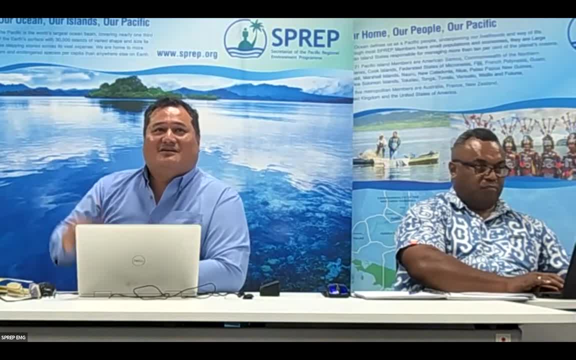 so i think we might need to talk. we ask, so i think we might need to talk. we ask brett, and will bank to come up with brett, and will bank to come up with brett, and will bank to come up with some sort of a certificate on uh. 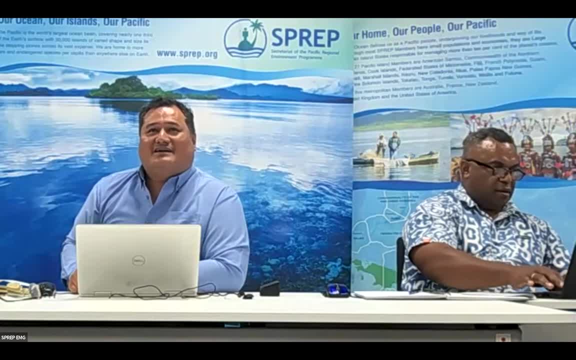 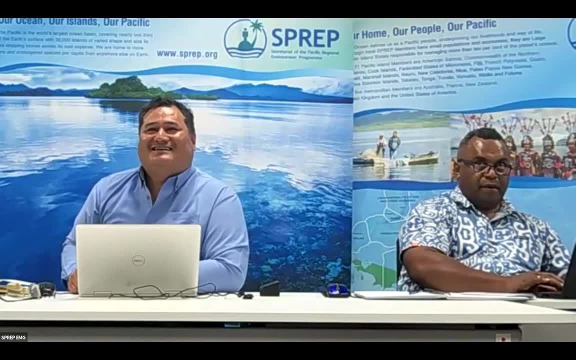 some sort of a certificate on uh, some sort of a certificate on uh on the best uh on the best, uh on the best uh module, with the highest participation module, with the highest participation module, with the highest participation. all right, so uh, how many of you guys actually uh? 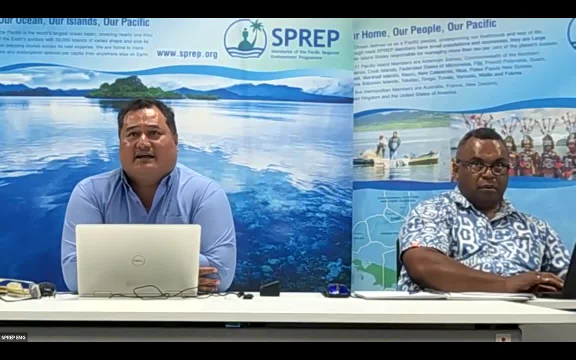 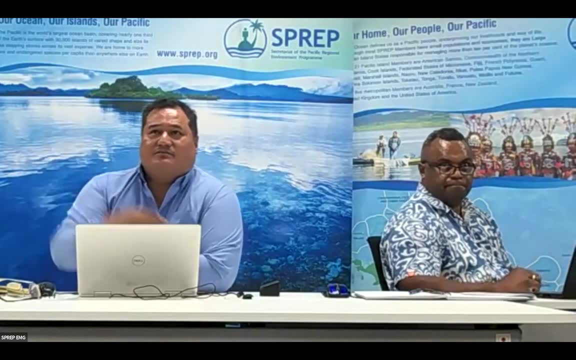 so, uh, how many of you guys actually uh? so, uh, how many of you guys actually, uh, are doing eia, preparing in terms of are doing eia, preparing in terms of are doing eia, preparing in terms of reference for eia? maybe you could, maybe you could uh. 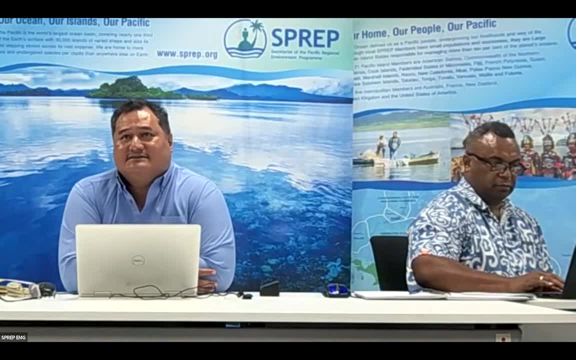 maybe you could, maybe you could uh, maybe you could. maybe you could uh, unmute and just sort of have a unmute and just sort of have a unmute and just sort of have a discussion, discussion, discussion while we, while we wait for greg, while we, while we wait for greg. while we, while we wait for greg, it'll be really good to sort of learn a. it'll be really good to sort of learn a. it'll be really good to sort of learn a bit more about you. this is still these. bit more about you. this is still these. 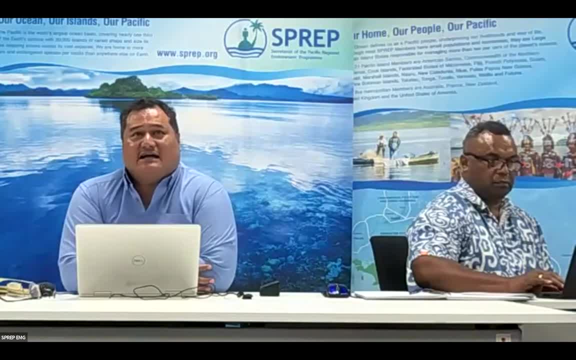 bit more about you. this is still these sort of things. tapping guys are willing to share. your tapping guys are willing to share. your tapping guys are willing to share your thoughts about you. know about the thoughts about you know about the thoughts about you. know about the experiences you do you, you confront with 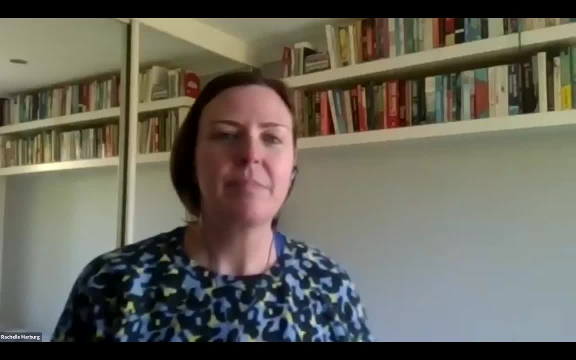 experiences. you do you you confront with experiences? you do you you confront with developing terms of reference for eia, developing terms of reference for eia, developing terms of reference for eia: hi mia pello, hi mia pello, hi mia pello. would it be okay if i just 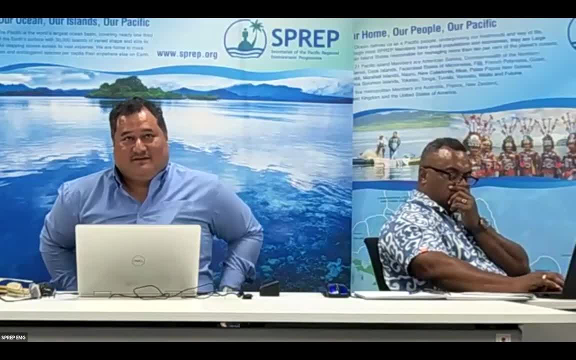 would it be okay if i just? would it be okay if i just start a conversation? great, thank you hi everybody um really great. thank you hi everybody um really great. thank you hi everybody um really appreciate you joining again. it's great. appreciate you joining again. it's great. 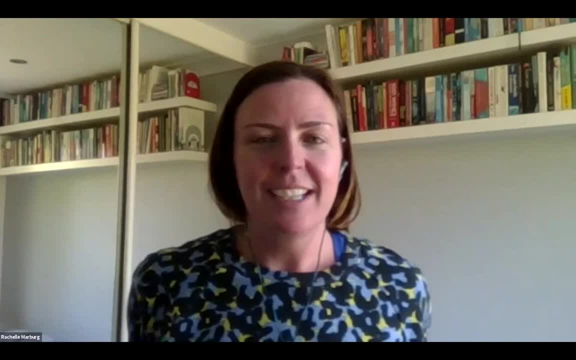 appreciate you joining again. it's great to see so many faces. i haven't been to to see so many faces. i haven't been to to see so many faces. i haven't been to the pacific for the pacific for the pacific for well too long now and i'm really missing. 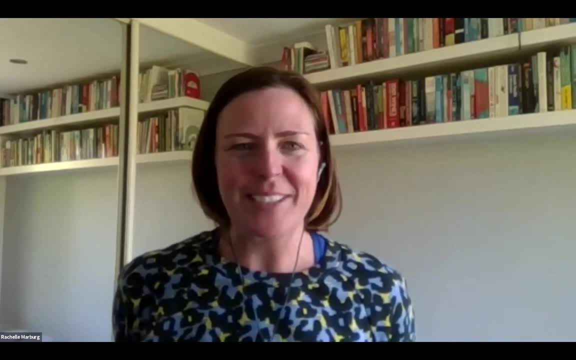 well too long now and i'm really missing well too long now and i'm really missing uh all the faces and and the people in uh all the faces and and the people in uh all the faces and and the people in the pacific. so thanks for having your. 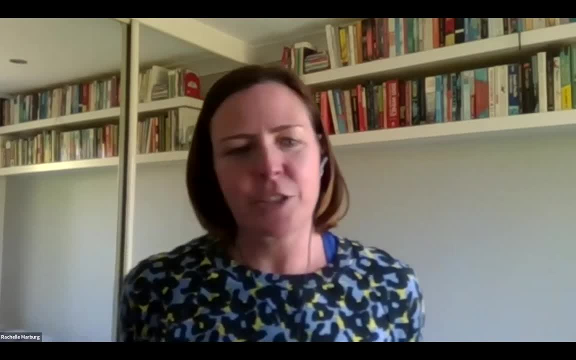 the pacific. so thanks for having your the pacific, so thanks for having your cameras on cameras, on cameras on um. just a really short reflection on um, just a really short reflection on um, just a really short reflection on, on terms of reference. to reiterate, i: 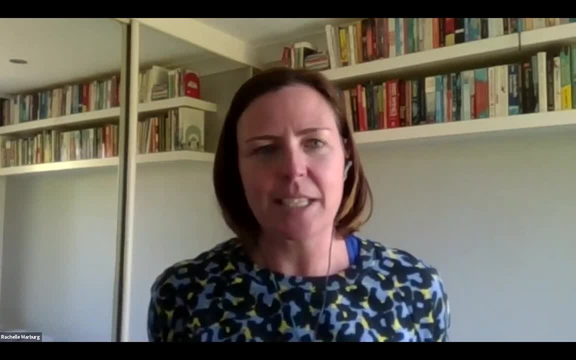 on terms of reference, to reiterate, i. on terms of reference, to reiterate, i think- what greg was starting to say and think what greg was starting to say and think what greg was starting to say, and perhaps the experience that many of you, perhaps the experience that many of you, 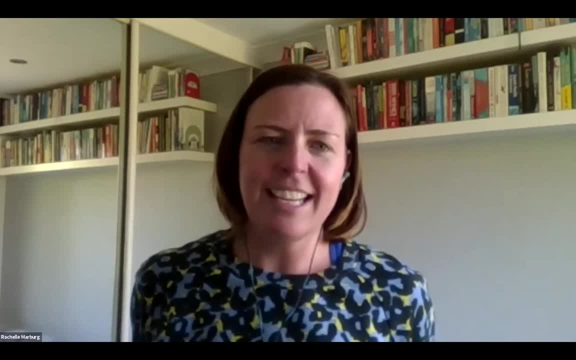 perhaps the experience that many of you have have have. it takes a lot longer than you think, and it takes a lot longer than you think and it takes a lot longer than you think and it's really important, it's really important, it's really important to to do that thinking for terms of 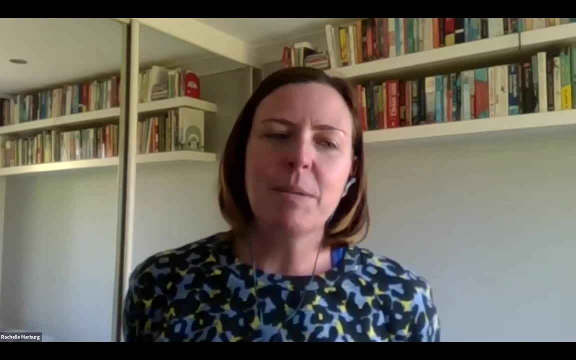 to. to do that thinking, for terms of to, to do that thinking for terms of reference for an impact assessment, or in reference for an impact assessment, or in reference for an impact assessment, or, in fact, anything, simply because that that starts the. simply because that that starts the. 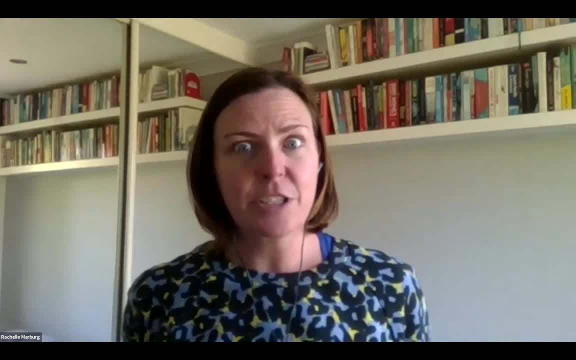 simply because that that starts the process. it defines the effort, it makes process. it defines the effort. it makes process. it defines the effort. it makes people think about key issues. it makes people think about key issues. it makes people think about key issues. it makes you think about. 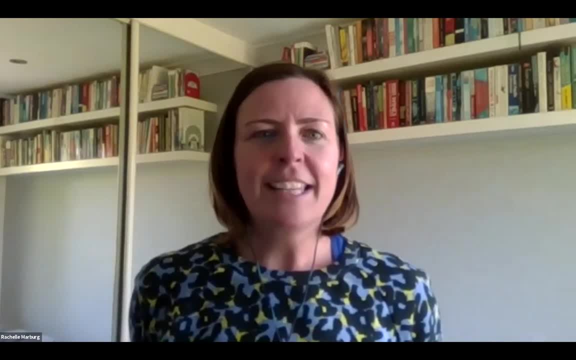 you think about. you think about the skills you need to do this. work it the skills you need to do this. work it the skills you need to do this. work it. makes you think about, makes you think about, makes you think about the relationship between different parts, the relationship between different parts. 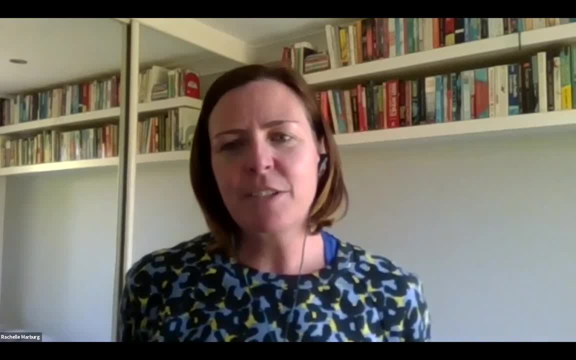 the relationship between different parts of a project or a program or a study of a project or a program, or a study of a project or a program or a study, and it makes you understand the kinds of, and it makes you understand the kinds of and it makes you understand the kinds of questions that you have. 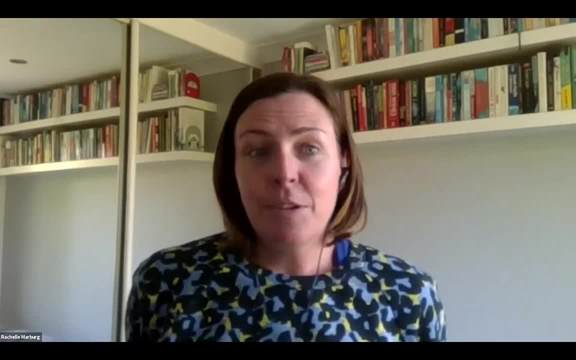 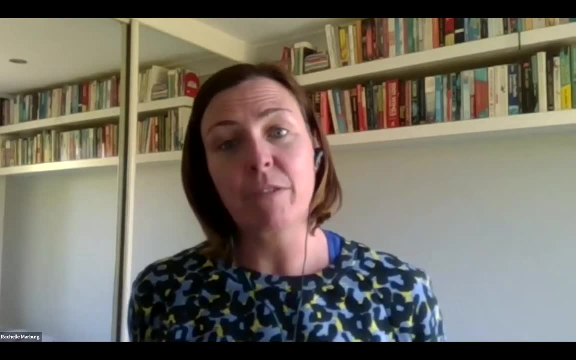 questions that you have, questions that you have, not just that you have fulfilled your, not just that you have fulfilled your, not just that you have fulfilled your terms of reference, or that you have a terms of reference, or that you have a terms of reference or that you have a report, but 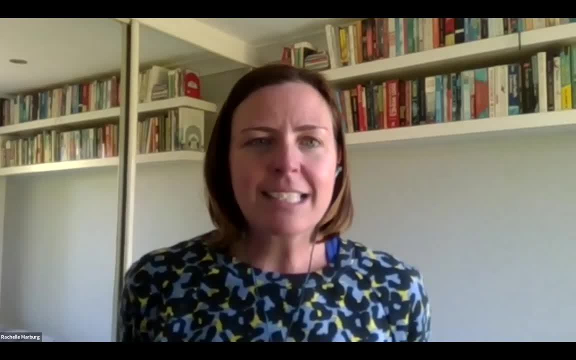 report, but report, but you're really trying to understand, you're really trying to understand, you're really trying to understand. you know the answers to questions, that you know the answers to questions, that you know the answers to questions that you're seeking through this process and you're seeking through this process, and 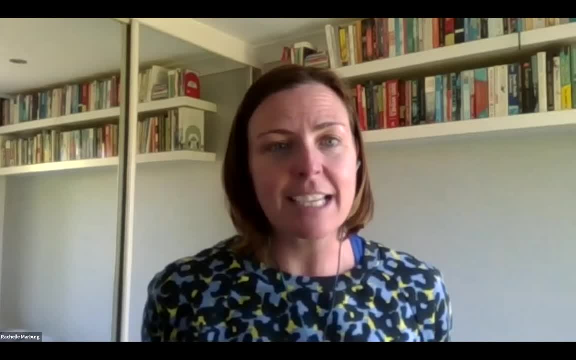 you're seeking through this process and this is a really important step in doing this, is a really important step in doing this, is a really important step in doing this. so it really does this, so it really does this, so it really does deserve some thinking and a bit of. 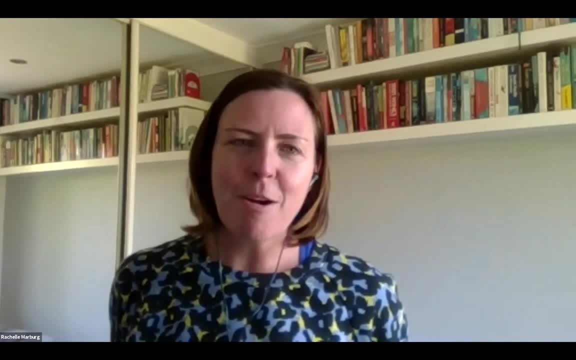 deserve some thinking and a bit of deserve some thinking and a bit of attention right at the front, and i can attention right at the front and i can attention right at the front and i can tell you from my own experience that it's tell you from my own experience that it's. 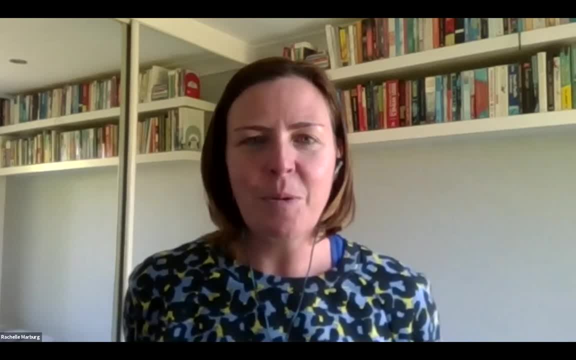 tell you from my own experience that it's very easy to take a generic terms of very easy to take a generic terms of very easy to take a generic terms of reference, reference, reference, or one that you've used before or one, or one that you've used before or one. 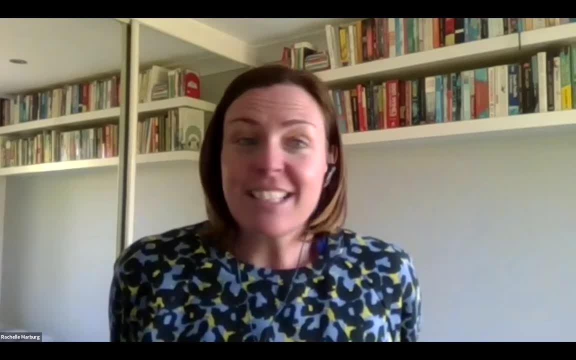 or one that you've used before, or one that somebody like me has sent you from that somebody like me has sent you from that somebody like me has sent you from the bank, the bank, the bank, and to think that that's okay, that's, and to think that that's okay, that's. 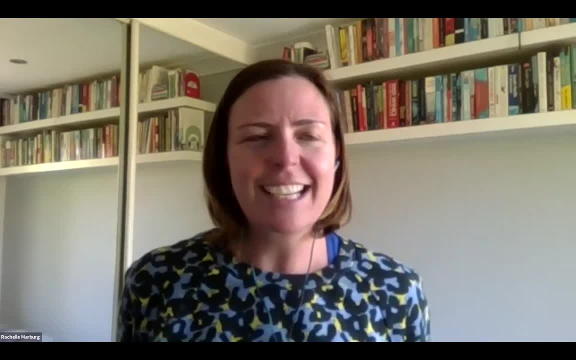 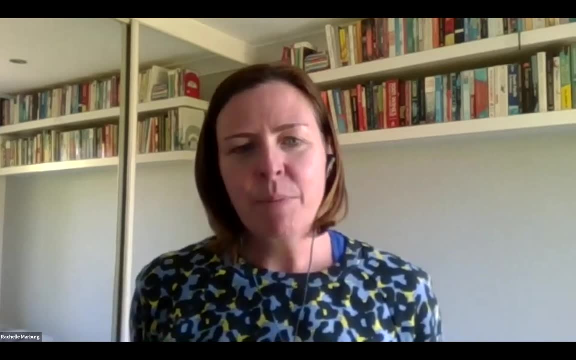 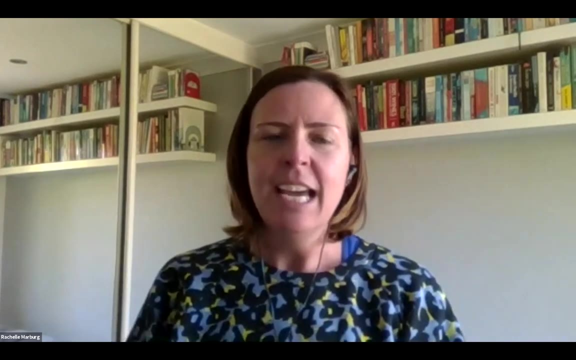 and to think that that's okay, that's good enough, or that good enough, or that good enough, or that yeah, that will do, because of course you're yeah, that will do, because of course you're yeah, that will do, because of course you're how you think about these questions. 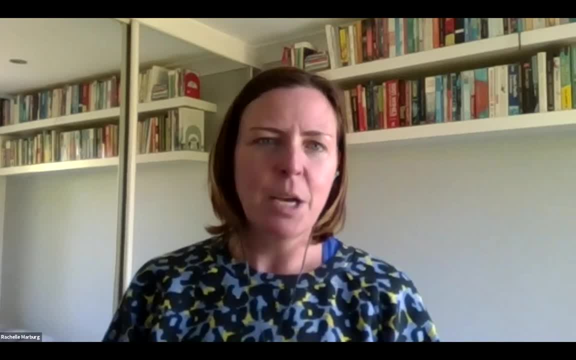 how you think about these questions. how you think about these questions is really, really important, and not every is really really important and not every is really really important, and not every scoping exercise- scoping exercise, scoping exercise will be the same. it won't involve the 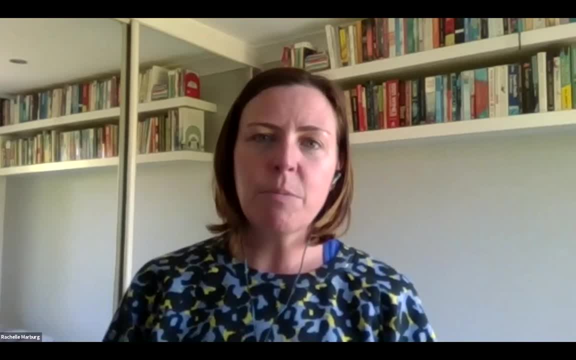 will be the same. it won't involve the will be the same. it won't involve the same people or the same issues, or the same people or the same issues, or the same people or the same issues or the same topics- same topics, same topics. it really will depend on what you're. 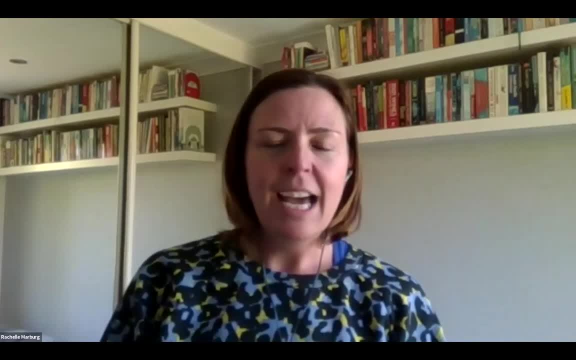 it really will depend on what you're. it really will depend on what you're building, what you're doing, building what you're doing, building what you're doing, where you are and who is around you where you are and who is around you. where you are and who is around you, what are the? 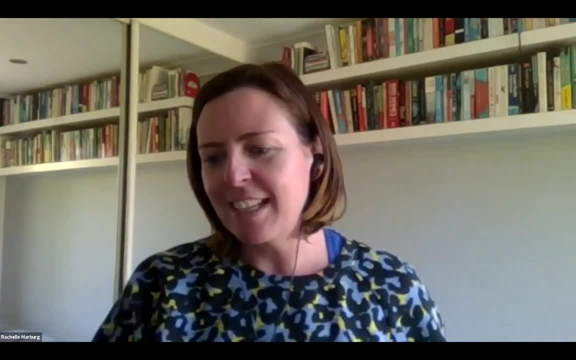 what are the? what are the? what is the context you're working in? so what is the context you're working in? so what is the context you're working in? so i, i would just really um, i, i would just really um, i, i would just really um reiterate what greg was saying: that it's 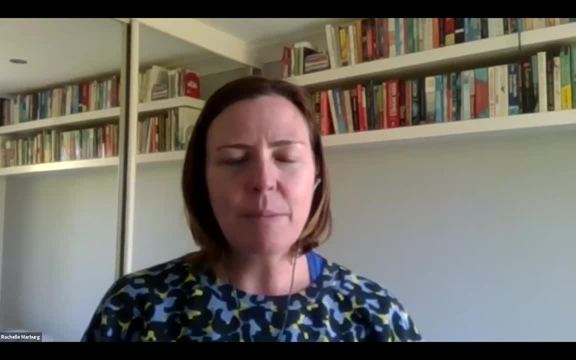 reiterate what greg was saying, that it's reiterate what greg was saying: that it's a really important process and it a really important process and it a really important process and it really helps set up the whole rest of, really helps set up the whole rest of. 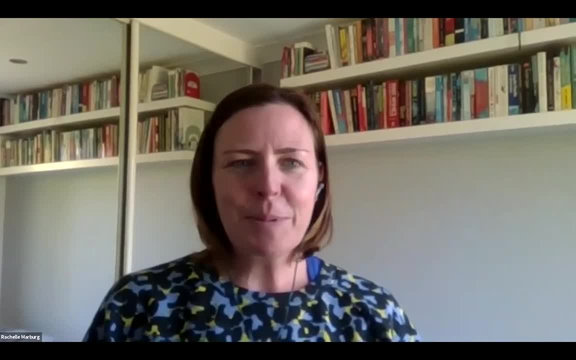 really helps set up the whole rest of your programming as your programming, as your programming, as as you go forward, so i'll stop. i'm as you go forward, so i'll stop. i'm as you go forward, so i'll stop. i'm happy to hand over to somebody else to 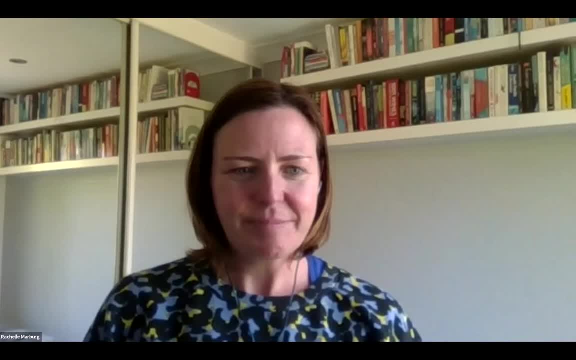 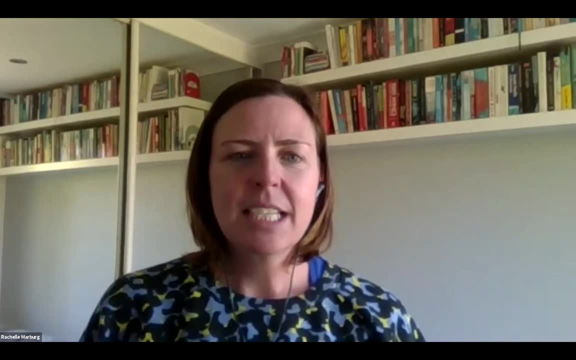 happy to hand over to somebody else to happy to hand over to somebody else to share their thoughts. share their thoughts. share their thoughts. sorry about that, thanks, rachel. that was sorry about that. thanks, rachel, that was sorry about that. thanks, rachel, that was uh, that was excellent good. 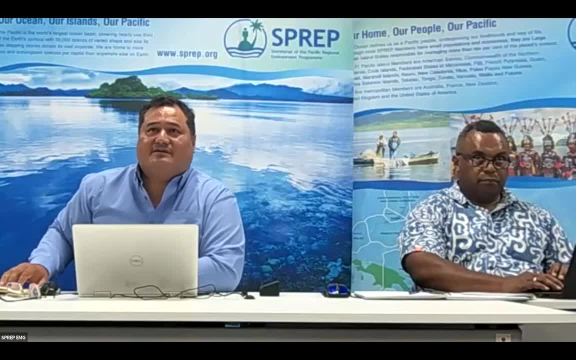 uh, that was excellent, good, uh, that was excellent, good, good, uh, good comment. anybody else wishes good, uh, good comment. anybody else wishes good, uh, good comment. anybody else wishes to share their, their thoughts about the? to share their, their thoughts about the. to share their, their thoughts about the, the eia. you know the issues, or that you? 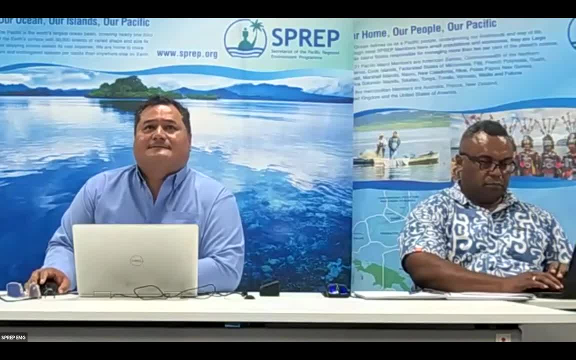 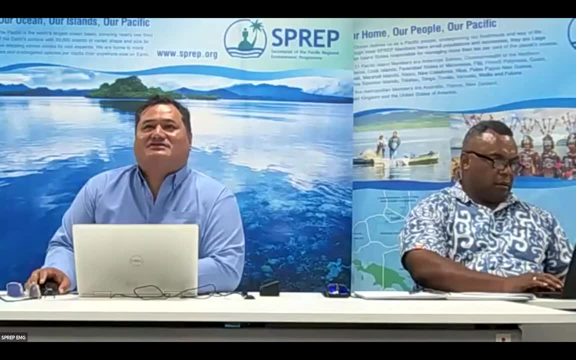 the eia, you know the issues, or that you, the eia, you know the issues, or that you confirm with preparing eia. terms of confirm with preparing eia. terms of confirm with preparing eia. terms of reference perhaps. uh, everybody's a bit shy in the. 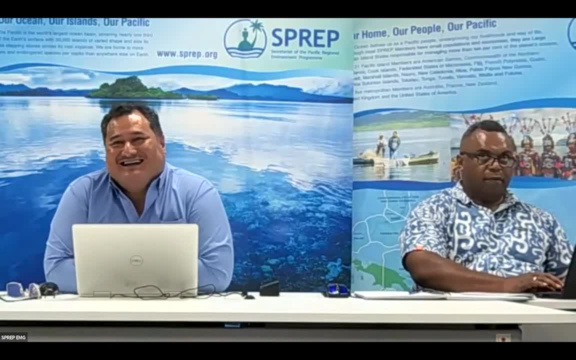 perhaps uh, everybody's a bit shy in the, perhaps uh, everybody's a bit shy in the beginning, beginning, beginning, okay, okay, okay, but um, i mean i just want to also uh, but um, i mean i just want to also uh, but um, i mean i just want to also uh chime in because- and i think a lot- the. 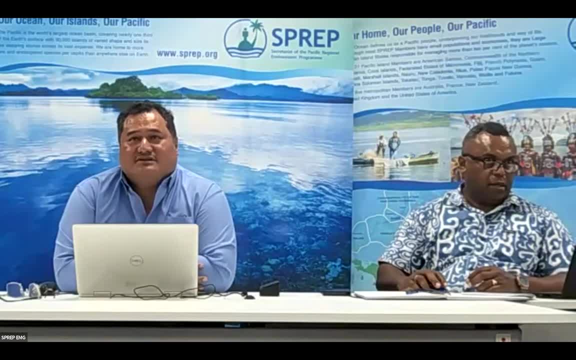 chime in because, and i think a lot the chime in because, and i think a lot, the reason why a lot of folks have reason why a lot of folks have, reason why a lot of folks have uh pointed to this issue, is because uh pointed to this issue is because 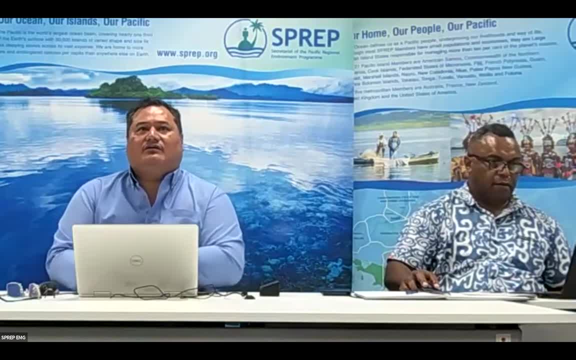 uh pointed to this issue is because you know, in many cases, the quality of you know, in many cases, the quality of you know in many cases, the quality of the eia report and every other- the eia report- and every other- the eia report- and every other instruments that come after that- the 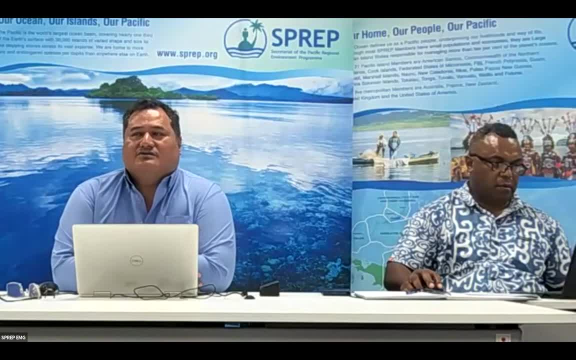 instruments that come after that, the instruments that come after that, the monitoring, the management plans, that monitoring the management plans, that monitoring the management plans that come after that, come after that, come after that- are uniquely tied in with how well you are, uniquely tied in with how well you. 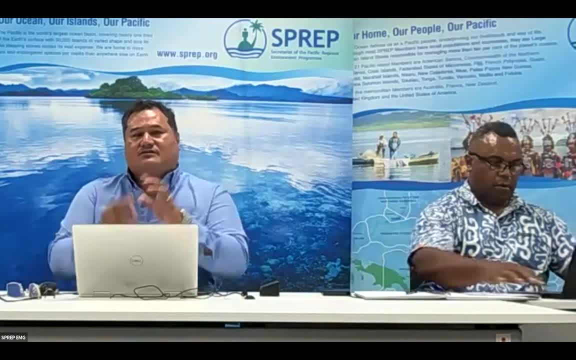 are uniquely tied in with how well you you prepare terms of reference and like you prepare terms of reference and like you prepare terms of reference and like rachel mentioned, it's sort of like a rachel mentioned. it's sort of like a rachel mentioned, it's sort of like a starting point where you pause and 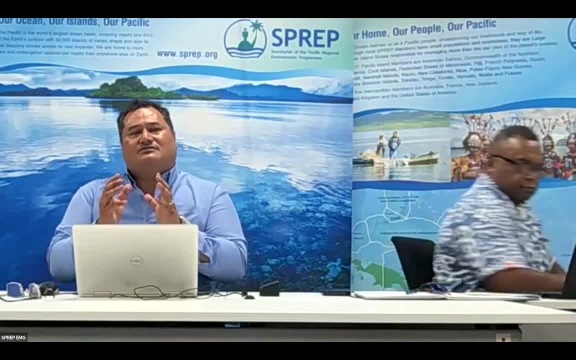 starting point where you pause, and starting point where you pause and reflect, reflect, reflect, and you really it's it's not meant to in and you really it's it's not meant to in and you really it's it's not meant to. in my view, from my own experience, not. 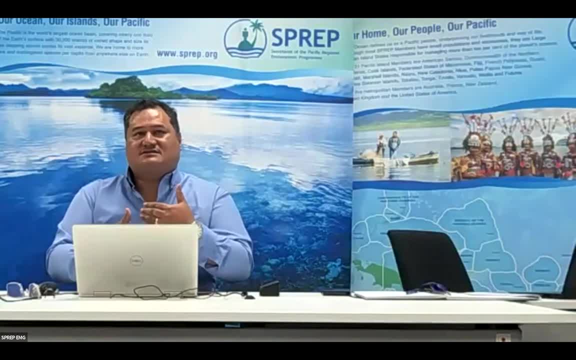 my view, from my own experience, not my view from my own experience. not meant to be very quick, meant to be very quick, meant to be very quick. there is a process, uh, in itself, and it's there is a process, uh, in itself, and it's. there is a process, uh, in itself, and it's meant to really flesh out, not just to 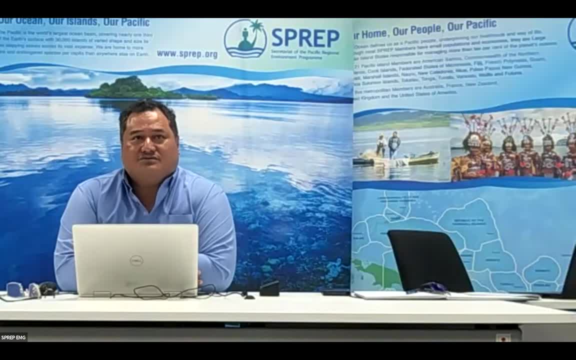 meant to really flesh out, not just to meant to really flesh out, not just to identify, but really flesh out the sort, identify but really flesh out the sort identify but really flesh out the sort of issues in terms of risks and impacts, of issues in terms of risks and impacts. 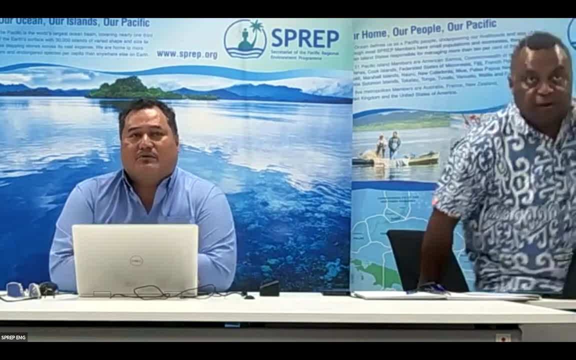 of issues in terms of risks and impacts. that's going to be associated with that. that's going to be associated with that. that's going to be associated with that particular development proposal, that particular development proposal, that particular development proposal that you've been asked to review, you know, and 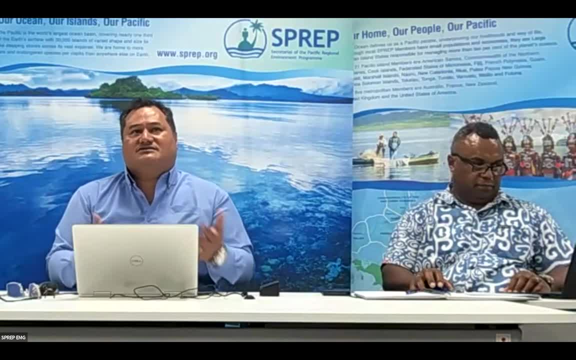 you've been asked to review, you know, and you've been asked to review, you know, and so like, every project is different, in so like every project is different, in so like every project is different in scale and scope, and of course you know scale and scope, and of course you know. 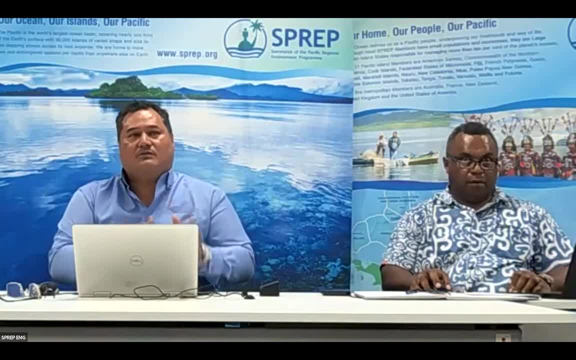 scale and scope and, of course, you know every uh in terms of references are not every uh in terms of references are not every uh in terms of references are not exactly the same for one project, or exactly the same for one project, or exactly the same for one project or another. 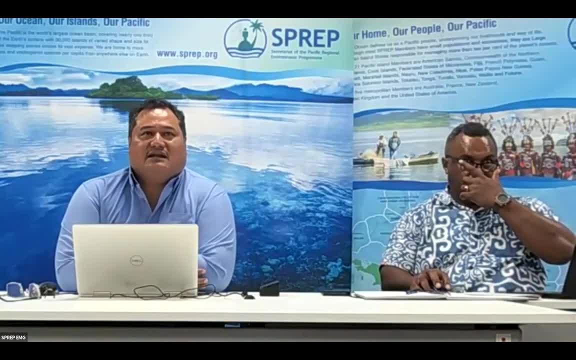 another, another, but i do want to point out particularly, but i do want to point out particularly, but i do want to point out particularly, the most, one of the most important, the most, one of the most important, the most, one of the most important things that i find is that 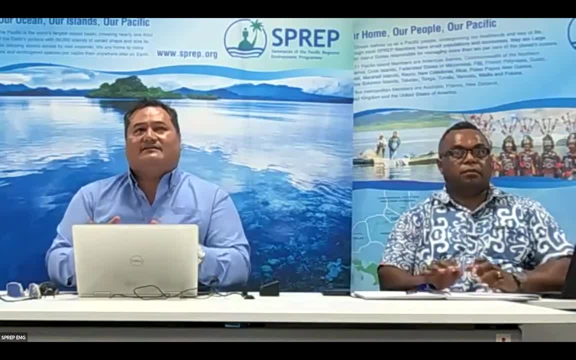 things that i find is that things that i find is that you need to have the right set of talent. you need to have the right set of talent. you need to have the right set of talent, the right set of people with the, the right set of people with the. 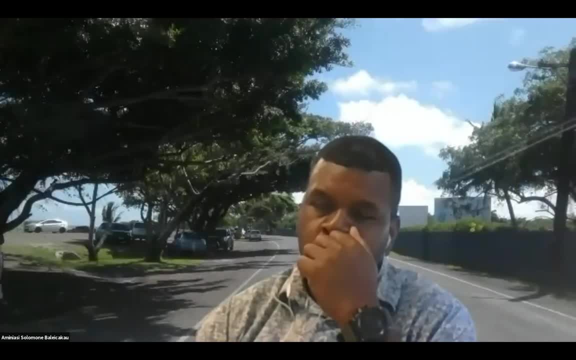 the right set of people with the experience and the qualifications experience and the qualifications, experience and the qualifications to be a part of that process. so it's not to be a part of that process. so it's not to be a part of that process. so it's not just when you have to review an eia. 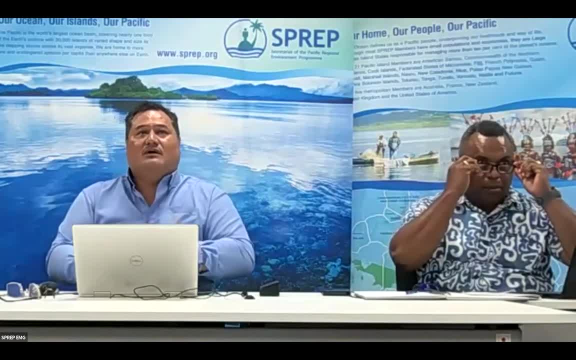 just when you have to review an eia, just when you have to review an eia report, that you need to bring folks in report, that you need to bring folks in report, that you need to bring folks in to review the actual report. but there is to review the actual report, but there is. 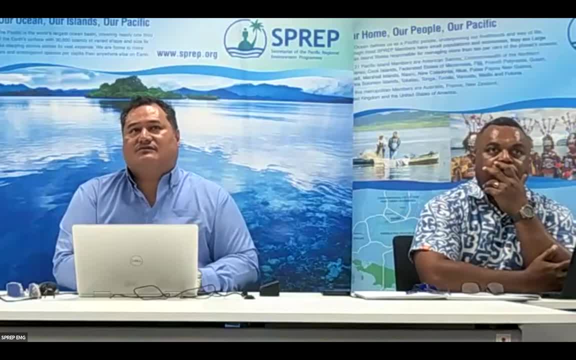 to review the actual report, but there is also merit to suggest that when you're also merit to suggest that, when you're also merit to suggest that when you're preparing a terms of reference, you also preparing a terms of reference, you also preparing a terms of reference, you also need. 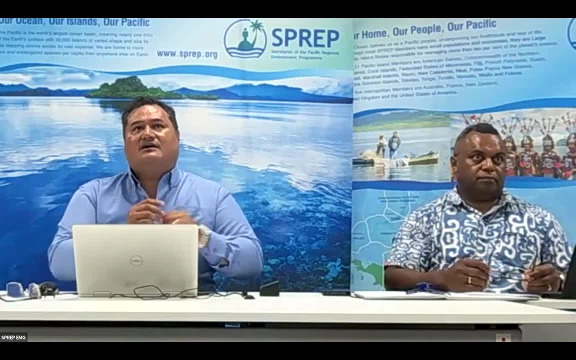 need. need uh the right set of uh expertise to be uh the right set of uh expertise to be uh the right set of uh expertise to be there to provide their conditions and there to provide their conditions and there to provide their conditions and input into the terms of reference. so 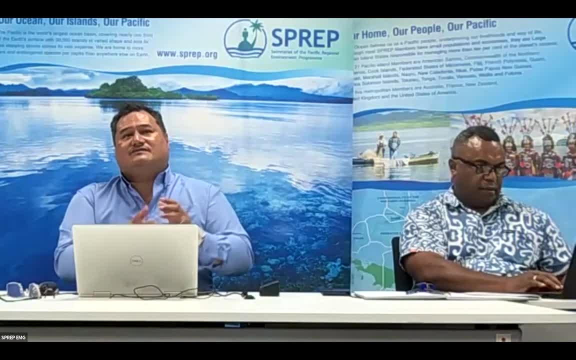 input into the terms of reference. so input into the terms of reference, so that's that's also a um, and once you've that's, that's also a um. and once you've that's that's also a um. and once you've done that, then it's easy to, then it's. 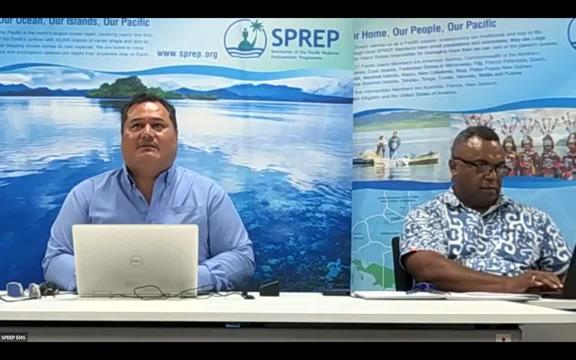 done that, then it's easy to. then it's done that, then it's easy to, then it's not it. then it's it flows- uh, rightly, not it? then it's it flows- uh, rightly, not it. then it's it flows, uh, rightly, from from that point, so that you've 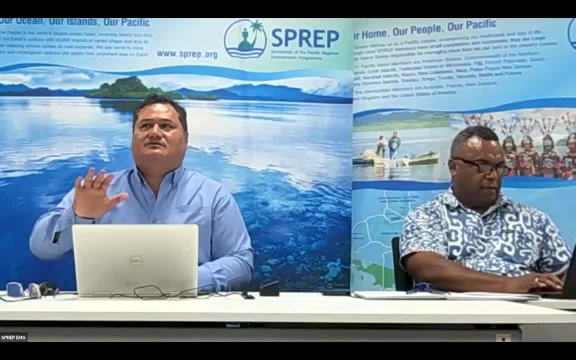 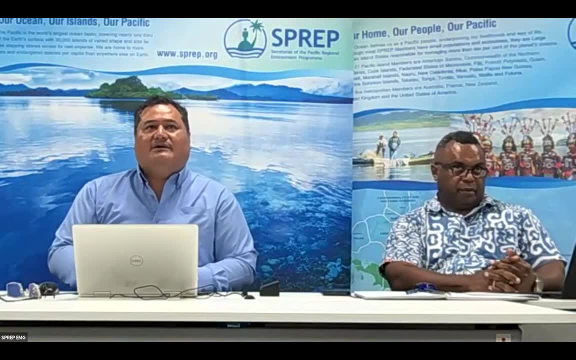 from from that point so that you've from from that point so that you've covered everything. and, as regulators, we covered everything. and, as regulators, we covered everything. and, as regulators, we have to exercise due diligence and ethical practices to ensure that, uh, when we ask a developer, when to, to adhere to a specific terms of 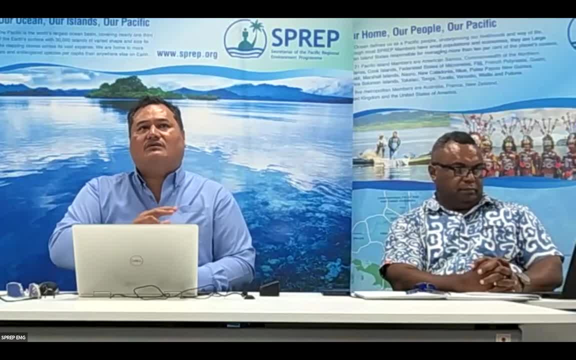 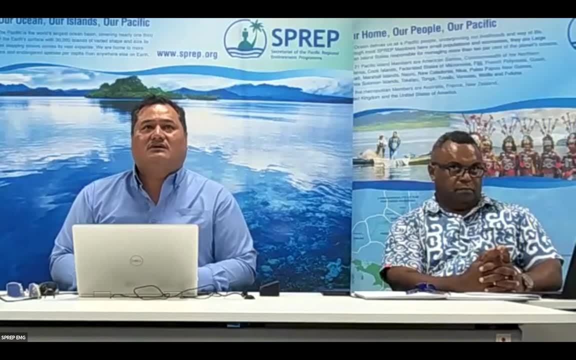 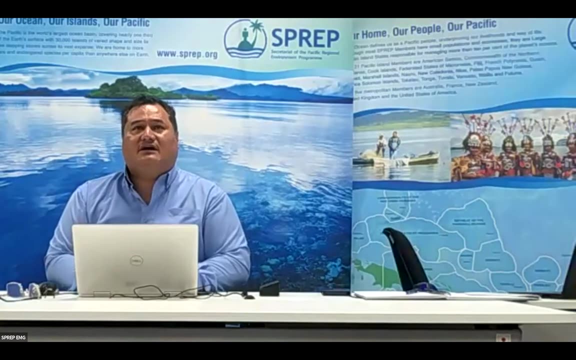 reference. what you're doing is you're covering all a broad range of issues that the government is mandated to regulate as part of their, as part of their role, and- and also inherent in that is your. also, there's a responsibility that we brought on to the developers themselves so that we do not 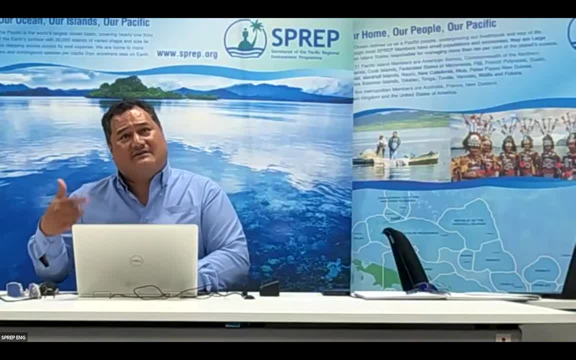 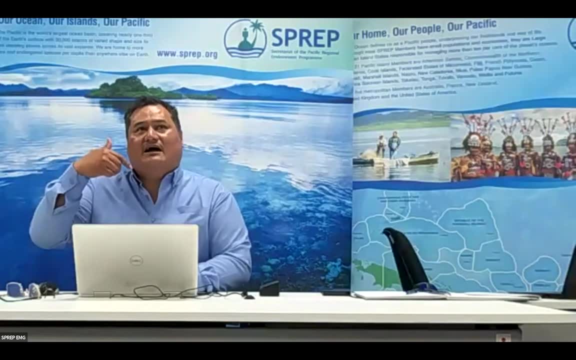 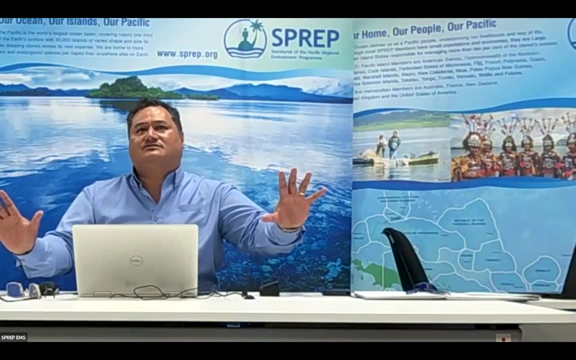 have too much come back and forth, because every time you do that, because you do not design the terms of terms of reference properly, a developer has to uh uh, incur costs because that's something that wasn't discovered, and so once you have a proper team to do to develop in terms of reference, 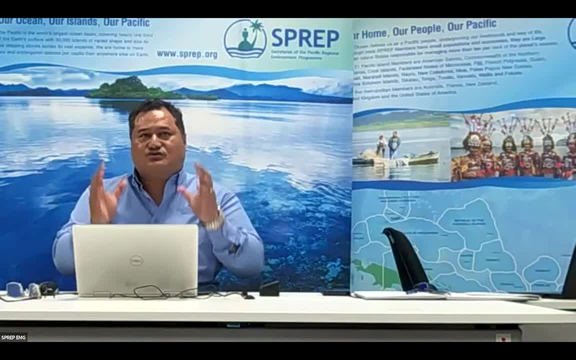 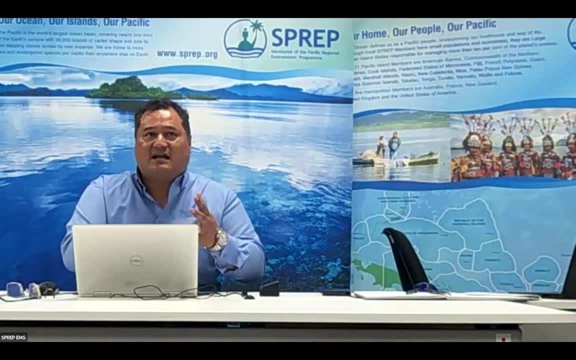 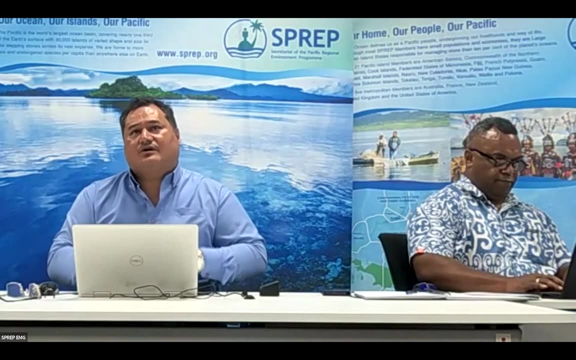 you know, i mean you're not going to cover everything under the sun, obviously, but you should know the key areas that a particular proposal, the key areas in environment, the key society, the key areas that would be, you know, affected by by a particular proposal. so i think 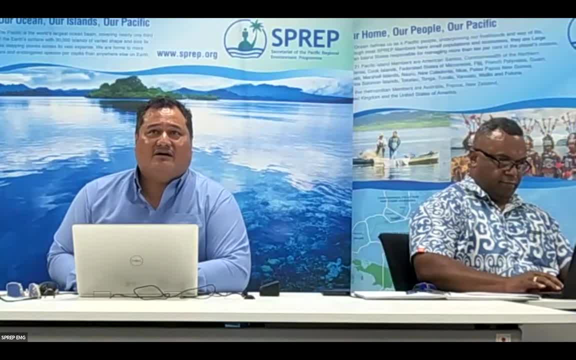 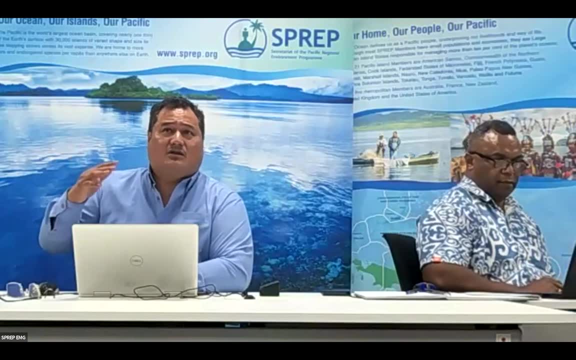 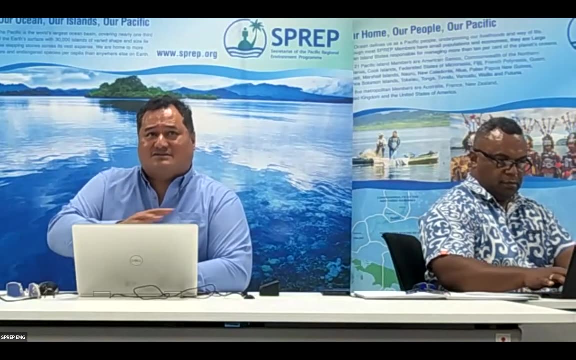 this is uh, and i think this is why many of you have uh requested to to for this, for this training uh to to occur. we did, we did touch a lot on on scoping in the first round last year, um, and so i think, uh, you know, there is still merit to continue that conversation today. now let me go. 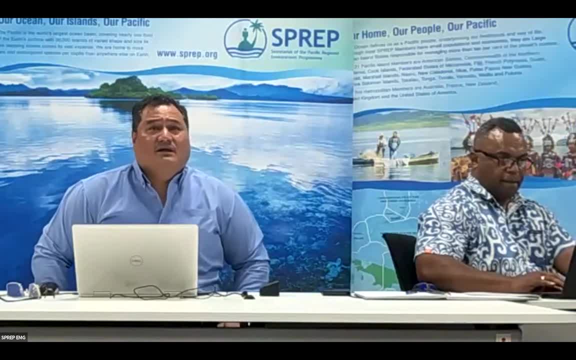 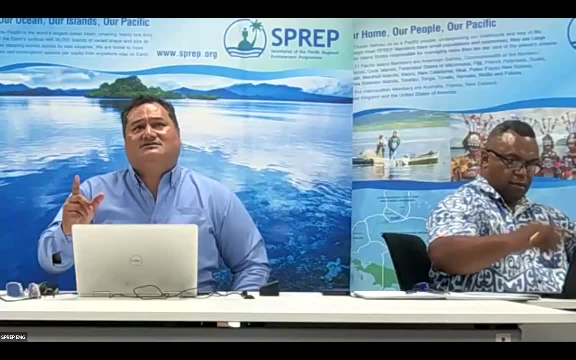 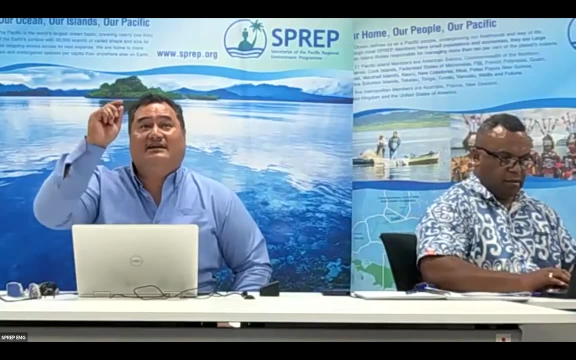 back and ask: is: is, uh, the barbara on board or if the? if that's not the case, i'd like to suggest if we could have all the cameras. yesterday, we did not take a photo, and that's the beautiful thing about zoom is we can actually have all of your beautiful faces online and then we can take a photo, because after this, 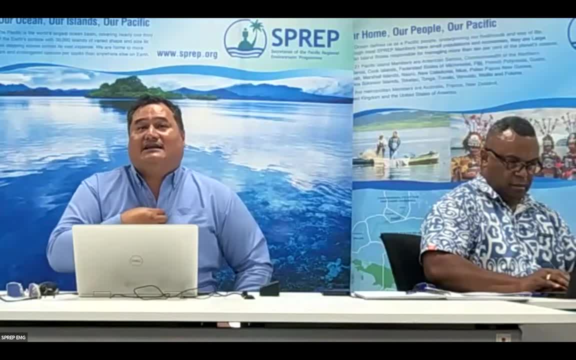 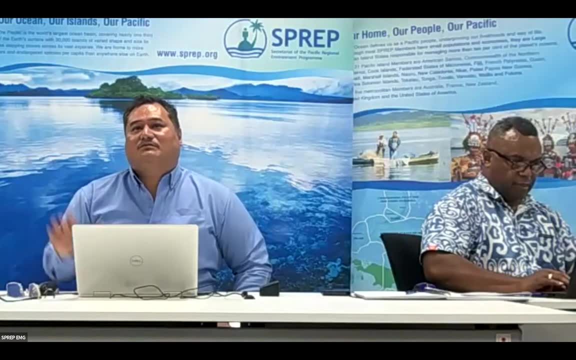 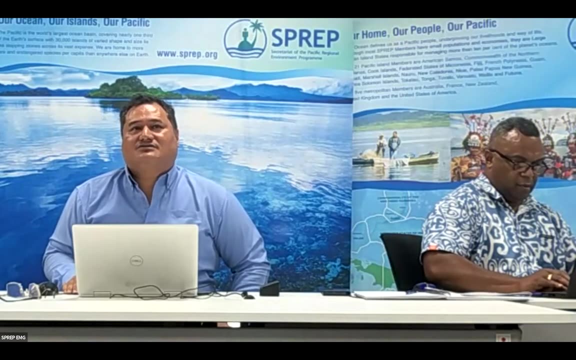 then we have a press release and, uh, like me, i need to have evidence that i'm here, so it'd be great to have a photo, or have a photo. so please do turn on your, turn on your cameras and we'll get ivan, and hopefully that's enough time, uh, for us to. 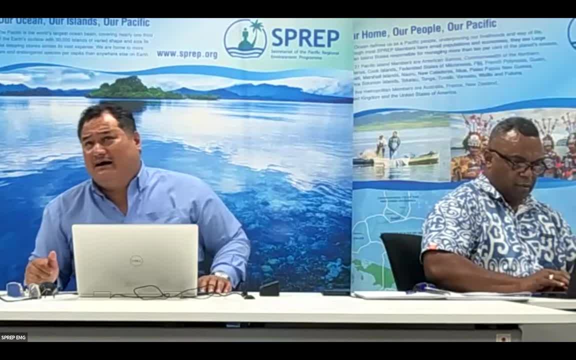 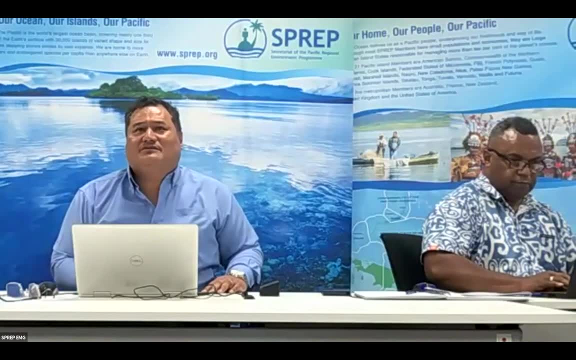 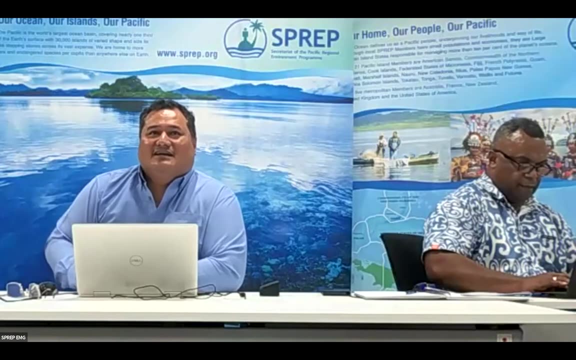 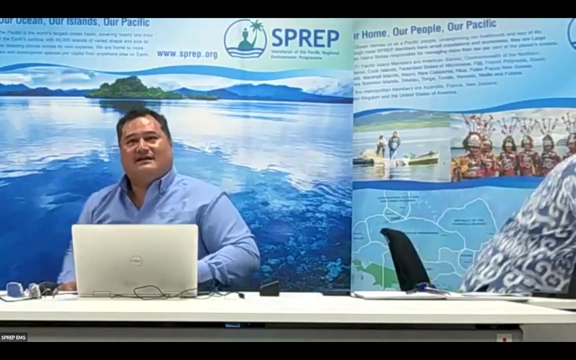 regroup. um, yeah, so please. we've got about 53 participants, so i'm expecting 53 picked um videos to be turned on, if you don't mind. oh great, uh, just um. ivan, would you like to take a photo? should you stand? stand there and um, wait, you want to photo the camera? 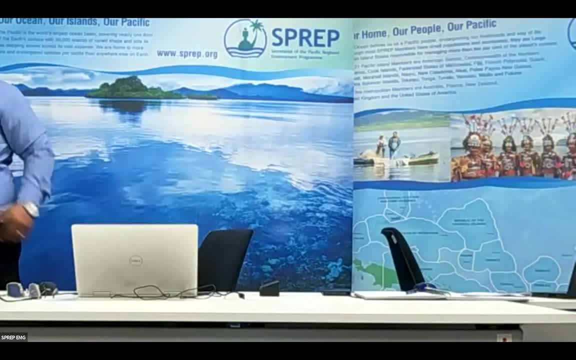 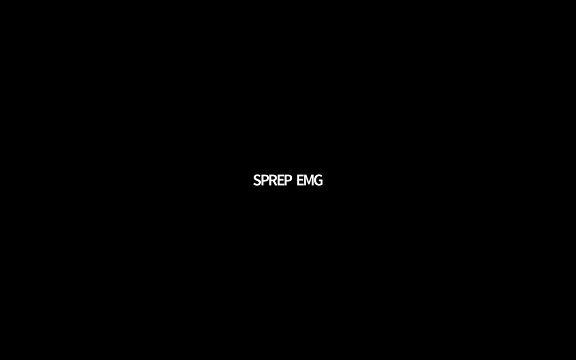 yeah, yeah, the camera. so do we just stand right next to the yeah, yes, yeah, we'll just stand right next to the yes, yes, all right, let's do that. yes, so, so all right. so Is it? you know? just okay, I'll give, I'll give Joppa five minutes, but one more, one more, one more activity to fill in the gap. 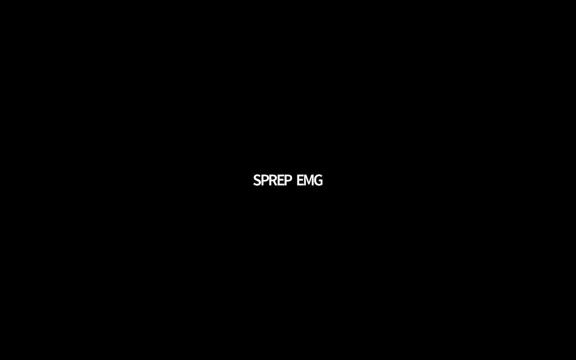 Can I? I'll name the country and please link and please put on your, your microphone to say you know, and say that you're from that, from that country. I want to see where we, where you're, you're joining it from. 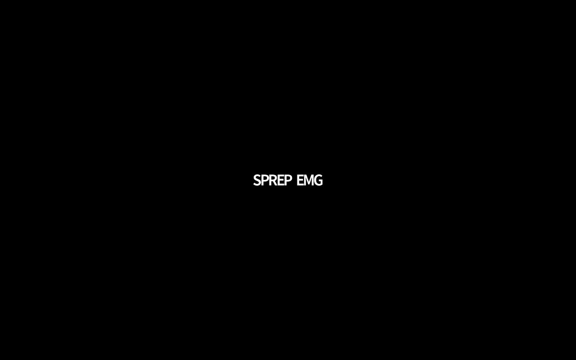 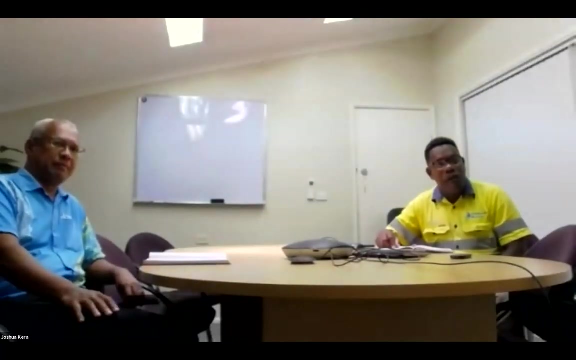 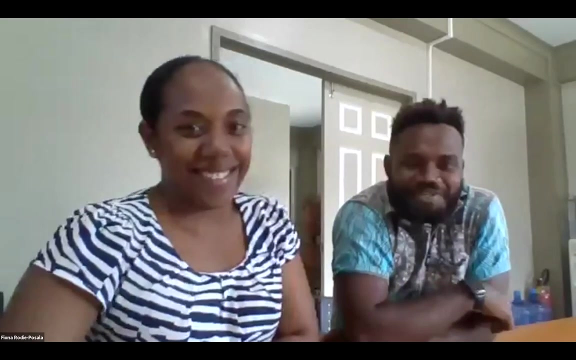 Very quickly. Papua New Guinea: All right, We've got Papua New Guinea present. How about Solomon Islands? Samoa: Bula spread, Bula bula. Okay, Fiji, Jump in Fiji, Fiji, Fiji Bula. 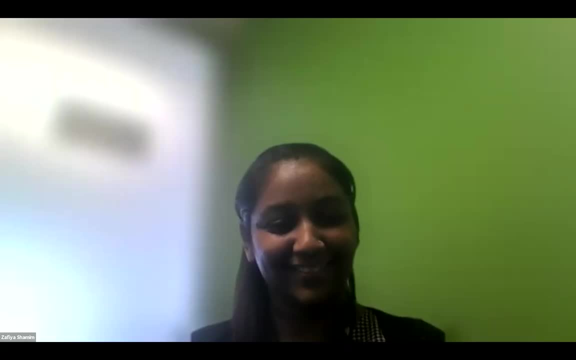 Bula, Bula, Bula, Bula, Bula Bula, All right, Okay. Well, it looks like everybody from the region is here, so that's great. All right, Let's move. Let's get on with the show. 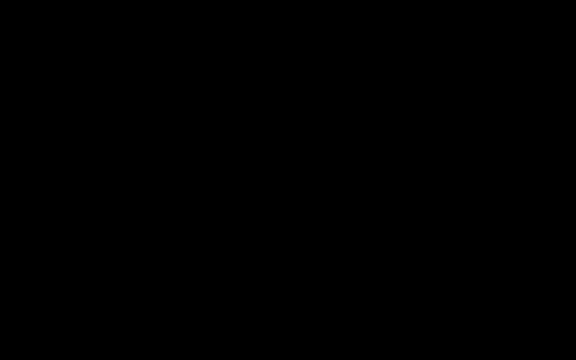 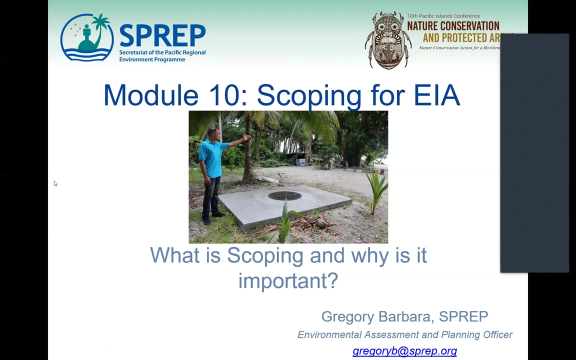 So Joppa will step in at the moment while we have Greg trying to link in, and we'll continue on. Thanks for your patience and my apologies for the technical glitches. These things happen, but the show must go on, All right. 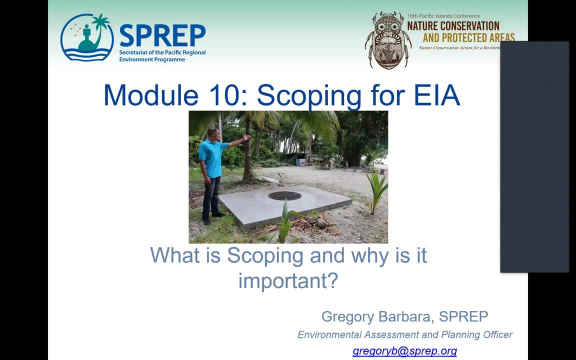 Thank you very much, Mr Moderator, and thank you, Rachel, for your earlier remarks on setting the scene for this particular module. And colleagues, I will be stepping in for Dr Barbara this morning And, yes, my name is Joppa and I'm currently managing the Environment Monitoring Governance. 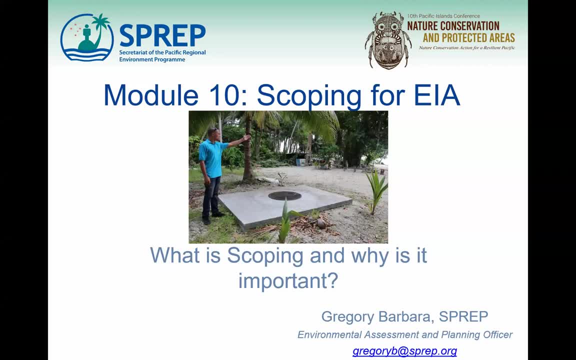 Program And it is so good to see lots of familiar faces. And please, colleagues, we are all in this together and please jump in to contribute to this important item, to share your experience and your know-how on how we can improve scoping. 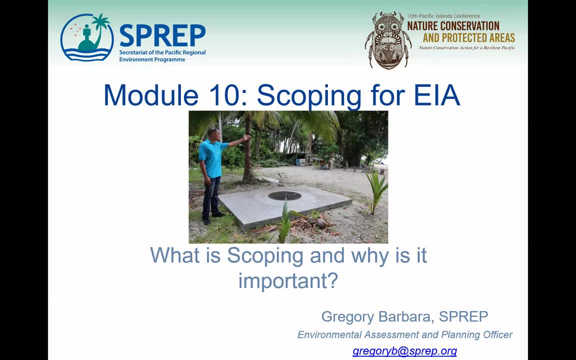 in the area of environment impact assessment And it is module 10.. And may please bear with me, and I'll be going through this slide that was prepared by Greg And jump in. as I said, jump in to contribute to the discussion. 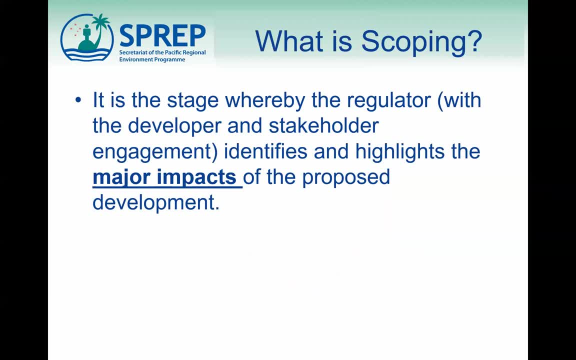 And the question that Greg started off with is: what is scoping? What is scoping, And as it reads, as it reads, it is the stage whereby the regulator identifies and highlights the major impacts of the proposed development. Okay, Okay. 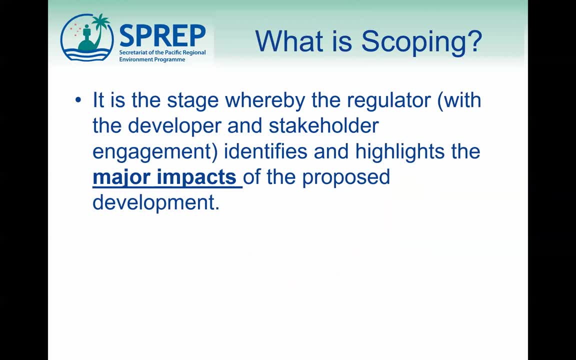 Okay, Okay, While working here in the Pacific region, we tend to observe, we tend to observe that there are some countries that are very good in setting up their governance system, including to include scoping as an important step, as an important step of the whole EIA process. 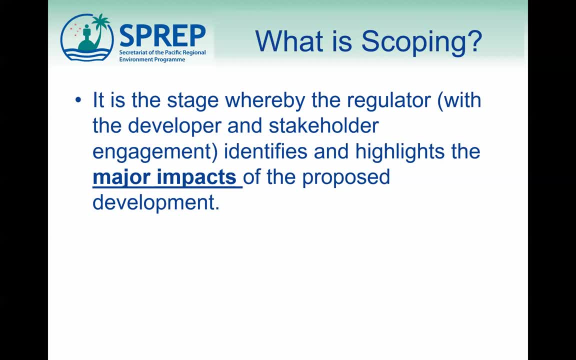 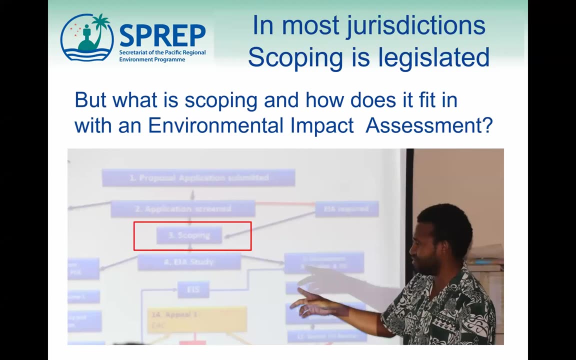 But for some they are getting there. They're getting there And please, in my understanding of the In the general process of EIA, this is an important step for the whole EIA process. In most jurisdictions scoping is legislated. 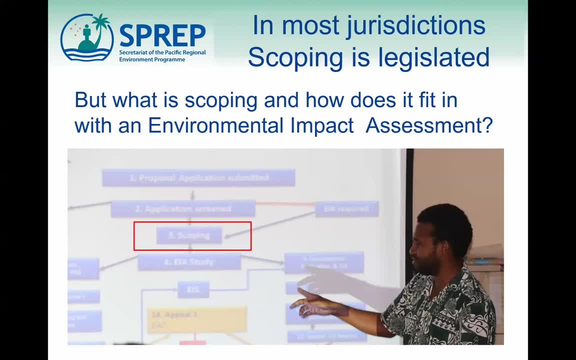 Yes, I talked about that earlier on. And when the application is screened, after the application is screened and it is scoped, it is scoped, And here on this slide we have our colleague from the Solomon Island in one of our EIA. 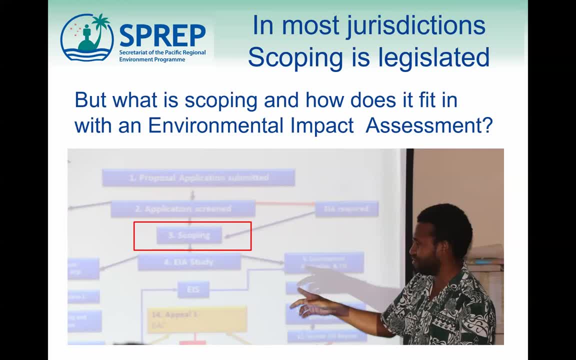 training And this is, if I'm correct, this is part of the EIA training for them to understand the approval process between the regulated EIA process and other approval agencies, such as mining and forestry In particular training. it is focused on mining. 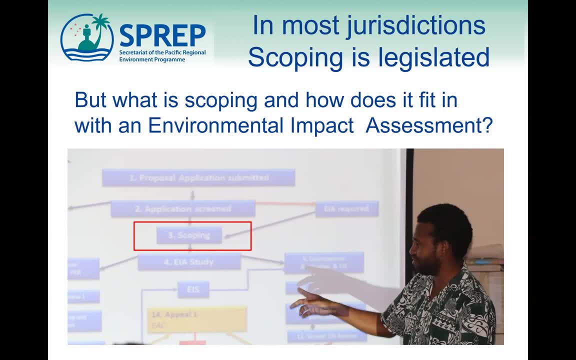 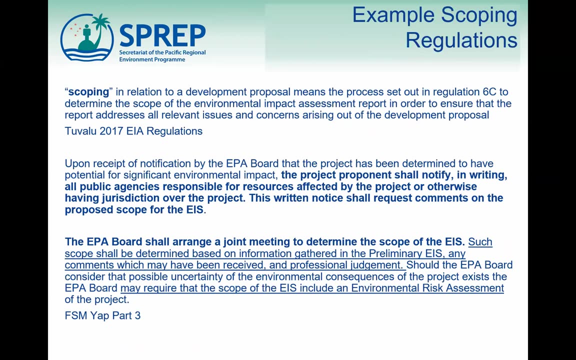 So, yes, when we talk about the scoping in the EIA process, it comes into play After the project has been screened. Example scoping regulations: Yes, under the 2017 EIA regulation, it clearly stated that the need to undertake a scoping 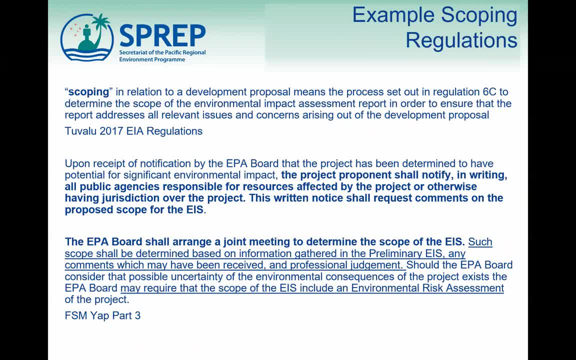 And not only in Tuvalu. Not only in Tuvalu, We have the FSM, part three of the regulation, And also in my experience working in Fiji and also while working with the planning and urban management agency of Samoa, they are considering and looking at scoping as an important. 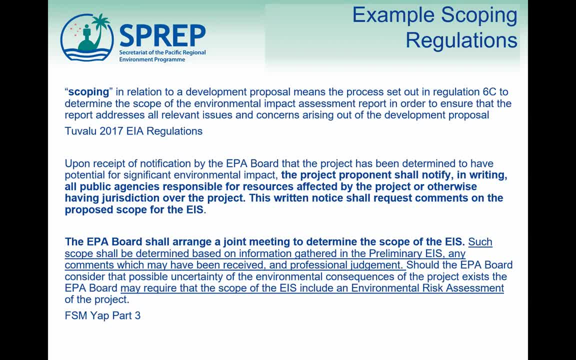 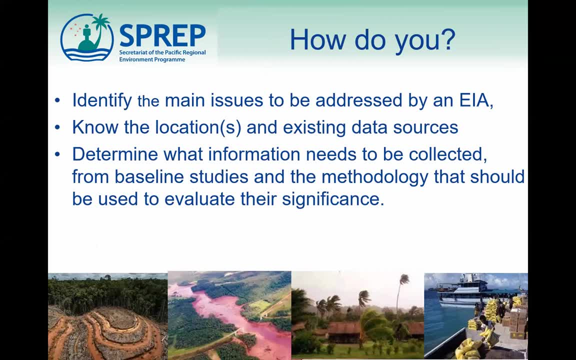 important, important step of the EIA process. So how do you carry out scoping? Why is scoping is important? It is mainly to identify. The main issue is to be addressed by an EIA And exactly to know the locations and existing data sources. 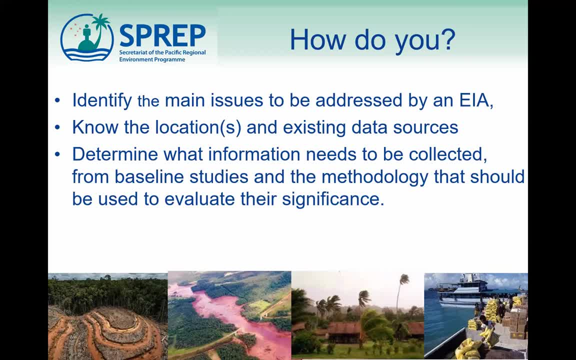 This was discussed at length and there were lots of interest in GIS yesterday, So there was a mention of this particular process, even using GIS- GIS 2- as part of the scoping And it also to determine what information needs to be used. 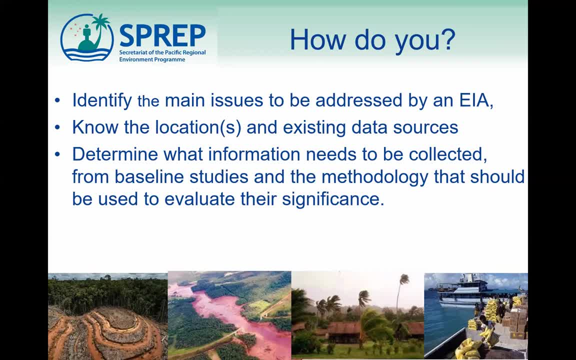 What information needs to be used- needs to be collected from baseline studies and the methodology that should be used to evaluate their significance. And colleagues, again sharing my experience on scoping in my term as an EI regulator, sometimes for environment agencies. they are always worried about them taking the task. 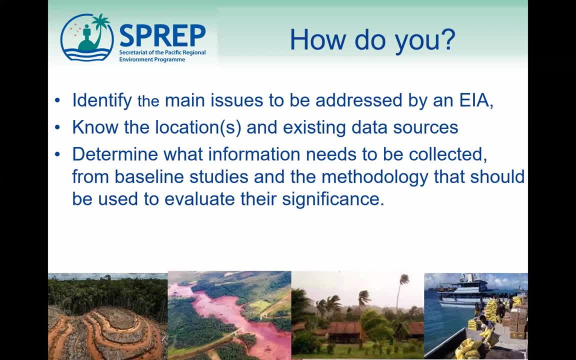 alone. But no, that should not be the case When we are doing scoping- and again this point was raised yesterday- it should be a collective commitment, collective contribution, not only of the environment agency, but other sectors, other sectors such as other regulatory agencies, such as mining, forestry, water. 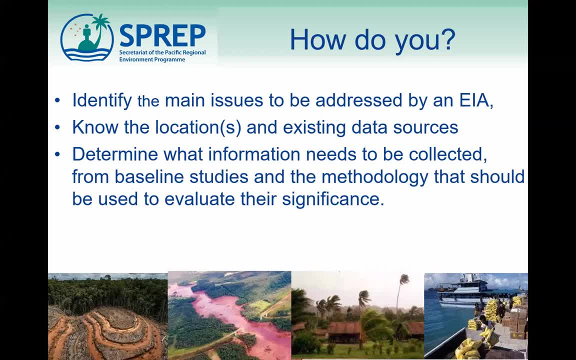 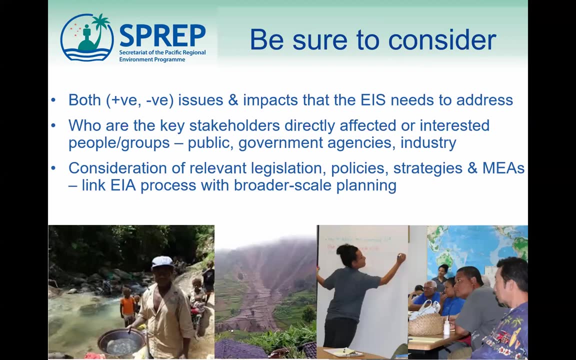 transport, and even colleagues, consultants and developers in some countries. they are all included in the scoping exercise And while undertaking scoping, colleagues, while undertaking scoping, be sure, be sure to consider both positive and negative issues and impacts that the EIS needs to address. 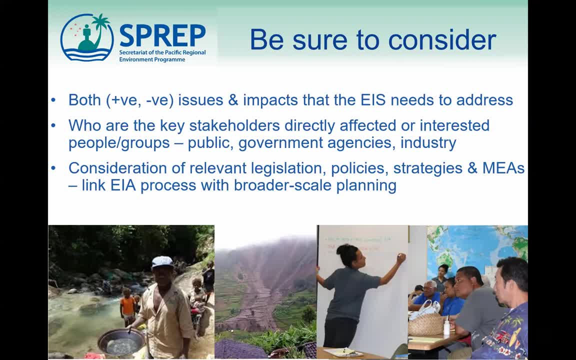 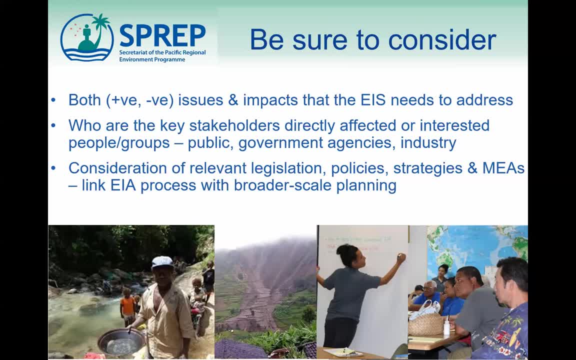 reference when it comes to addressing the content of the EIS. there is no boundary to govern their work in the area of review of that particular EIS report. So it is vital. it is vital why scoping is important, why they divide. 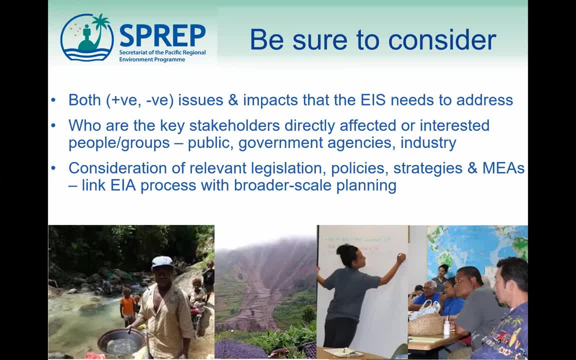 So it is vital. it is vital why scoping is important, why they divide Positive and negative issues. Second bullet point: Who other key stakeholders directly affected or interested people groups, public government agencies, industries? Very, very important, colleagues, very, very important. 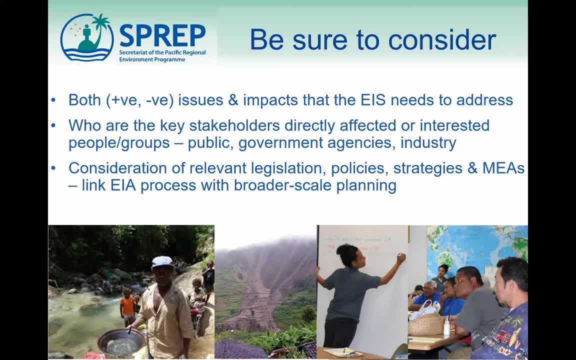 We, as environment or regulatory agency responsible for a particular development, or if you represent the department or an environment agency regulating the EIS process, it is important, important that you consult with the key stakeholders so that they will be involved in the initial stage when this project is screened and scoped, because come a time when the terms of reference 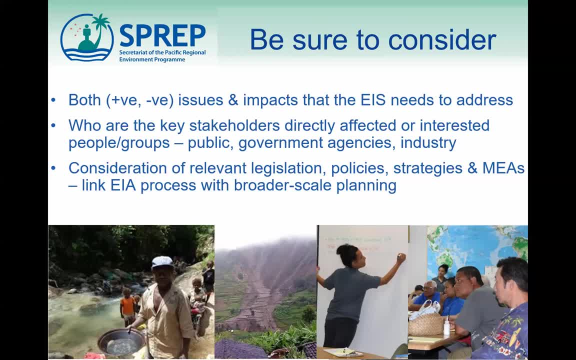 is developed. they will also need to input their opinion and their comments in the terms of reference because at a later stage they will need to review the EIA report. Bullet point number three: consideration of relevant legislation, policies, strategies and multilateral agreements and link to the EIA process with broader scale planning. 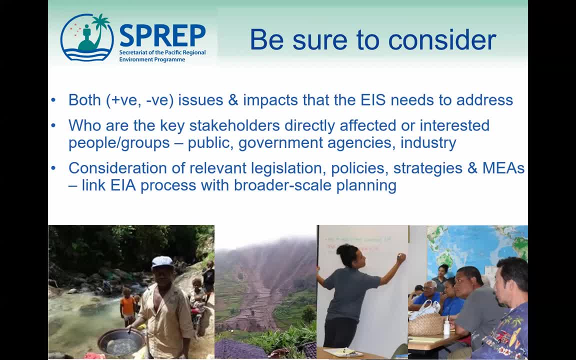 Colleagues and representatives of the various agencies and countries. this is very, very important. When undertaking scoping, we must consider existing relevant legislation. Yesterday there was a good scenario shared yesterday About gravel extraction. when we talk about gravel extraction in Fiji, we talk about the 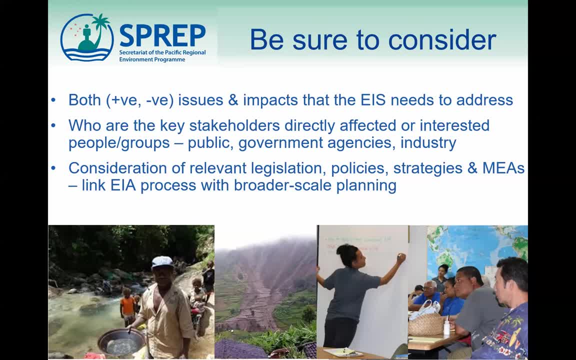 EIA regulatory agency. we talk about the lands department, we talk about the minerals department, we talk about the forestry department. So it is very, very important that all these sectors have their own mandate in enforcing the legislation within these environments. So that is very, very important, colleagues, that consideration must be applied to these. 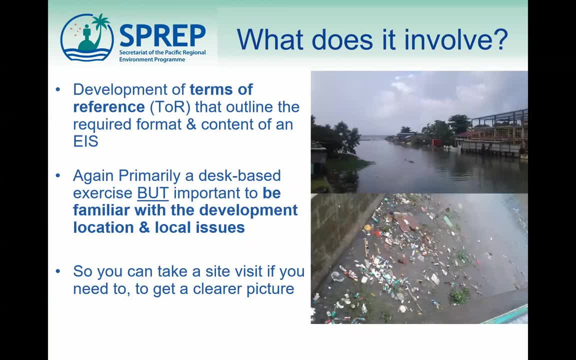 relevant legislation. Thank you. So what does it involve, colleagues? What does it involve? Development of terms of reference that outline the required format and content of an EIS. It's been observed that for some member countries, it is part of the regulation that it has a 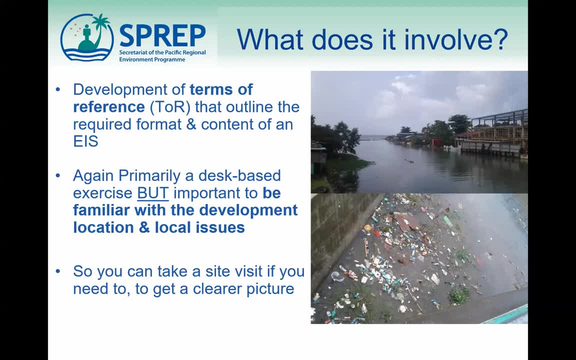 role to represent the timeline, the required format or content of an EIS. Some have referred to it as that is the terms of reference. Yes, to some extent. yes, But we need more detailed information that needs to be included in their framework or. 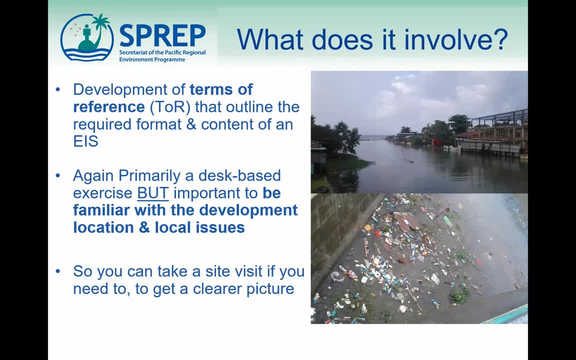 outline so that it reveals the impact of that development on that particular location. Again, primarily a desk-based exercise, but not for all countries. Is there any question about the EIA? Is there any discussion side? but important to be familiar with the development location and local issues. 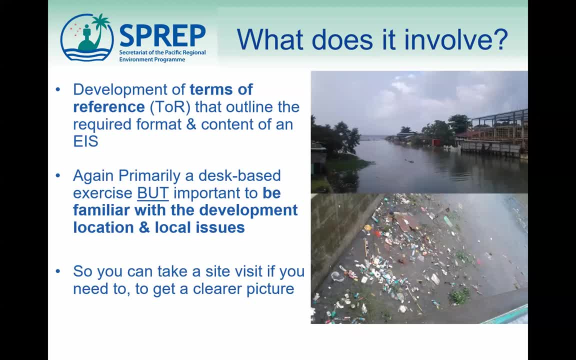 Colleagues again allow me to further discuss this particular bullet point. And when receiving a particular application, it is very, very important for EIA regulatory managers to mobilize their team in understanding the location, the development shelf and also the location. 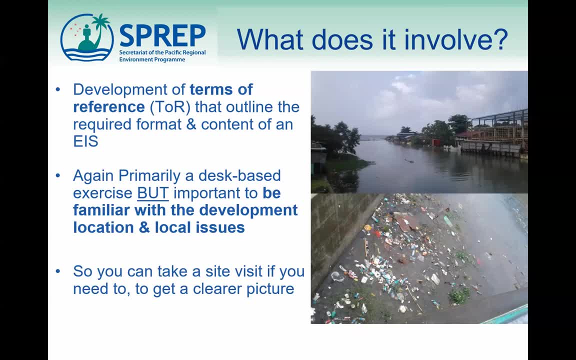 That is why critical system thinking must be applied And even, at some stage, you can do your own internal analysis to see what are the positive impacts, what are the negative impacts, before you go and do validation on the ground. And yes, colleagues, again, this point was shared by our GIS ladies yesterday: the importance. 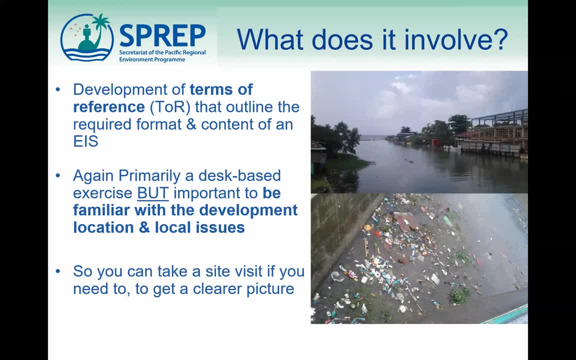 of being familiar with development location. There was a good scenario too, shared yesterday, where the Forestry Department has a clear map outline of the Ramsar site in Fiji, where it triggered the decision to relook at adjusting the boundary by the developer. 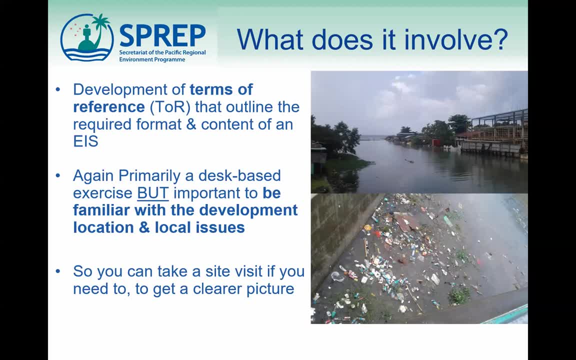 So, colleagues, on bullet point number three, so you can take a visit, site visit if you need to to get a clearer picture. Thank you, May I again elaborate more on this? Colleagues, for some countries in the Pacific region, when they talk about scoping, they 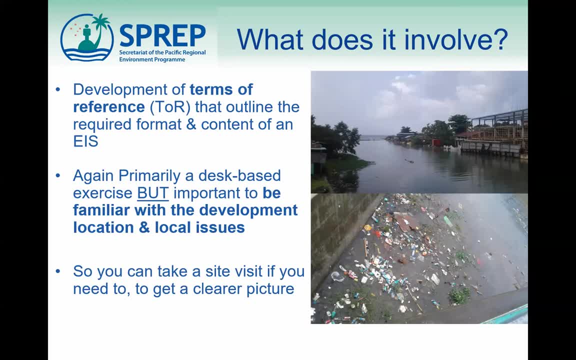 have provisions. They have provisions that allows the developer to support the agencies in taking site visits so that a clear terms of reference and understanding and validation of what's written in the application is there on the ground. Critical thinking- what is this? Critical thinking: what is this? 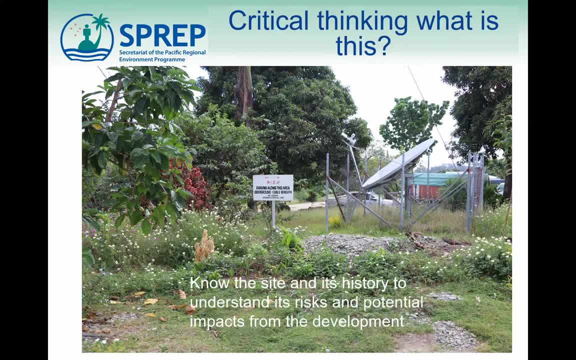 So know the site and its history to understand its risk and potential impacts from the development. Very, very important Again, when working as a team for regulatory agency, please may we kindly advise that you are not working there alone. There are agencies involved. 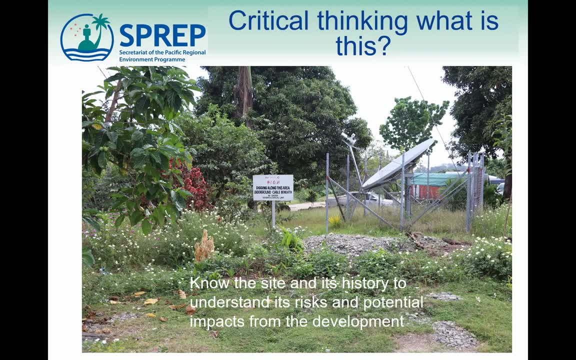 Thank you. They are there to support you in understanding and knowing the location in which a particular proposal is planned to be made. And thank you to the ladies yesterday about addressing the importance of scoping within the various scenarios. they presented Key issues with doing it right. 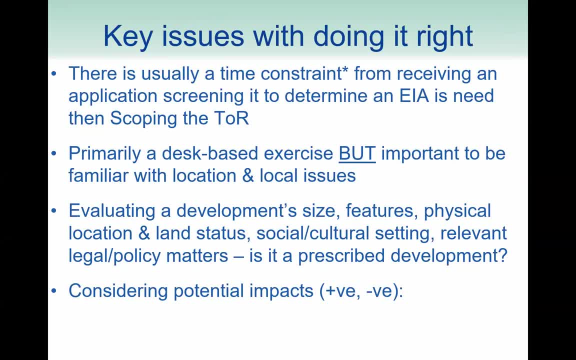 Key issues with doing it right. There is usually at time constrained from receiving an application. screening to determine an EIA is needed. then scoping the TOR: Primarily a desk-based exercise, but important to be familiar with the location and local issues. Evaluating the development size features. 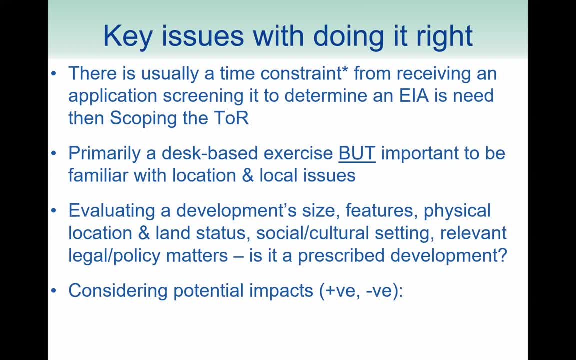 fiscal, location and land status, social and cultural settings, relevant legal policies. is it a prescribed development, Considering potential impacts, positive and negative? Colleagues, if I may share my experience while working as an EIA regulator, in some instances 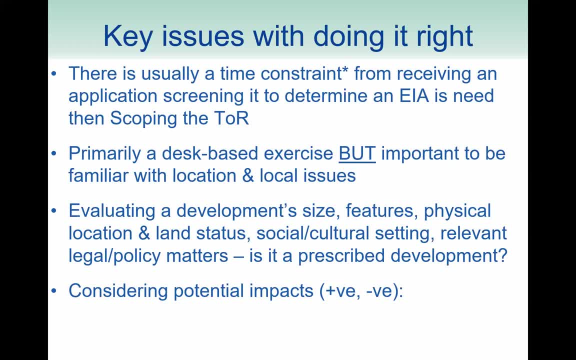 in my experience, some concepts are redesigned because of the importance of this particular step of the process called scoping, And also some developments are changed. The location of that particular development are re-looked at finding other alternatives when scoping is properly carried out. 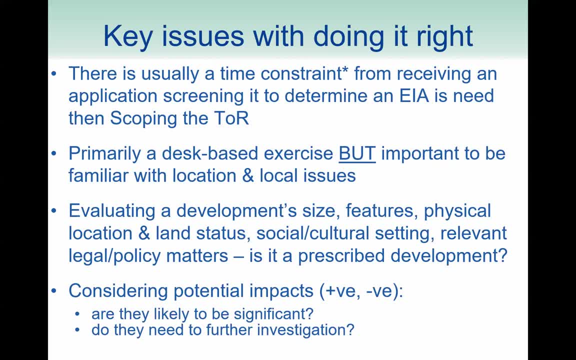 Considering the potential impacts. are they likely to be significant? Do they need further investigation? So these are the questions. These are the questions that needed to be asked by the team when they are developing the content Of the terms of reference in this particular step called scoping. 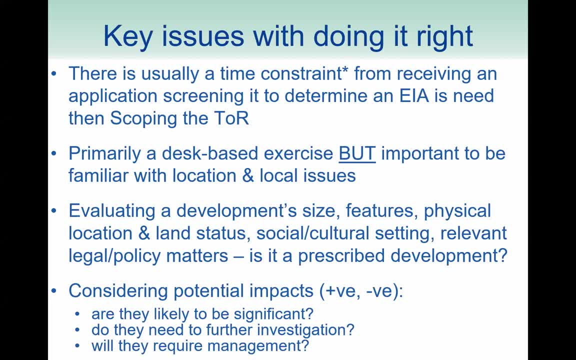 Will they require management? Yes, Very, very important colleagues, One of the items that was observed or we found out from our participants in the last meeting, and also it's raised in our discussion while planning through these training modules, is the importance of management: Management of a particular 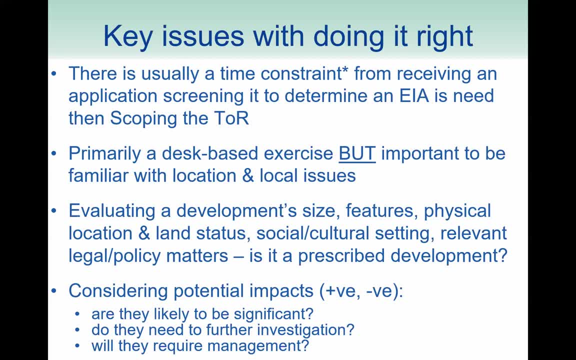 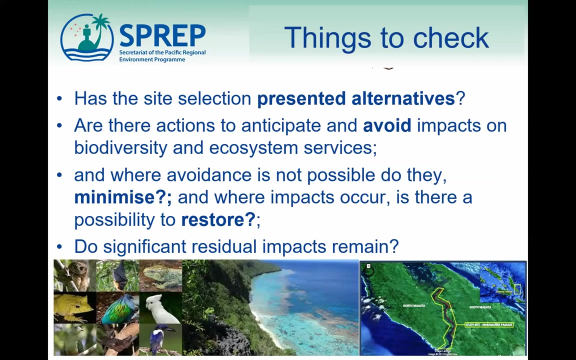 particular development With this specifically I flagged this time is the importance of understanding and designing proper construction and operational environment management plans. Things to check. Things to check, colleagues, As the site selection presented alternatives. yeah, I talked about this. I talked about this And this was also came up in the discussion yesterday. 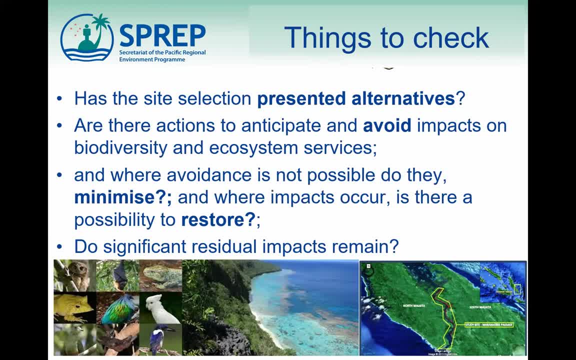 on the GIS presentation. Are there excellence to anticipate and avoid impacts on biodiversity and Ecosystem services? Yes, very, very important. And where avoidance is not possible, do they minimise? And where impacts occur, Is there a possibility to restore to significant residual impacts that remain? 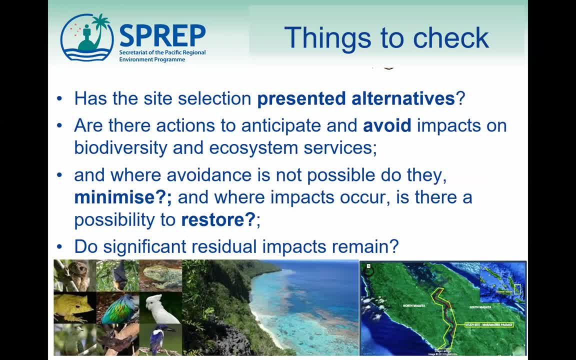 I think for this one, for this one, a good example again I would like to reflect on, on the REMSCG site in Fiji, where it crossed the boundary and the decision is: they must walk according to what the legal boundary of the Ramsa site. 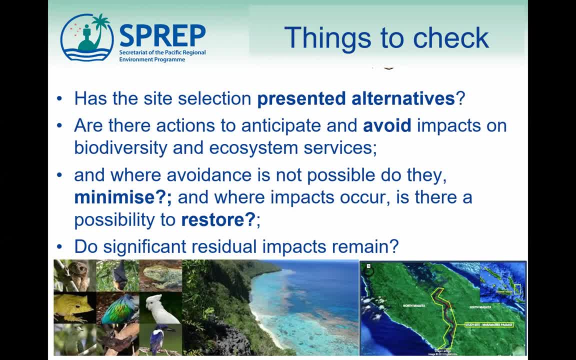 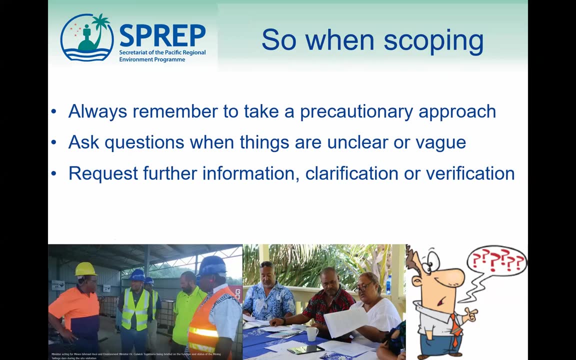 So for that one they have to avoid reaching or moving into the Ramsa site. So when scoping, colleagues always remember to take a precautionary approach. Ask questions when things are unclear or vague. Request for information, clarification or verification. 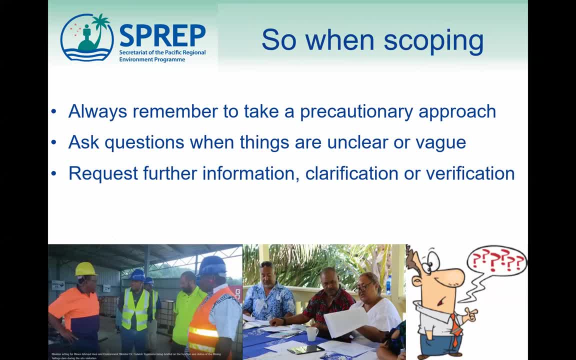 Very, very important colleagues, Very, very important. Sometimes, when a scoping is completed, a scoping field visit or field visit is completed, we can always have time to revisit again what we saw and create some discussions on what is really necessary to be found out in. 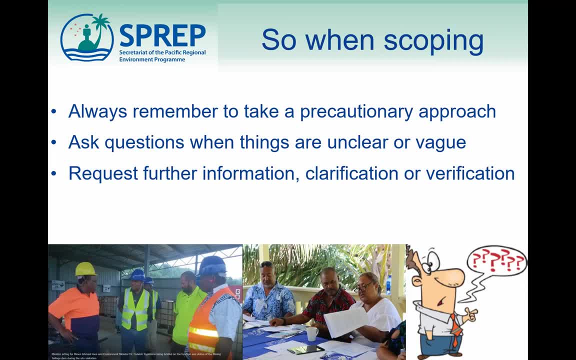 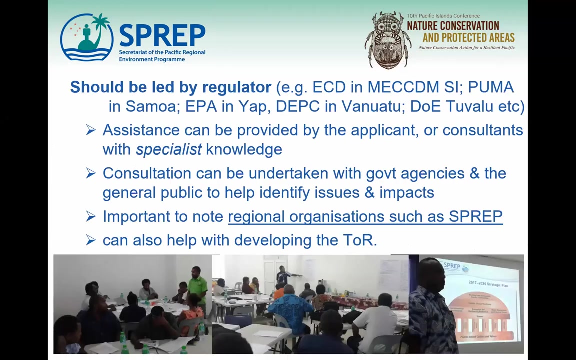 the EIA study that has to be undertaken by the developer or the EIA consultant. Then focus the TOR. Once this discussion is clear, then your TOR or EIA Terms of Reference will be clear. Should be led by regulator. Example: Environment Conservation Division in the Solomon Islands, in Samoa. 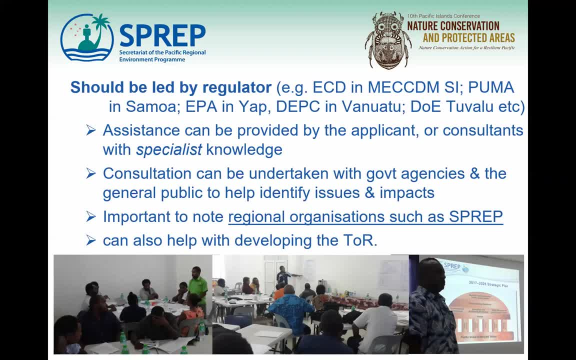 the EPA in IAP, the EPC in Vanuatu, DOE in Tuvalu, etc. But, colleagues, it's very interesting that you know for some of our member countries they do scoping, but the idea of developing a clear Terms of Reference is something. 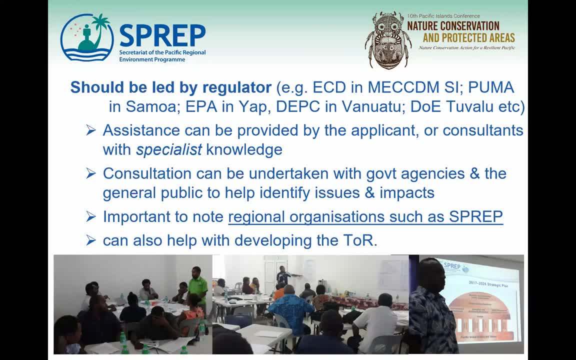 that needs to be added in into their policy or existing regulation, But there is an excellent work done by all these environment agencies in undertaking This particular step of the EIA process. Assistance can be provided by the applicant or consultants with specialist knowledge And for some of our member countries. thank you to you for always using SPREP. 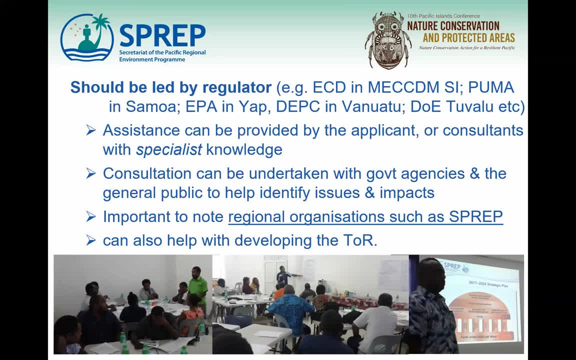 in providing support to your respective environment agencies in developing or providing assistance or contribution to Terms of Reference, And the EIA has a list of reference of some particular developments that they are interested in or they are screening. Consultation can be undertaken with government agencies and general public to help identify issues and impact. 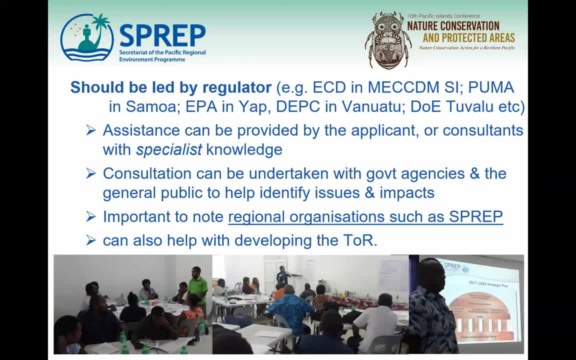 Colleagues, very, very important. Sometimes in the EIA process there is a separate step which is called public consultation or, yes, community consultation. But in the scoping step alone, colleagues, yes, public consultation is an important activity to be undertaken. 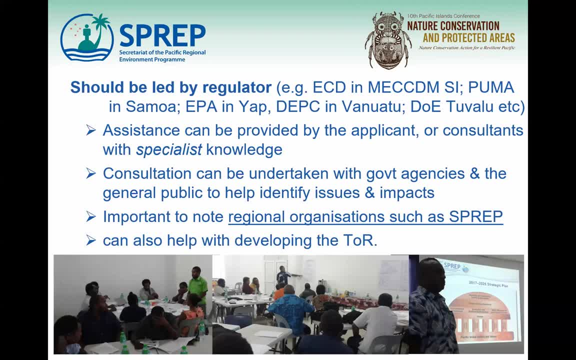 Because there are lots of knowledge and observations that are done by, that are known by the public, that we need to know as regulators. Important to note: regional organisations such as SPREP can also help with the development of the Terms of Reference. May I also add in this juncture that 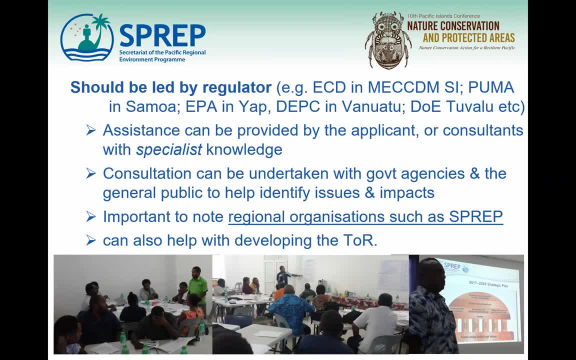 in some countries they have provisions in their regulation identifying the various corporate agencies and institutions that can help them in this particular step or this particular process called scoping. That is only to do with development of Terms of Reference. Importance of Terms of Reference. 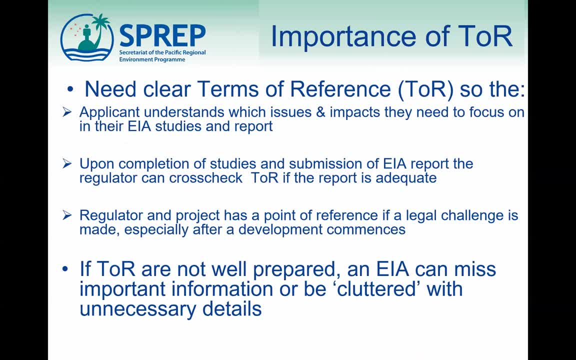 We need a clear Terms of Reference So that applicant understand which issues and impacts they need to focus on in the EIA studies and report. Very, very important, colleagues, Very, very important: Upon completion of the studies and submission of EIA report. 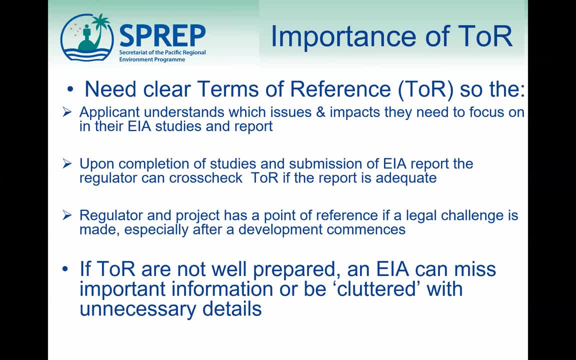 the regulator can cross-check Terms of Reference if the report is adequate. Colleagues again, in some countries there is provision in their EIA regulation that when the developer submits an EIA report, the approved Terms of Reference must be attached as an annex to that EIA report. 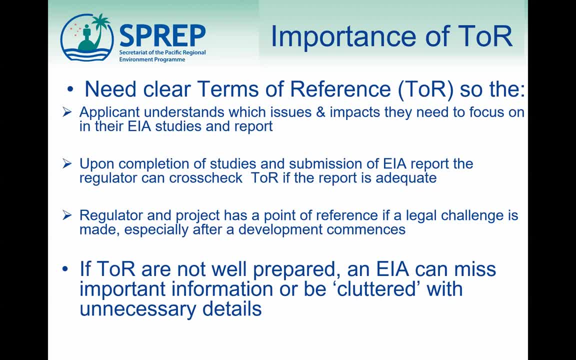 So that the regulator can cross-check the Terms of Reference with the copy they have and this will allow proper review of the report according to the Terms of Reference, approved Regulator and project has a point of reference if a legal challenge is made, especially after a development commences. 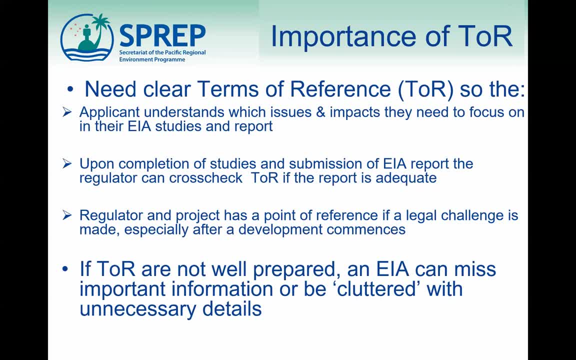 Colleagues, if a TOR are not well prepared, an EIA can miss important information or be cluttered with unnecessary details. Colleagues, while working at PrEP and working with some of our member countries, it's good that this area is developing very, very quickly. 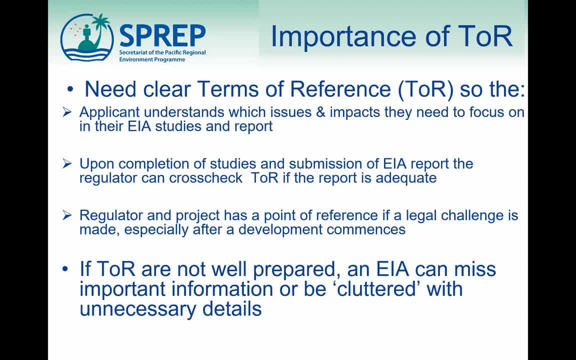 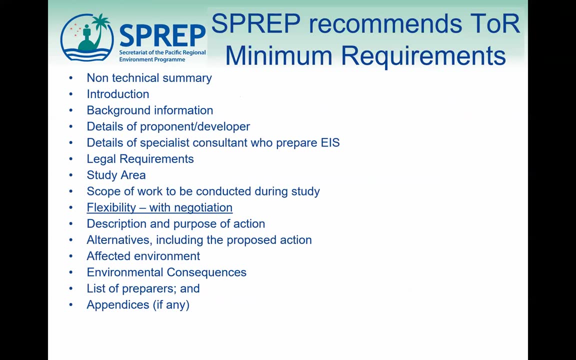 especially the area of Terms of Reference, And it's helping the countries Now in understanding the importance of this, because it will help them in getting the necessary information that is needed for a particular development. PrEP recommends secure minimum requirements. Yes, if we look into these minimum requirements, 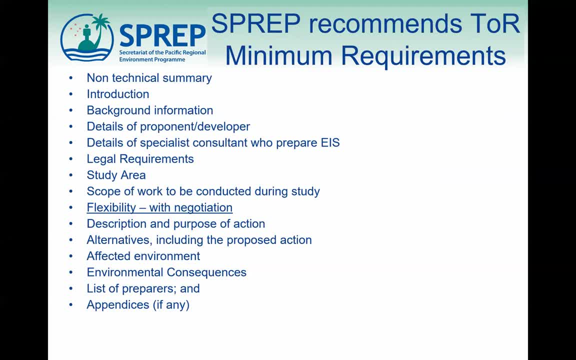 most of these are reflected in most EIA regulations In the countries And if we look through this list, non-technical summary is always an important part of an EIA report and also should be reflected as part of the Terms of Reference because, due to the technical component or content of the EIA report, 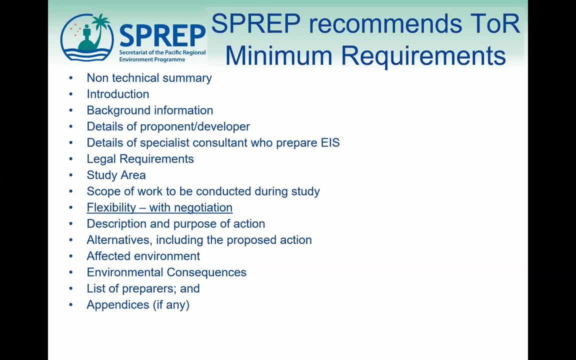 it needs to be simplified so that it is understood by the local communities. It must have an introduction, a background information, details of the proponent or developer, details of specialist consultants who prepare EIAs, legal requirements and study area. scope of work to be conducted during the study. 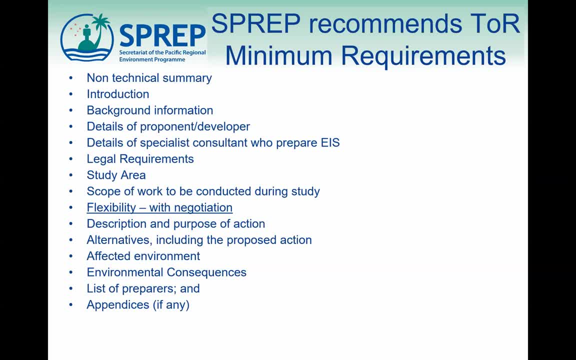 flexibility with negotiation, description and purpose of action, alternatives, including the proposed action affected environment, environmental consequences, lease of preparers and appendices, if any. So this is just a minimum requirement, As I said a while ago. there are lots of other specific details that can be included. 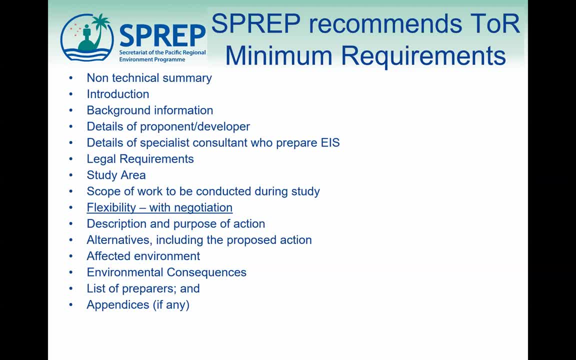 under this minimum requirement to make the report more informative and allows better decision to be made. Colleagues, the SPREP Regional Guidelines also provide a toolkit for developing a Terms of Reference. And these details, these minimum requirements, as summarized on the slide, 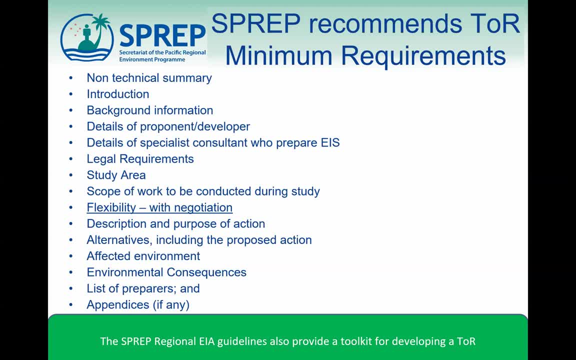 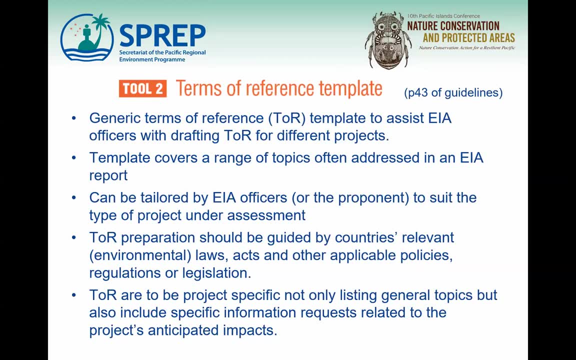 the details are contained in the SPREP Regional Guidelines as you can find in the SPREP website. Tool 2, Terms of Reference Template, page 43 of the Guidelines. It has a generic template. Terms of Reference Template to assist EIA officers. 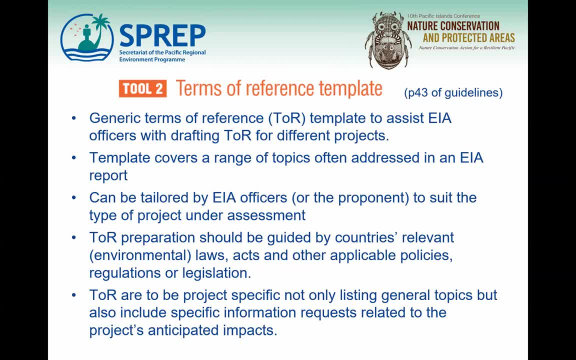 Colleagues, we've been sharing this with some of our member countries and we found it very, very useful. They found it very, very useful because it guides the member countries on what they need, what they need to understand and also what they need to observe. 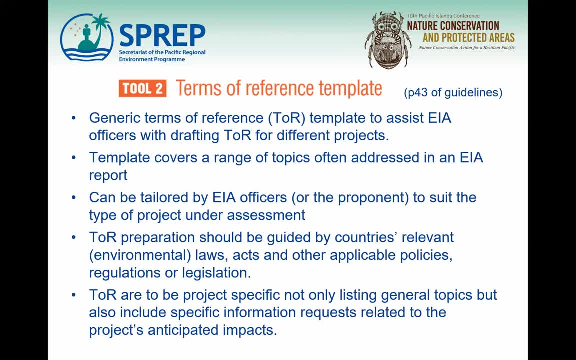 when undertaking a scoping, And your preparation should be guided by countries, laws, etc. and other applicable policies, regulations or legislations. Terms of Reference are to be project specific, Not only listing general topics but also include specific information requests related to the project, anticipated impacts. 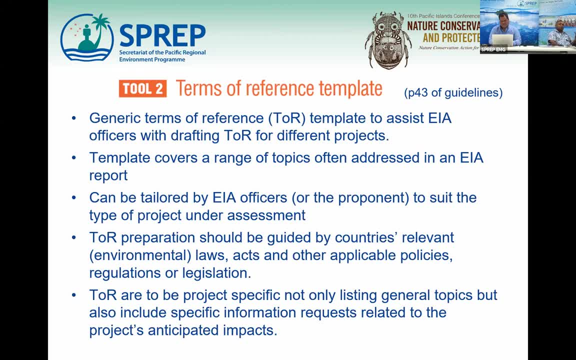 Very, very important. Yes, this is something that has been standing out in the presentation today about the specific information Colleagues. why we are emphasizing this point? because in some instances, some instances when EIA reports are fully completed, we then pick up some very, very important information. 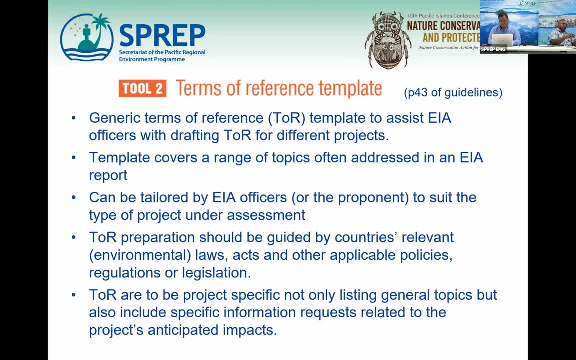 or issue or error that needs to be provided in the report to assist in the decision making. So that is why, colleagues, when you look at the whole process of scoping, the importance of engaging a wider stakeholder, important stakeholder in this process, 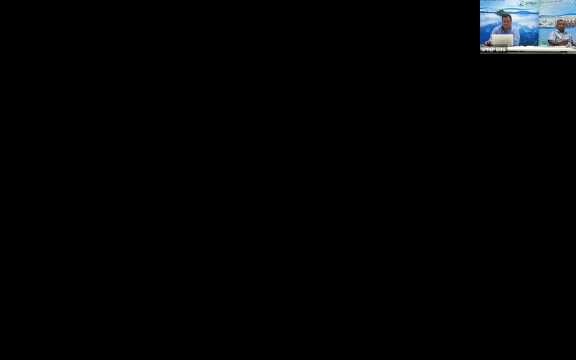 So that's what we're doing, Thank you, Thank you, Greg. Thank you, Deborah. Thank you, Greg. Thank you, Greg, And thank you, Greg as well. Thank you again, Greg, for all the amazing insights that you've given us in the last 6 months. 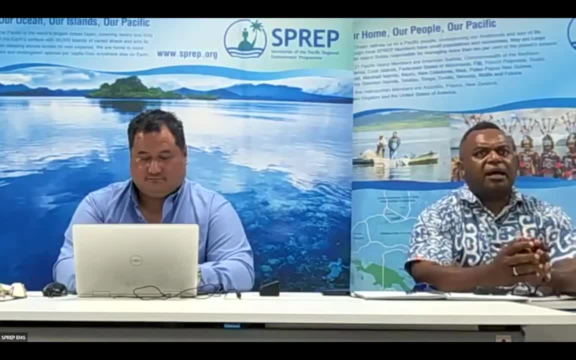 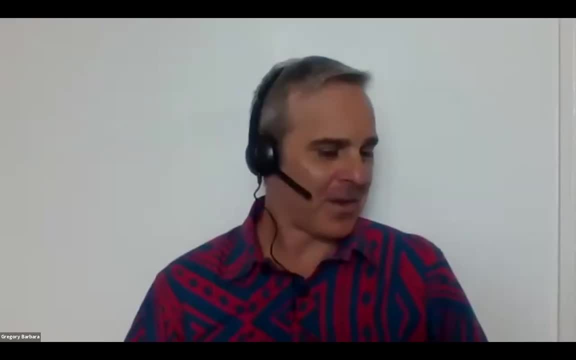 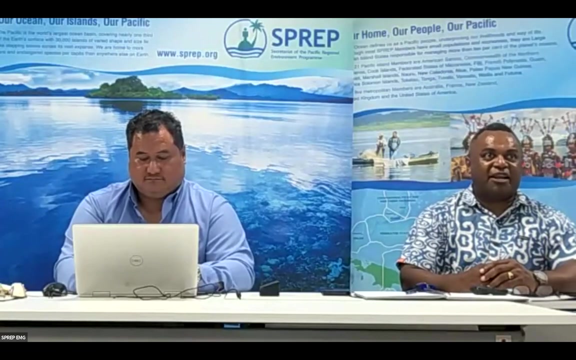 Thank you. Thank you very much, colleagues, And that is. that is a run-through of the slides presented, prepared by Dr Craig, about part way through that. really sorry, i had a systems question on the laptop, but uh, i'm really glad you were able to to uh jump in and uh cover for me in my absence, please, while you are online. 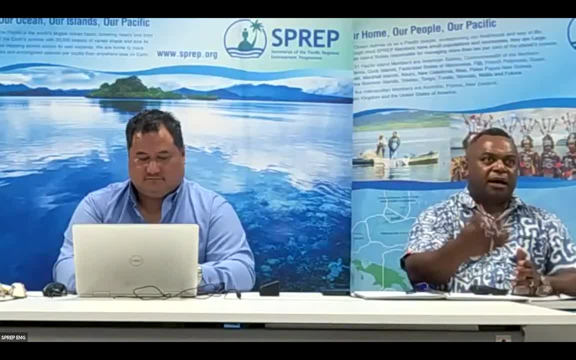 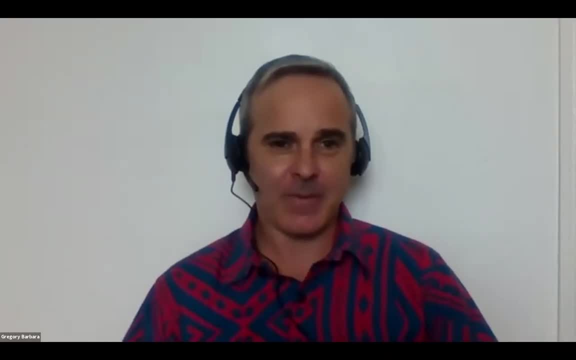 now please, uh, you can revisit, you can revisit and uh, uh, continue with the talanoa. i just went through the slides and, yes, don't get that uh with, uh, the approval of mr moderator. yes, of course, of course, please go ahead, thank you. thank you, mr, my good to see you. so, uh, so yeah, thank you for for. 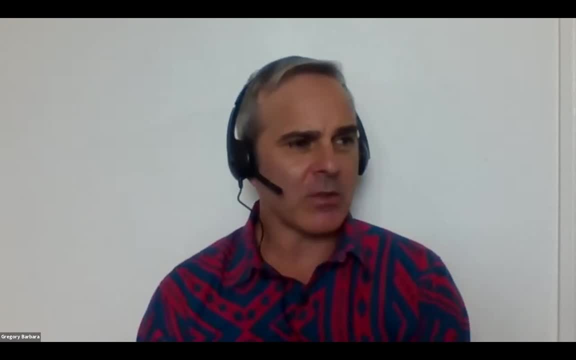 stepping into my in my absence. um, yeah, so hopefully, um, our slides gave you a a bit of an overview of why you need to do it, do a scoping, and how, um it's important to do it. um, so, the key elements that you need to put in there, although we didn't go into specific project examples, although i did. 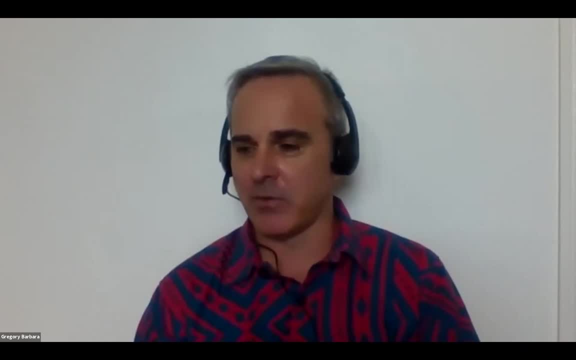 hit joppa, provide something examples? um, particularly referring to yesterday's module on gis. um, we will talk about that during the talanoa. hopefully my other panelists are online too and they'll be able to provide some examples from adb as well as usp's experience. um, yeah, the key element is when you're doing. 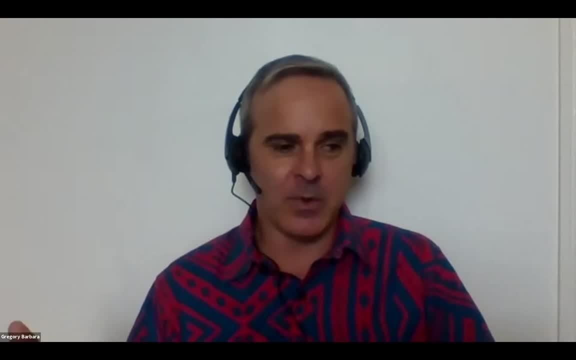 your scoping. we do have a template that spread provides um you look at what is relevant to your project. so if that, if the legislation or the templates that you're given when you're you're drafting up your scope of works, um says something about marine studies, um check, because it may not actually be. 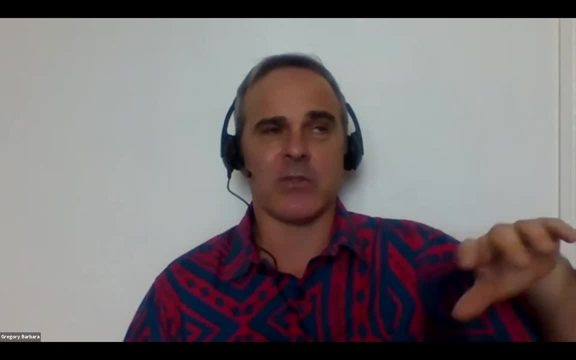 relevant to your project. if it's not relevant, you don't have to worry about doing marine studies. for instance, if you're up in the highlands and you're doing um some log logging clearance, unless you anticipate they're going to be huge amounts of runoff going into the river and impacting on. 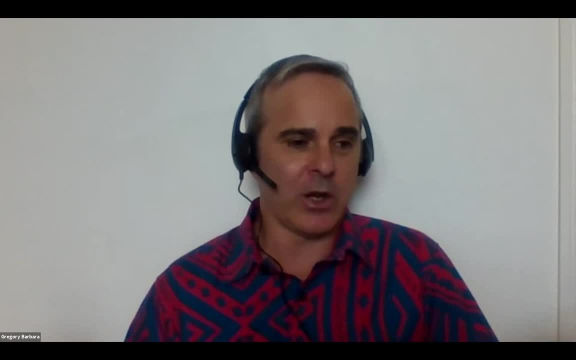 a reef that's nearby, then you you're unlikely to need to go out there and do hydrographic surveys to see if there's potential for smothering, but you're unlikely to do all the other surveys that are required for marine project. likewise, if you're a marine project, you're unlikely to have to do. 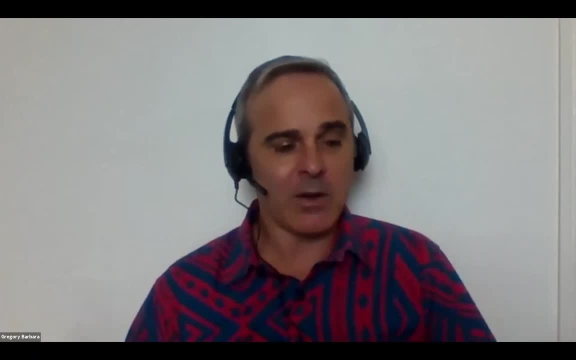 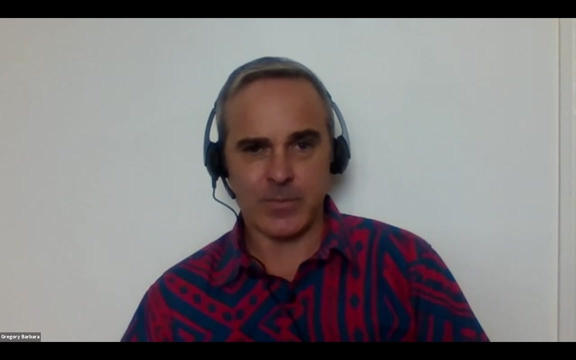 lots of terrestrial studies. so be clear on what your project scope of works is going to require, because, as joppa said, you don't want to clutter your eis with a whole heap of studies that were not needed. okay, so we can see that there's a lot of data here. 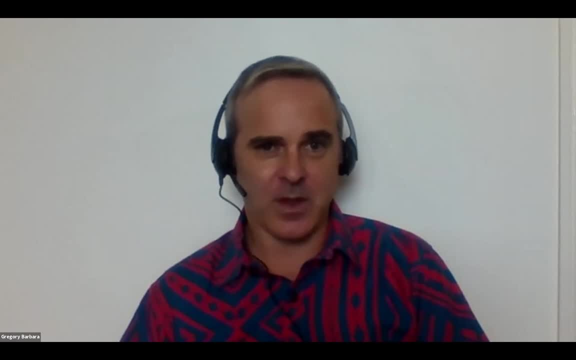 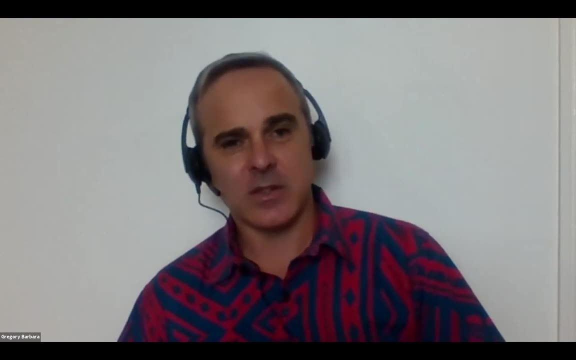 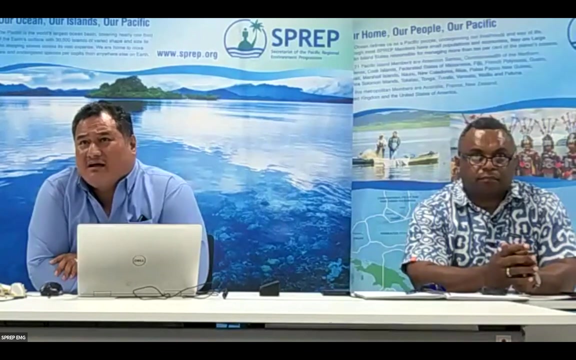 there's a few comments that have come in during the presentation. um, i might hand over to our moderator to uh take us through those to start off the talanoa. all right, mate, uh, thanks, uh, i've got a few questions, so i'll try and read it. um, uh, so we've got a question from 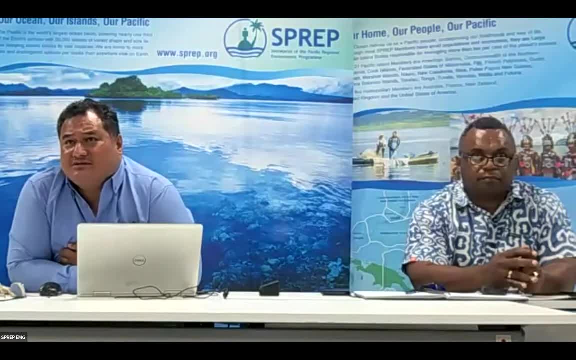 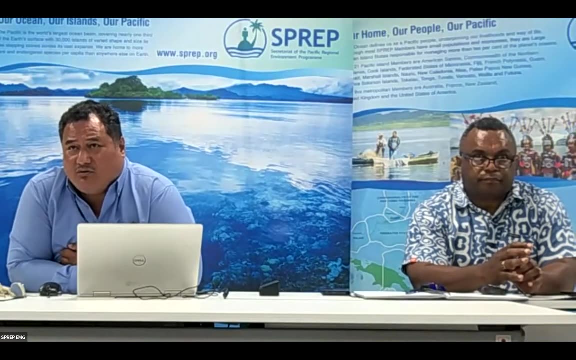 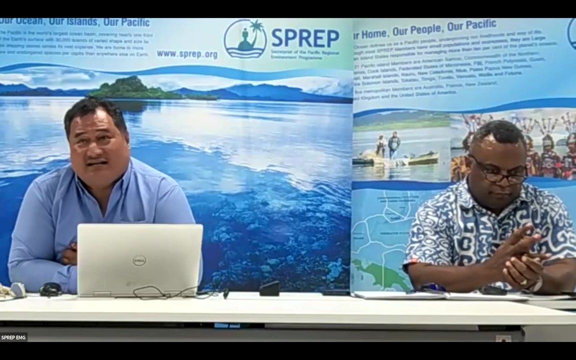 so the question is: can an eia consultant on behalf of the proponent challenge the terms of reference issue by the approving authority? as you mentioned on one of the slides that the terms of reference should be clear and precise in order, all necessary information should be captured in the eia report and avoid unnecessary information. that's an. 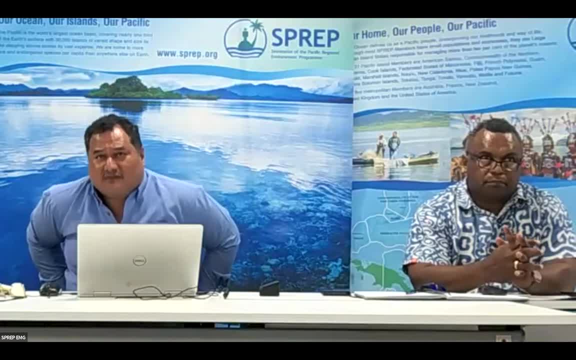 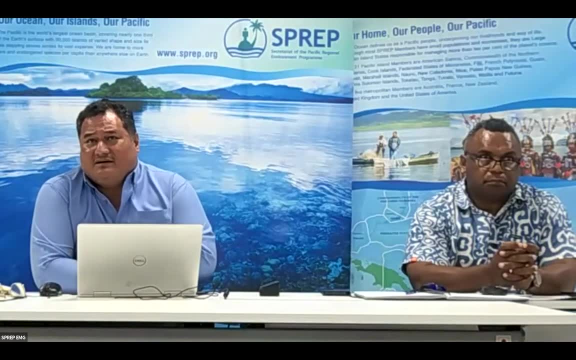 excellent question, uh, so i'll uh sort of go around the table, see, uh, if anybody has any sort of response to that. greg, do you want to have a first shot at that one? yeah, sure, it depends on your jurisdiction, on the process, that you do that. but yeah, you can do that in my 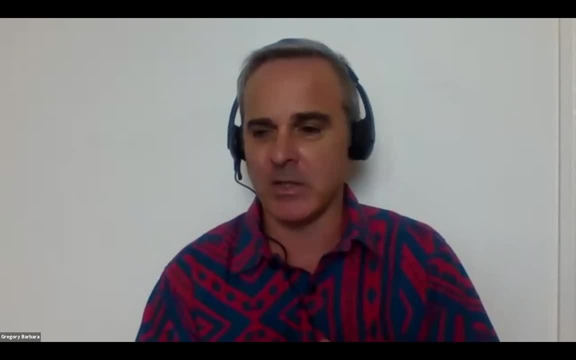 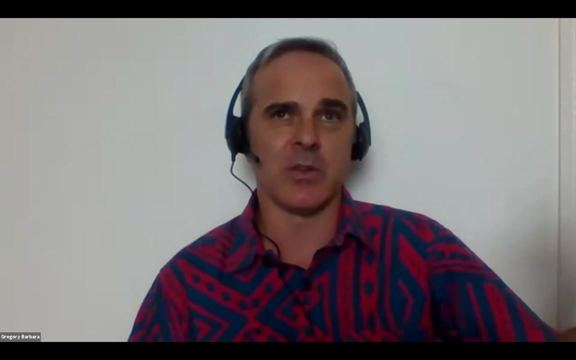 previous life as a consultant and developing up eia. you can um go back. i wouldn't call it challenge the approving authority, but you can go back for clarification on the tor. normally you do that through the proponent or the proponent has to give you specific authority to do that um the consultant. 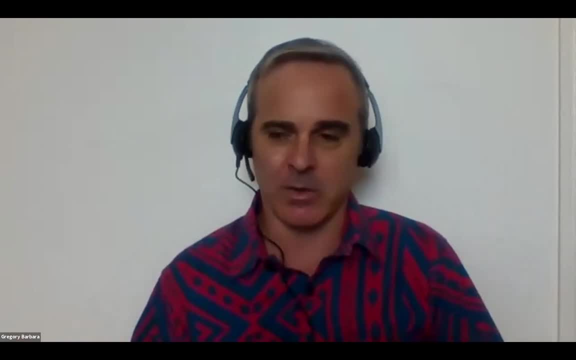 yeah, it's. that's a little bit tricky one in regards to when you're allowed to actually do that, so you'd have to be given explicit approval from the proponent to go back and seek clarification. you're challenging the tor, is it's? it's that that's more for the proponents territory? um, but the consultant can definitely advise that. 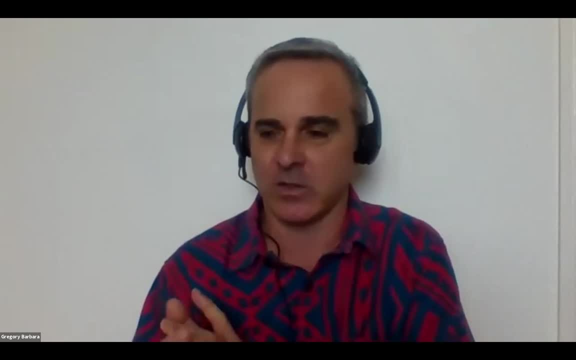 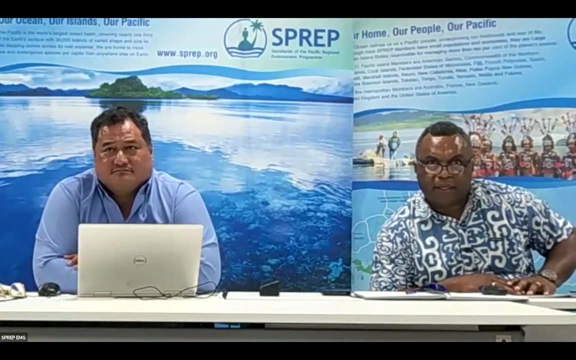 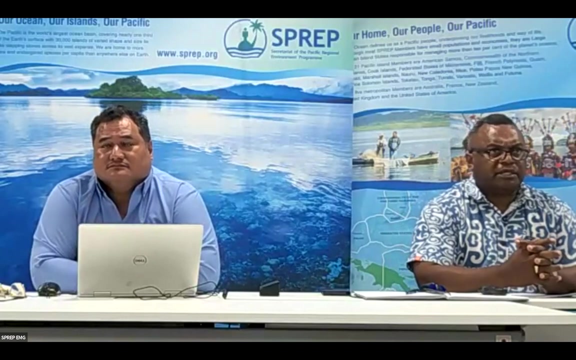 this. this tor seems a little unclear. we need some further clarification. all right, any other comments to add on to that? thank you, uh, greg, and may i say uh, thank you very much, mr. This is an excellent question indeed. it is really indeed an excellent question. 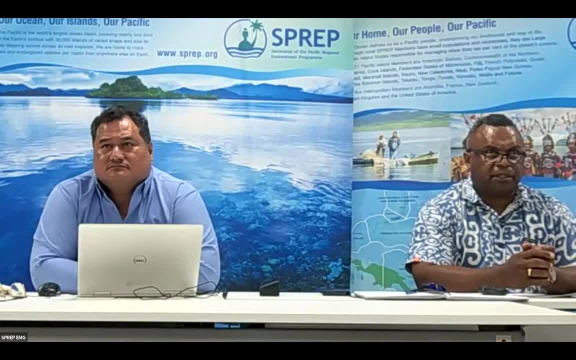 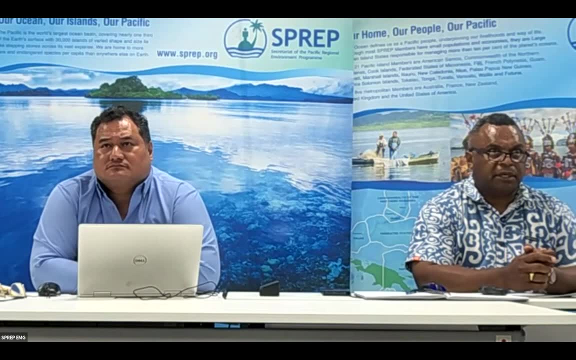 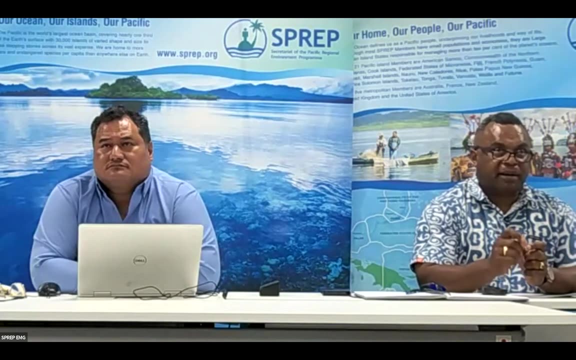 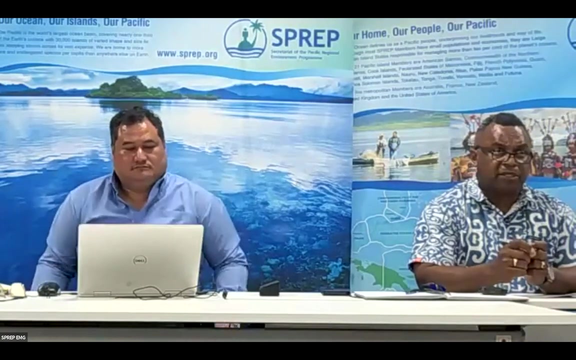 And, yes, similar to Craig, in my past experience working as an EIA regulator, in some instances the consultant on behalf of developer, questioned why some studies are reflected in the T1. And we, as regulatory agencies and supporting agencies and stakeholders must be well aware. 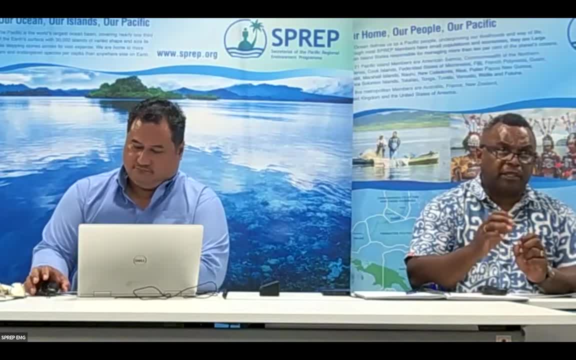 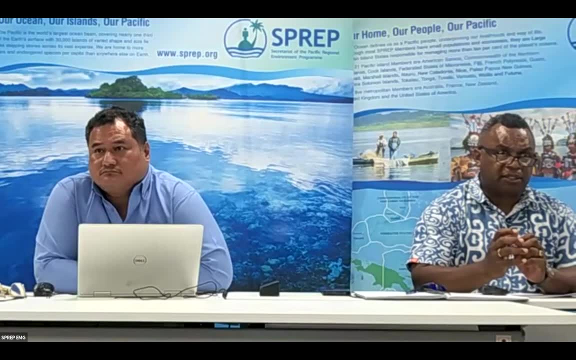 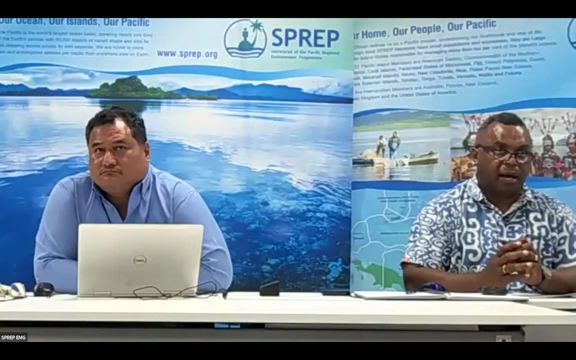 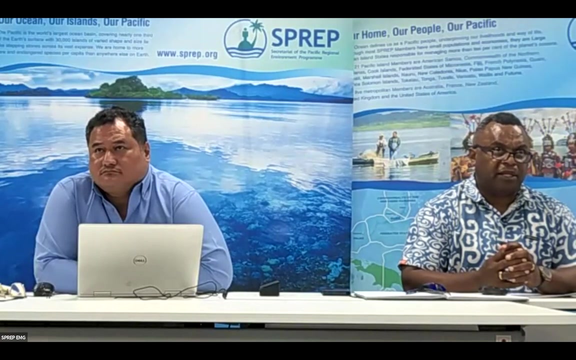 that's why it's really important to do a desktop analysis, understanding of that particular development. When we are questioned, in this instance, we have a proper reply, proper response to address that question. I've been through that And yes, And that is why I raised in one of my discussion points that even the developer and the consultant 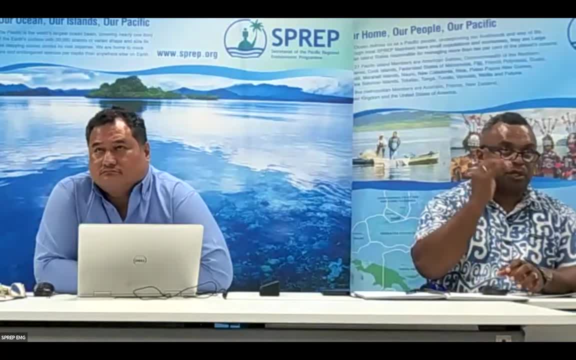 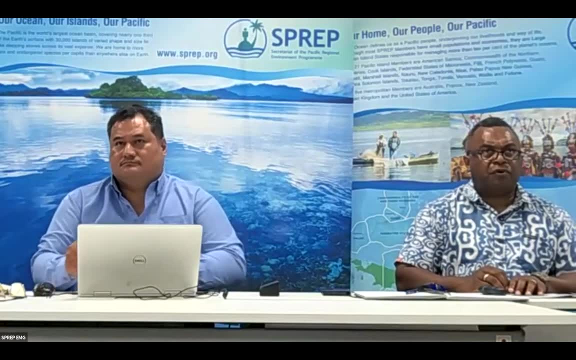 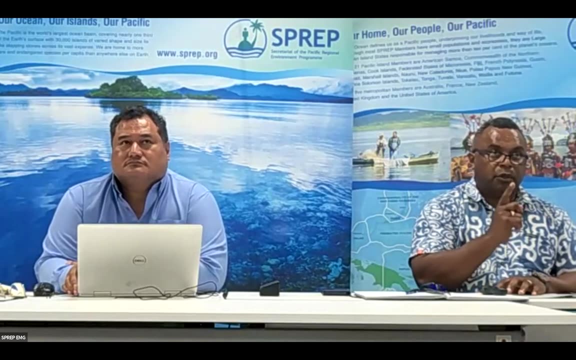 can come and be part of the scoping exercise so that we deal with issues on the ground. before it's being put on paper And before the terms of reference is finalized, it's circulated to all the scoping team for them to approve, And that's where the question, or say, using the terms of reference, it's circulated to. 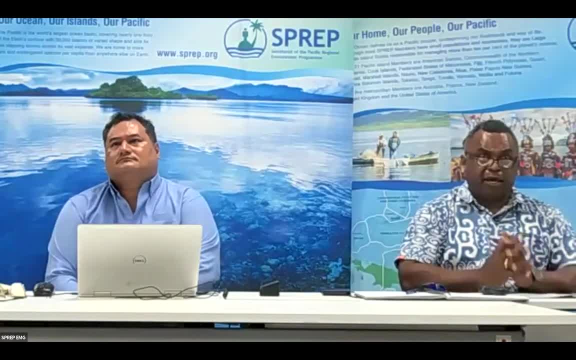 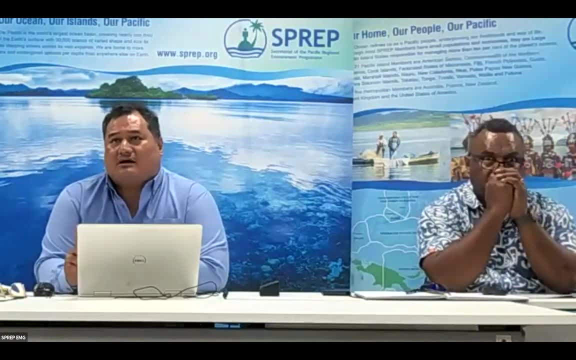 them or it's not circulated to them. So, yeah, it's a very different way of dealing with the terms being raised challenged. But yeah, that is how this system works in my experience. Thanks, Hey, Nick. I see I think you have a comment, so I'll come back. 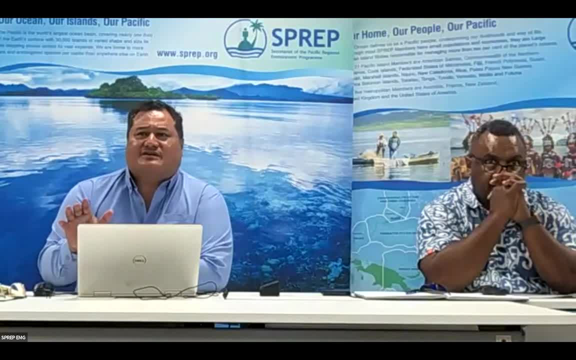 Perhaps you can put on your video before that. I would say that you know that word challenge. it's really sort of focusing on whether the consultant or the proponent does not like a particular condition placed on the terms of reference, a particular activity that's on terms of reference. 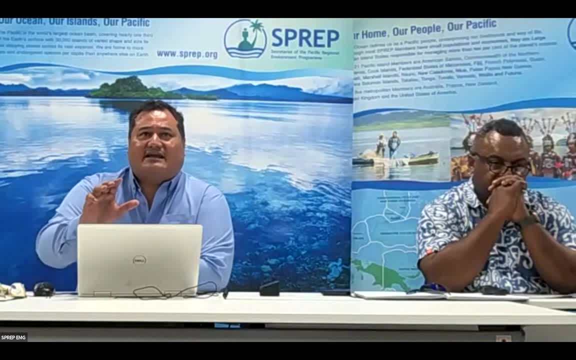 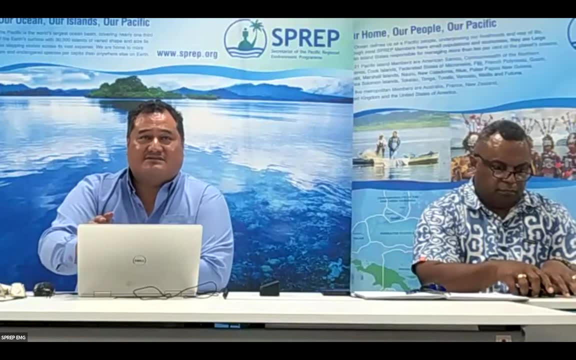 It's just a very complicated process And it's hard to understand, right? Yeah, and in that case it's really sitting down with the regulator and asking for clarification why that particular pose has been put into the terms of reference, given that the project is this and 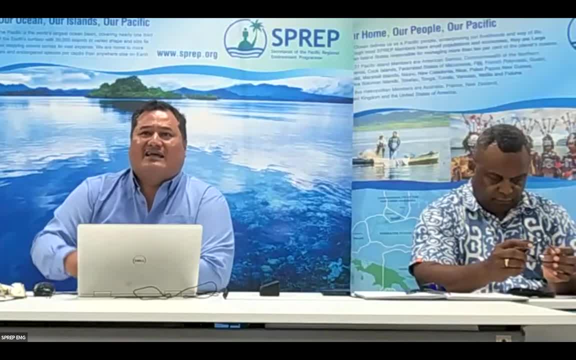 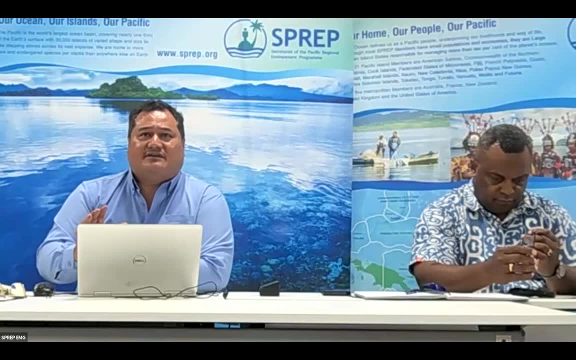 that and this and that, so the scale and scope of the project becomes very important. if it is a condition that is placed in the terms of reference mandated by law, that would be tricky, and that's something that would become compulsory and mandatory, and so the regulator would just sort. 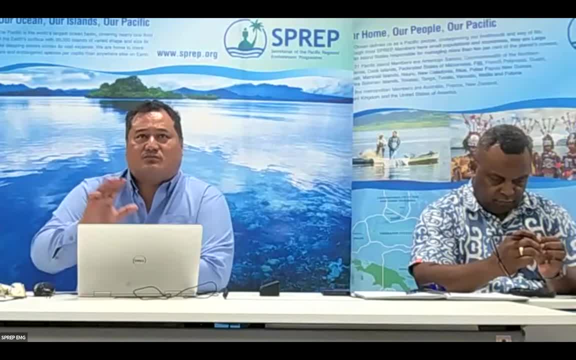 of respond. that's the law. but if it's sort of activities, why are we doing this? why are we doing that? it's the regulator's responsibility to explain and clarify, uh, what that is, and then perhaps you know, through that conversations you're able to come to a consensus. uh, nick, can i have you? 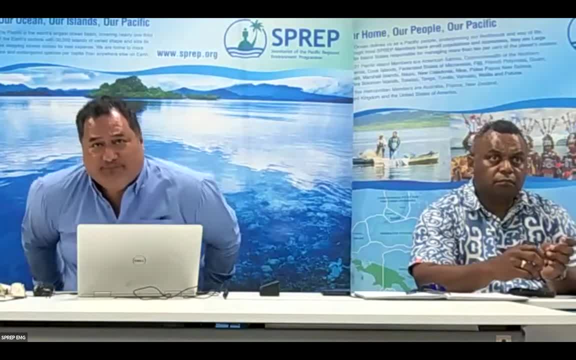 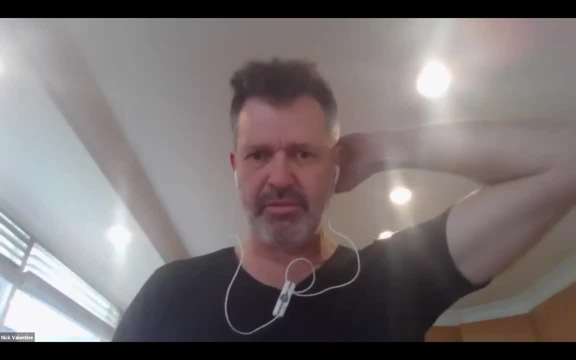 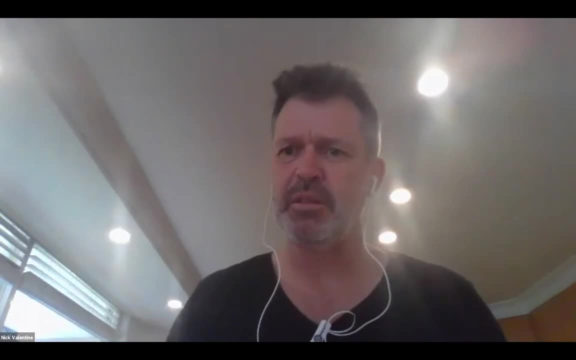 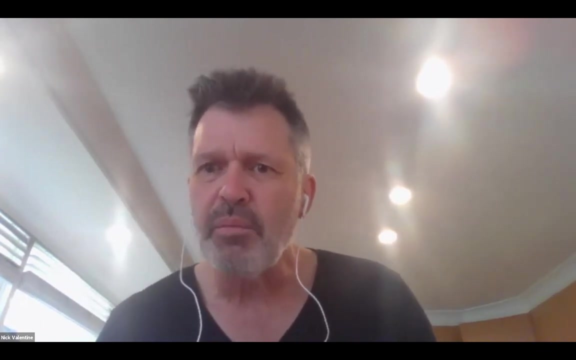 come online and offer. i see you have a comment. best to verbalize it from the morning: i need nick for the world bank. uh, how are you all? good, thanks, good, good, um, sorry if i'm answering your questions for for you, but, um, just a few comments. 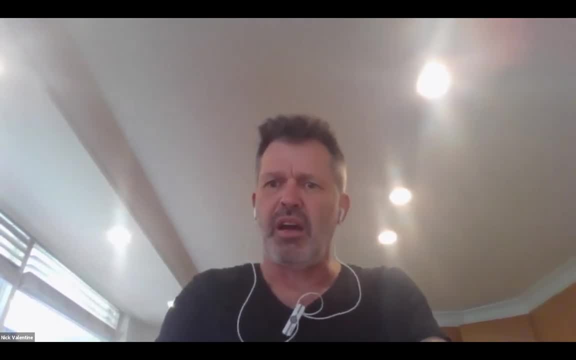 um to keller calio's question, i think um the tor should always invite comments from the consultants. that's why we're going to consultants in the first place to provide expertise. um invite that on the toa. um so as a normal practice. um the question from james where he talks about uncertainties, eia's. 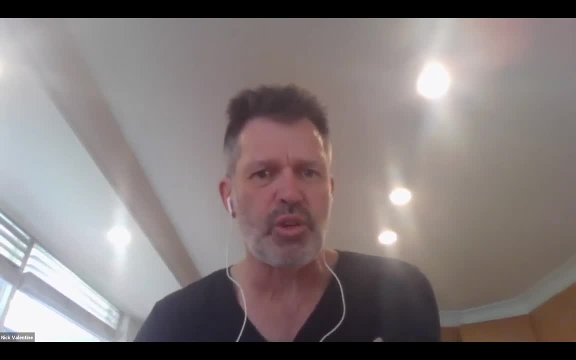 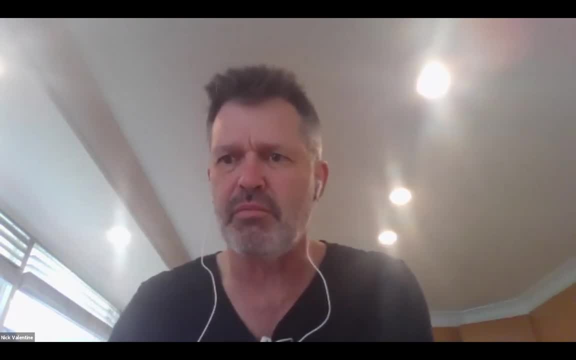 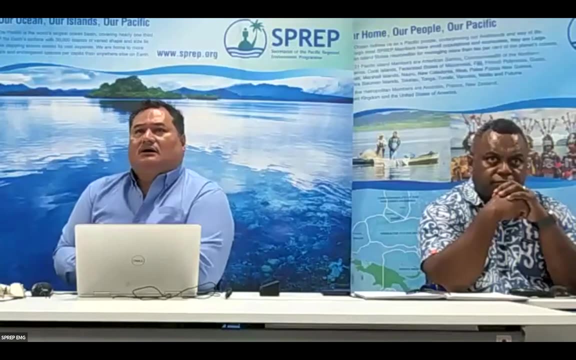 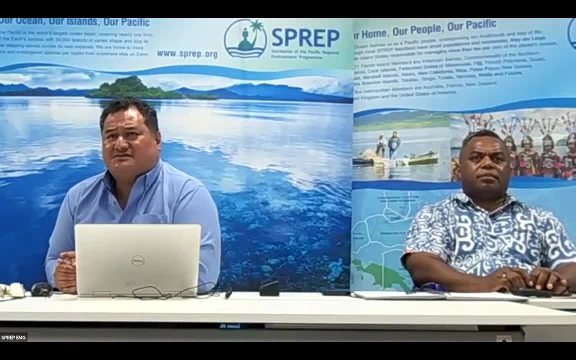 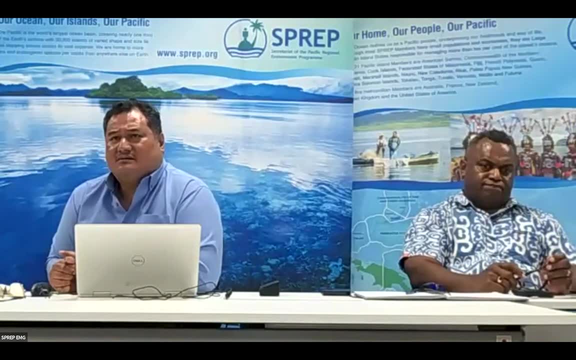 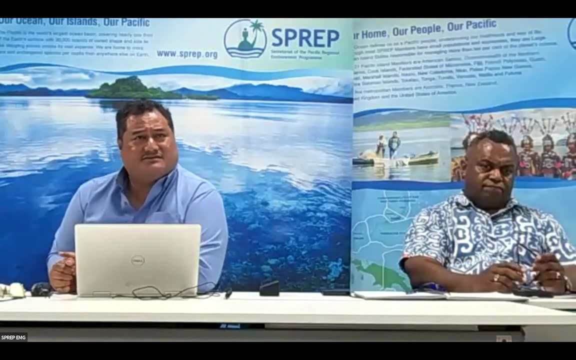 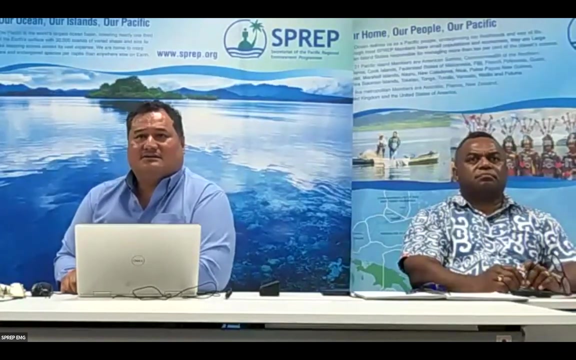 i think in assignments. how do you deal with uncertainties in eias, any case studies? how can the developer deal with those deviations based on inaccuracy or prediction in the eia process? this during implementation stage, any takers? that's a very, that's a very uh uh. good question. um, i don't think you know. 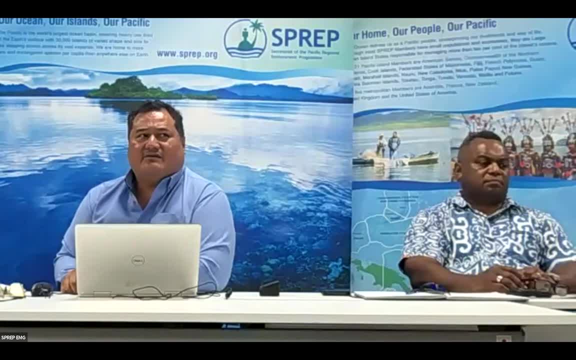 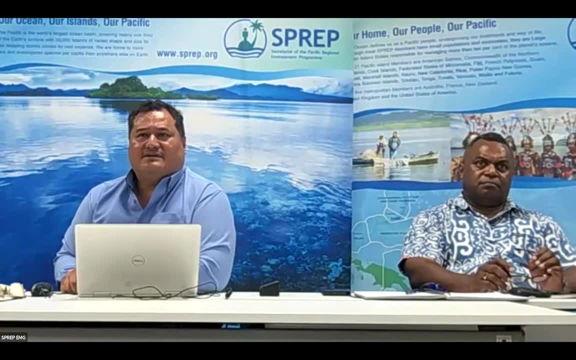 doing proper scoping is addressing every. you know should address uncertainties. um we you usually, where there is an uncertainty, you adopt the precautionary approach and that assume the risk is real and natural until it is proven otherwise. so that's really something. that's where the precautionary approach kicks in. 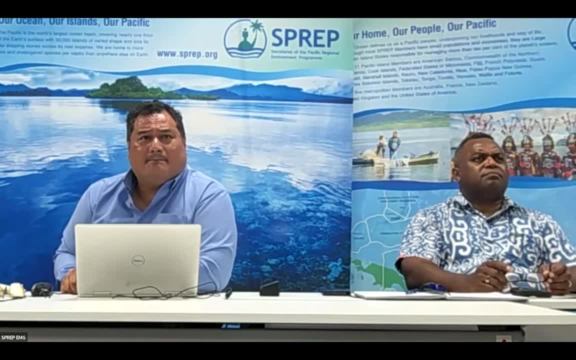 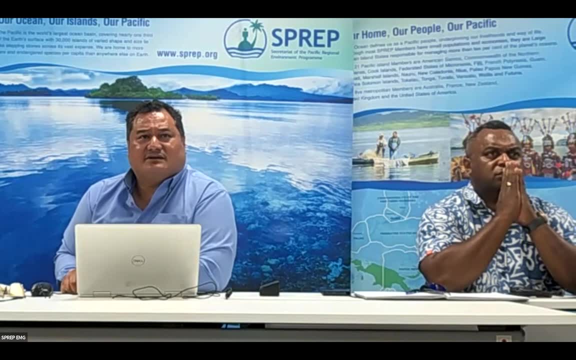 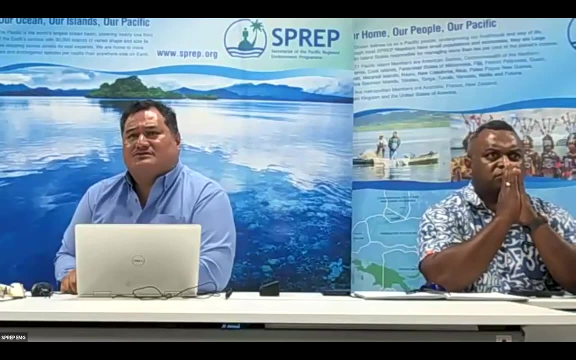 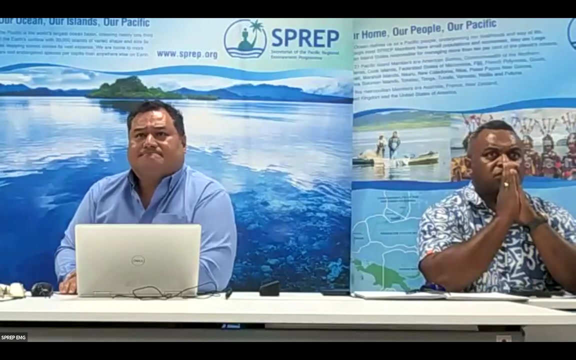 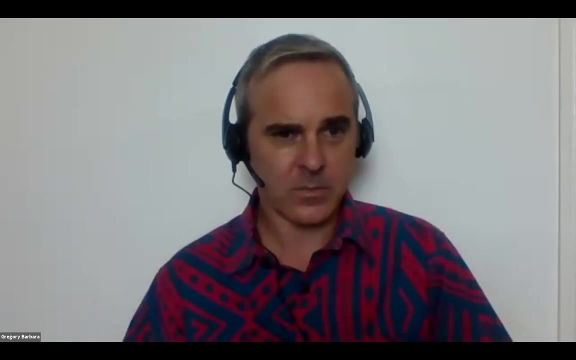 can, uh, can you enlarge that please? um, yeah, so um, and how can a developer deal with the deviations based on the inaccuracy of deviations? uh, listen, james, um, i'm, i'm, i'm going to say sorry, a good question. see, these are all assistance h, so many DIYs that don't get dying. is that okay, karen? will you turn it on for you? in five videos at the moment, please, uh. so i know we're still uh blind for about five minutes, so i'll tryktosh�� on the spot. can you come online and explain a bit more about what that is? that seems to be like a really good question, but provide a bit more context for our trainers to respond. is that you j uh? can i get james online please? hello, james, are you there? hi hi, james. are you there now? are you thereァ? 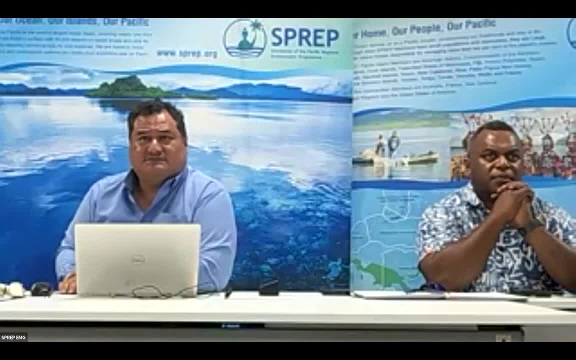 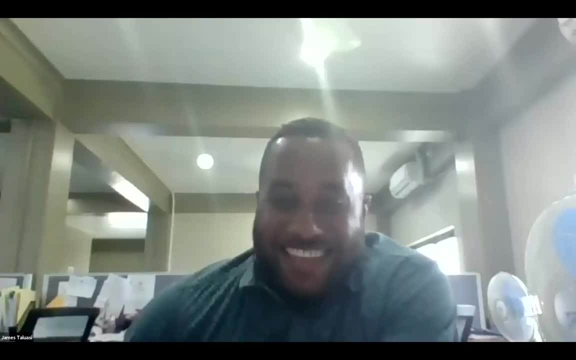 hi, hi, hi, james, are you there too, of course, is that you're on the chat? Thanks, Can you put on your video please? Hi, buddy, Hi, how are you? It's good to see you. How's Tina Hydro? So you've got a really good question. 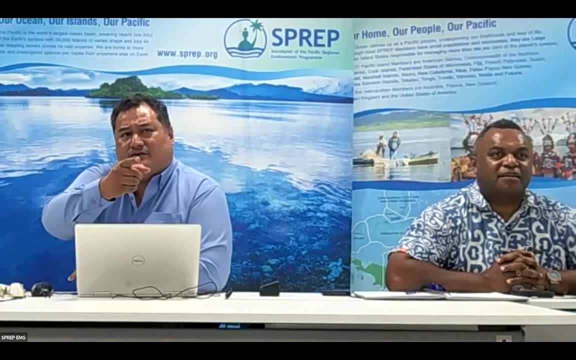 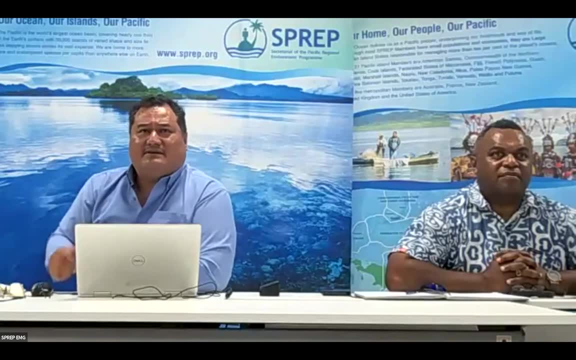 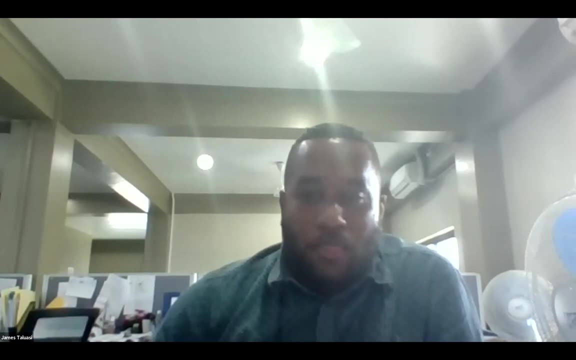 But could you that question you have: how can the developer deal with those deviations based on inaccuracy of predictions? Can you explain a bit more about what that means? I think just referring to like mostly in terms of scoping and to do with content and extent of how to mitigate. 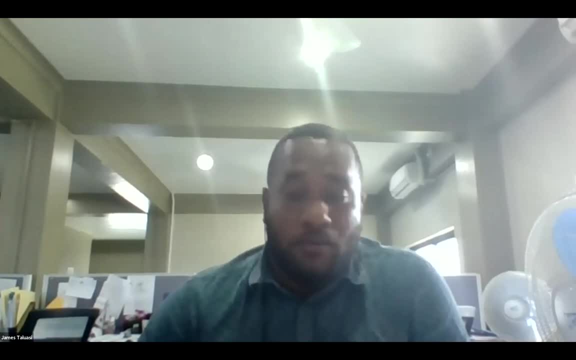 the risks that involve in the project. What I'm referring to here is there will be some, you know, if the there'll still be some inaccuracy of how we predict the possible mitigation measures for those, you know, when assessing the risk. 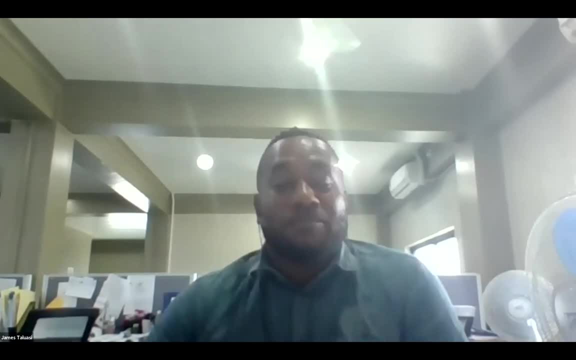 So later on, in the post implementation, there are some issues that came about during the project implementation, which is normally, we refer back to the EIA. So that is where my question coming from. So how do we, you know, deal with those inaccuracy of prediction during the EIA post? 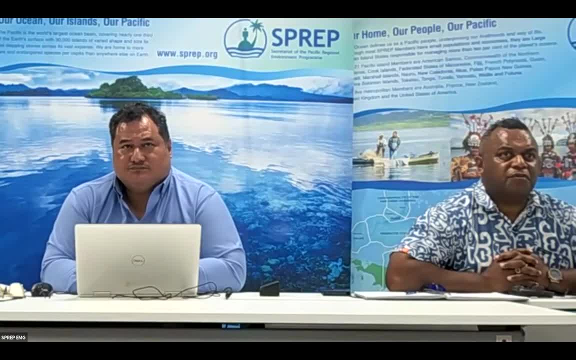 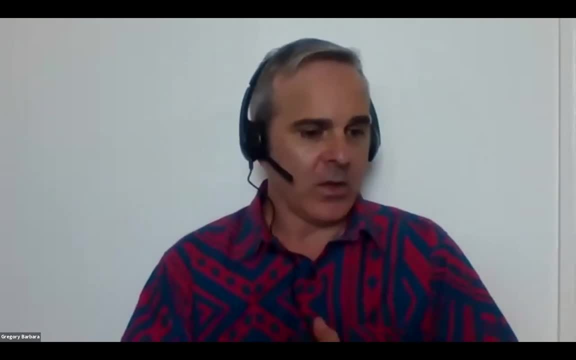 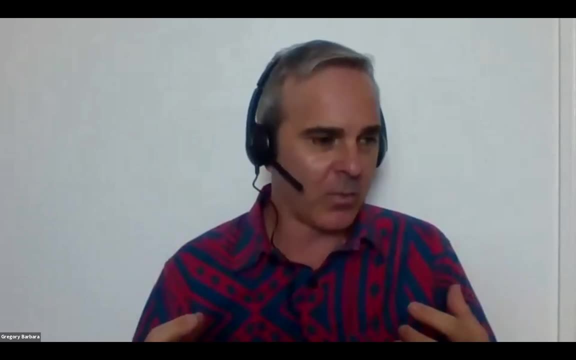 It affects the implementation of the project. Go ahead, Greg, If I may. I think I understand your question there, James. So yeah, it's a very common problem and it's an excellent question. So just let me summarise what you said, just to make sure. 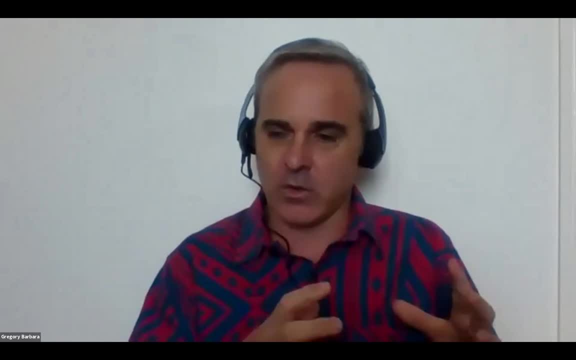 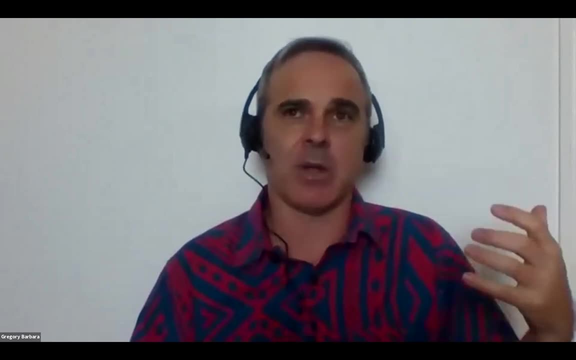 that I'm understanding you correctly. So your question relates to once the EIA has been completed and then you've been given the expected outcomes, expected mitigation and the expected impacts from that project and you're now commencing the project. how do you deal with deviation? 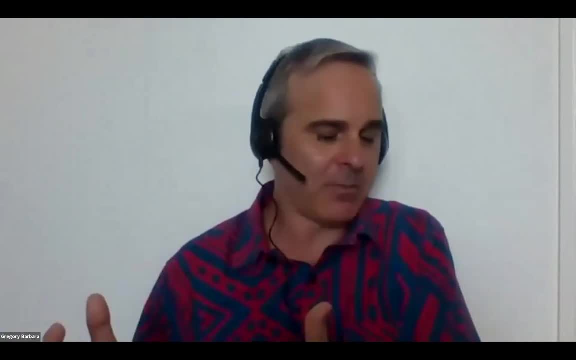 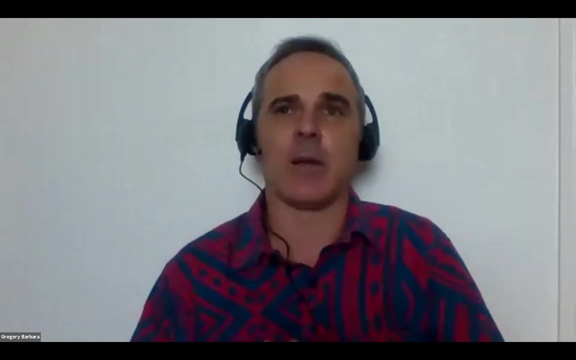 So when you start actually onsite and you're in the midst of construction, you discover that it's different to what the EIA had predicted, Exactly Right, Okay, So that is a common one, especially when there's a lot of paucity of information. 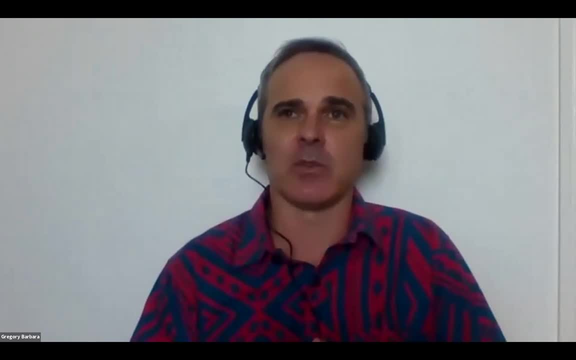 when you're doing up the EIA, and that happens a lot in the Pacific because we do lack a lot of data. So the scoping phase can help a little bit by making the studies broad enough but focused on what you think are going to be the key problems or the key impacts. 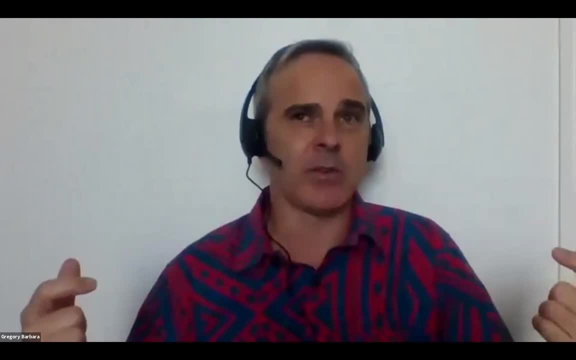 and the key benefits of the project. Sometimes, however, what happens is the team becomes so focused on what they think the project's going to be. they kind of put the blinkers on and they don't take into account of all the other things that are going. 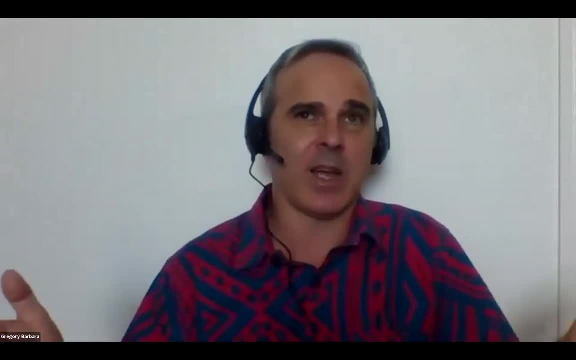 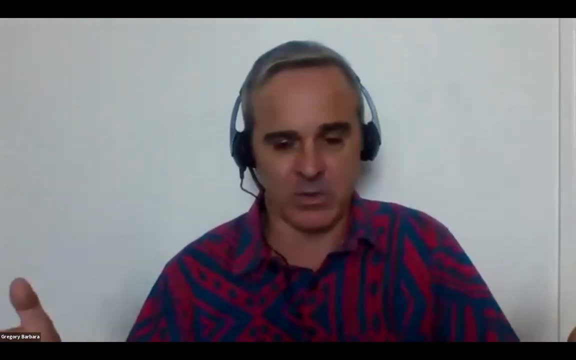 on onsite, because that's what the TOI said, And that comes down to scoping, understanding your location and the project and the project risks in the wider context, and making sure it's refined. What you're talking about, then, is what happens then. 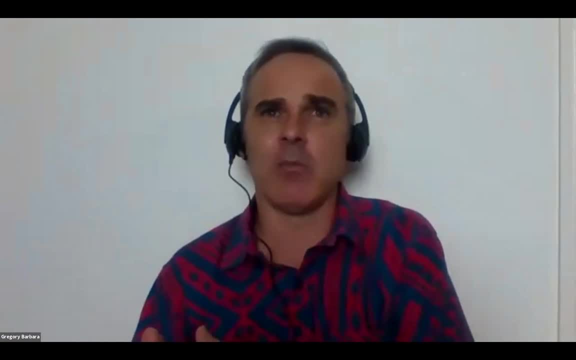 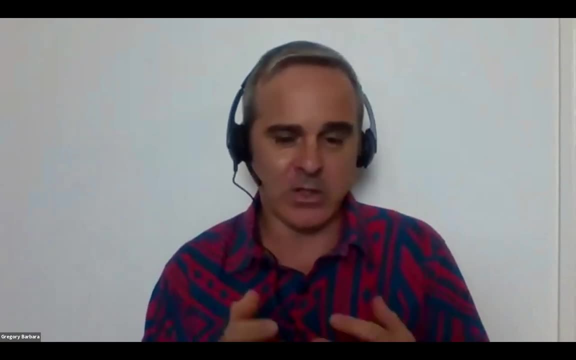 How do you deal with that? So we're going to be dealing with that, I think, in Module 14, when we talk about environmental monitoring and management plans. Now, this is the document that you develop alongside your EIA when you're doing your impact assessment, which is your. 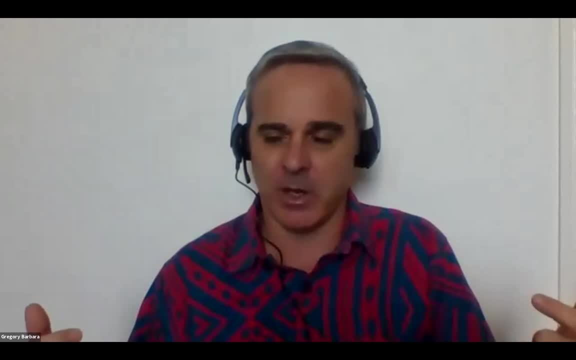 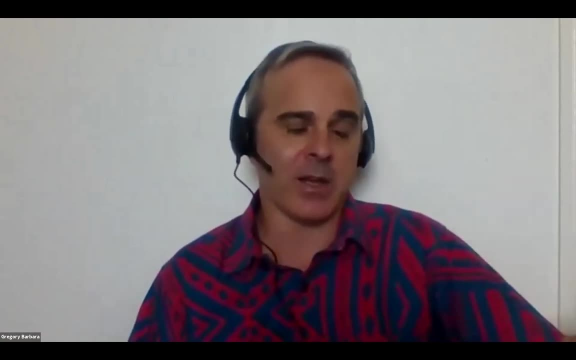 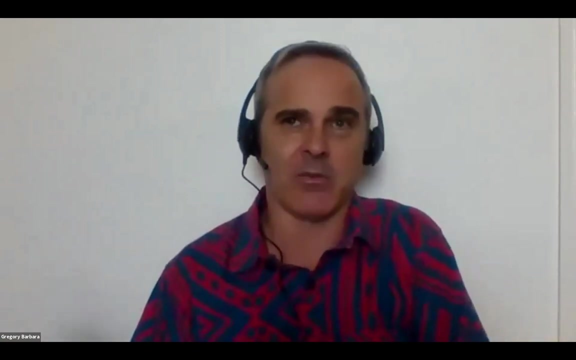 how do you monitor your project as you're developing it and as it's running in an operation, and how do you manage your impacts and how do you check and go back and have a feedback loop for correcting any actions onsite? So perhaps you didn't accurately estimate the amount of rainfall. 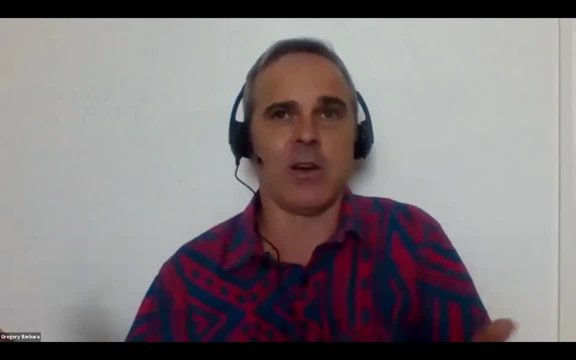 and the amount of potential erosion that's going to come down on the site, and now you've got to figure out ways to deal with that. Well, that's what the EMP is about, and that's when you have the monitoring and management plan in place and you have a feedback loop. 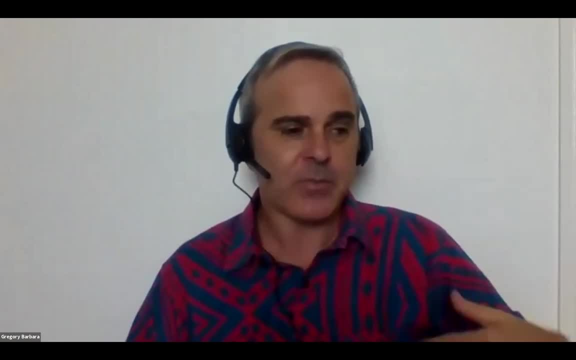 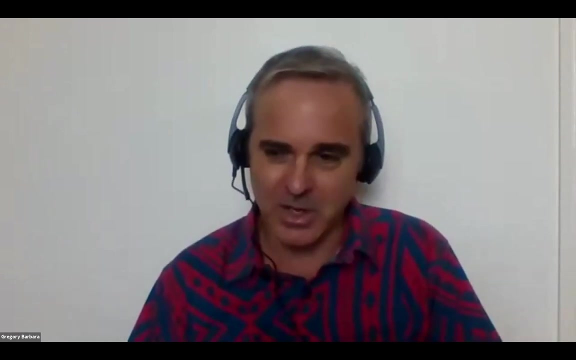 when you realise it's not performing the way it should be, you go back and you reassess and you do a refinement of your mitigation plan. So hopefully that really briefly answered part of your question. I know it's a much more complicated question that you've asked. 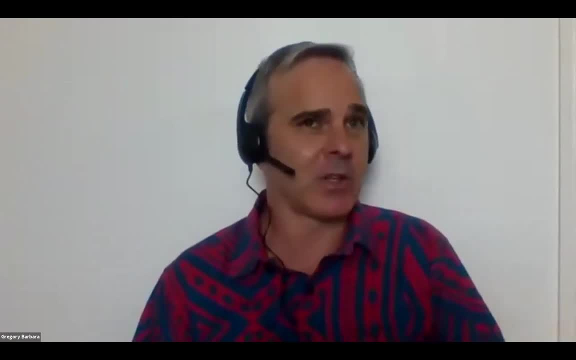 but thank you, But hopefully we'll be able to address it a bit more in Module 14.. So yeah, what you're talking about is when the EIA doesn't reflect what you find when you're in the middle of construction and operation. 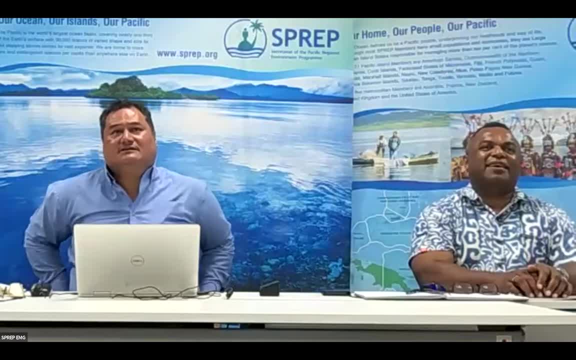 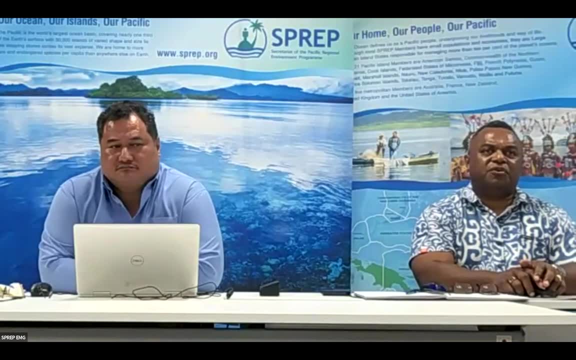 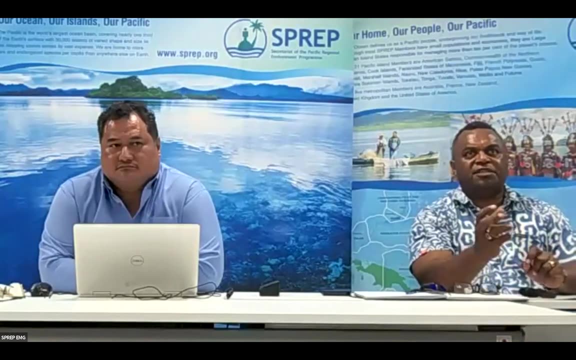 Thanks, Dr Varo. I had a moment to jump in. I'll probably chime in after, Thank you. Thank you very much for the Question 1 talk and thank you, Craig, for your contribution And if I read it, hear it correctly, you're talking about a change. 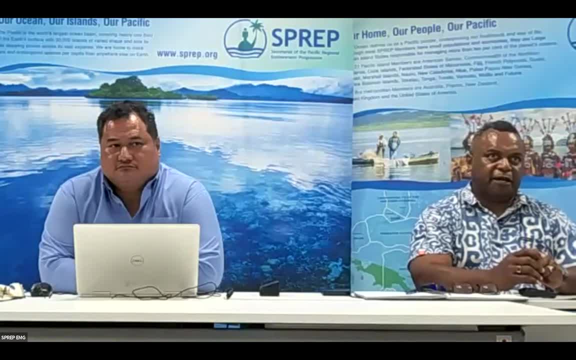 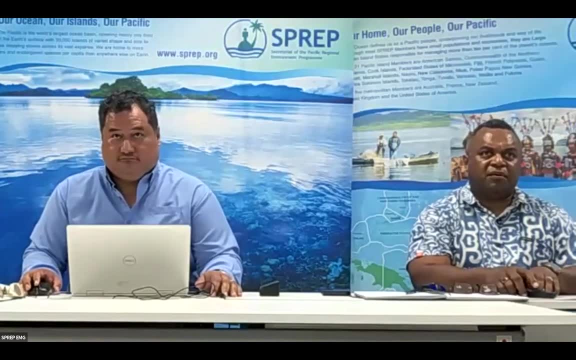 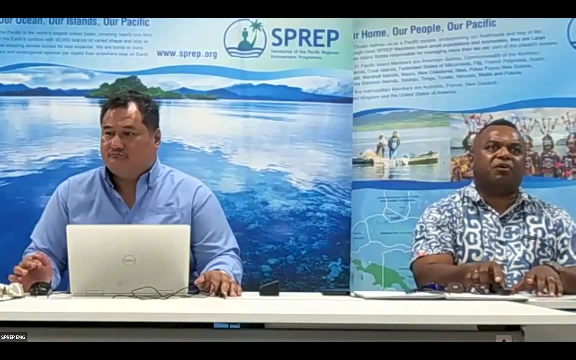 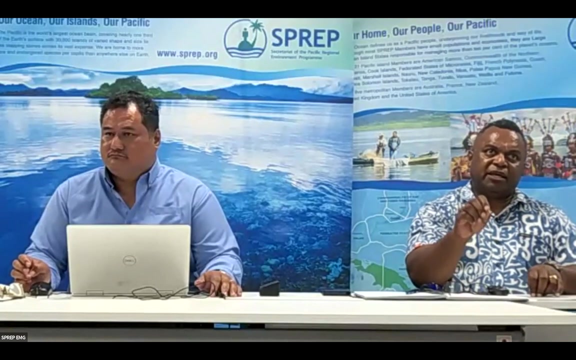 that will take place when you're implementing the project. And, yes, James, as a regulatory agency. one of the main conditions that they can put in place as part of the approval condition is the setting up of a monitoring committee to oversee the management. 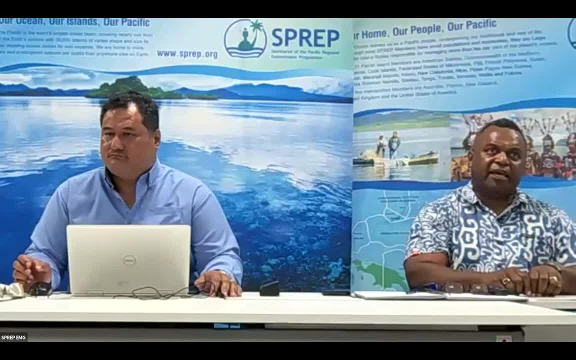 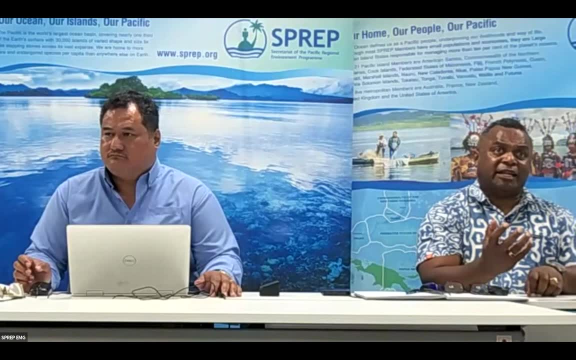 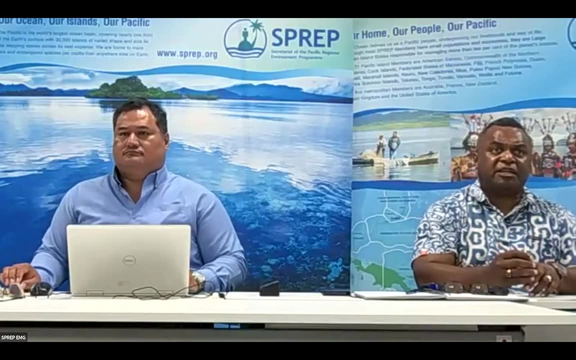 the implementation of the Environment Management Plan, as stated by Craig. So you asked the question how. That is how or one way we can address that, because you know, nature keeps on changing. Sometimes our human thinking has its limitation, but there can be new things that are coming in. 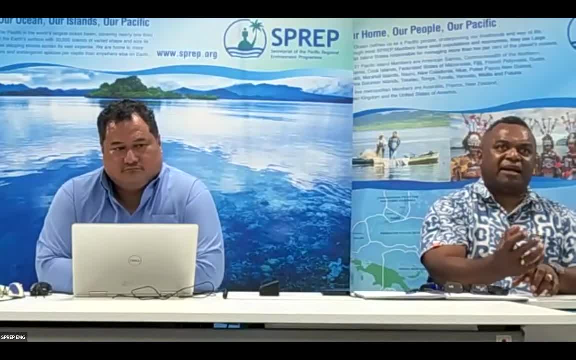 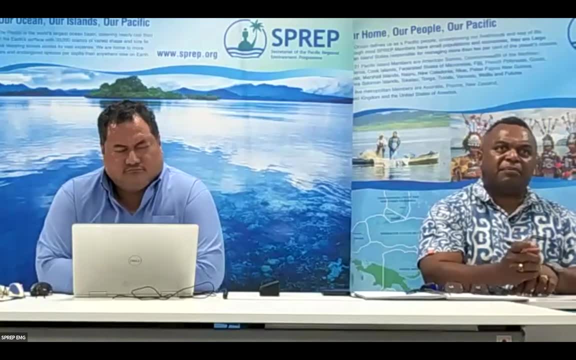 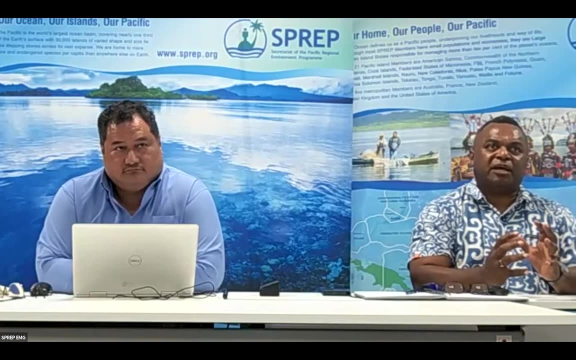 and this can only be seen when the impact arises. So there is a way- That is one way in my experience- of setting up an environment committee to meet the needs And of course there is a way to do that. but there is a way to do it monthly or regularly, depending. 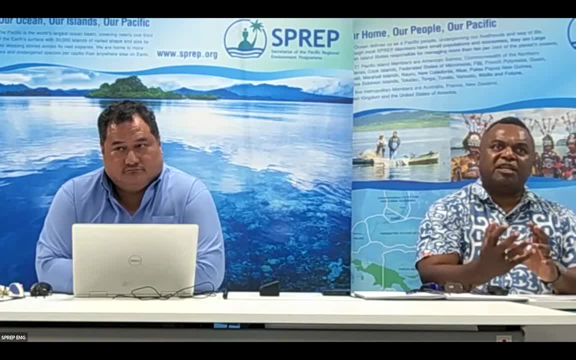 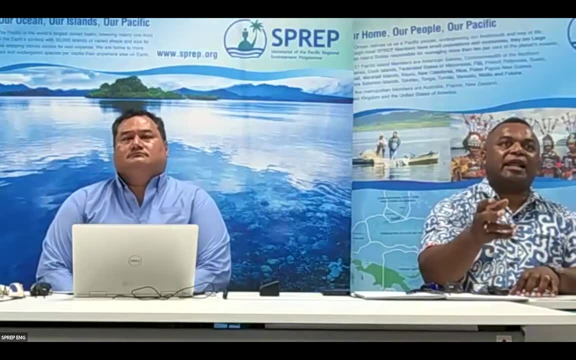 on the nature of the project Because, at the end of the day, if there is a new thing, new issue that comes up, the committee is there to address it, linking it to the existing sectors and existing legislation on how it can help with that new development. 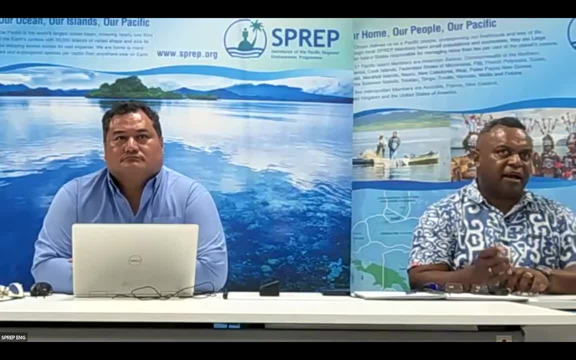 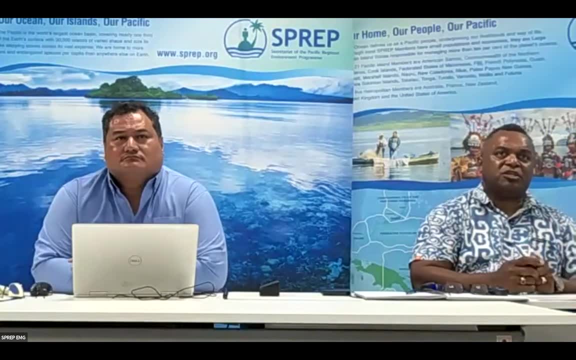 And again, James, that is an excellent one. That's something that needs to be considered by governments and the legislation, requirement or regulation, in addressing new issues for uncertainty. Thank you, Mr McAvoy. Thank you very much, Joppa. 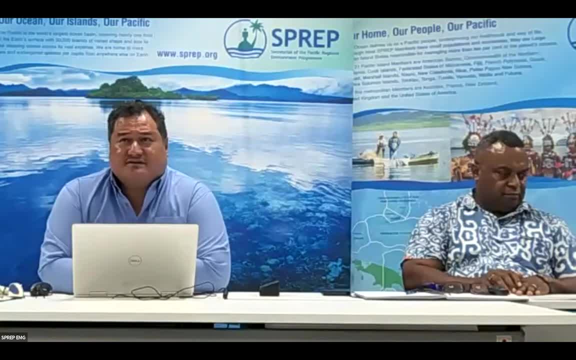 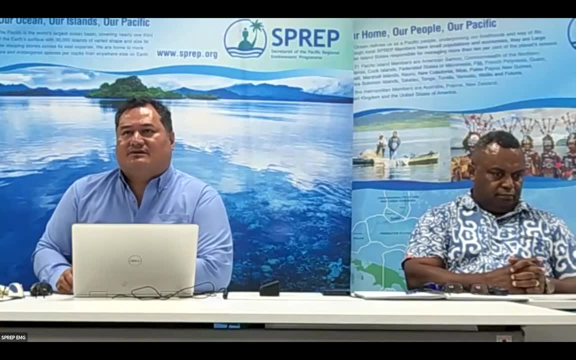 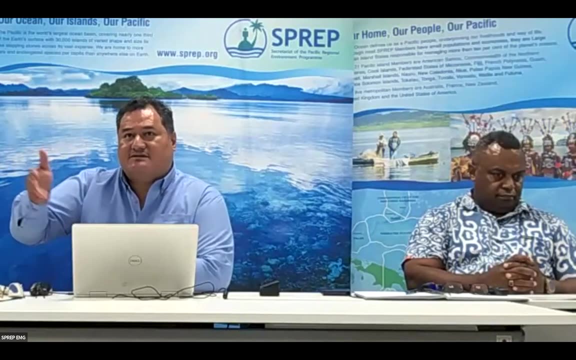 Just chiming in. so, James, I think if it's a development consent issue by an EIA regulator, the EIA regulator will define to you the monitoring program for your project, for your licence, And through that monitoring program there will be intervals for you. 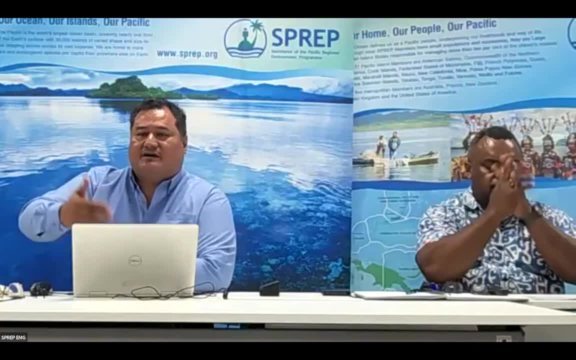 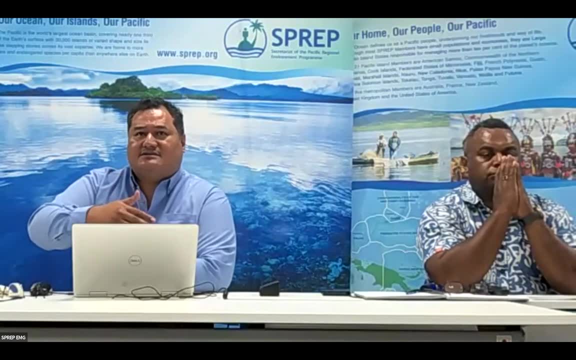 to report back to the EIA regulators. That will be sort of something that you can do Using those intervals. that's where you take reviews and you add in new things or whatnot. So it's really, I think and in terms of safeguards- 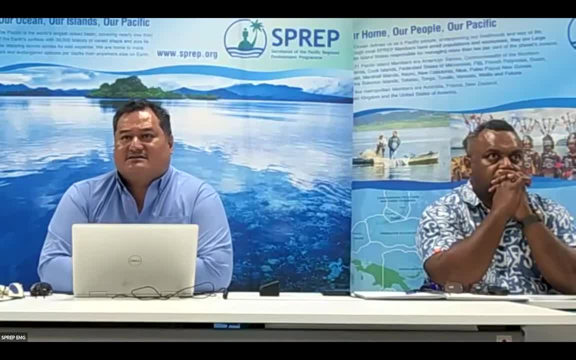 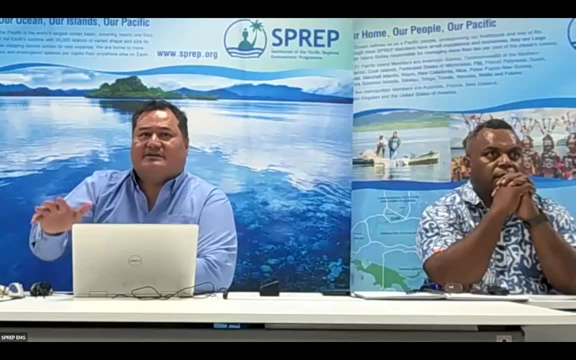 project safeguards officer. again, that's the compliance, the monitoring for compliance function that you perform. You can't predict everything. Some things will pop up that we didn't predict. Don't worry about it. Document them properly and push it up to the chain and make sure. 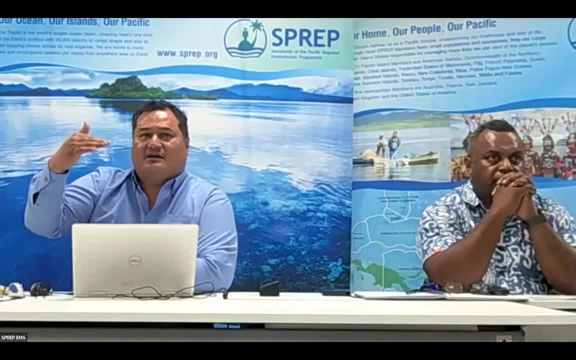 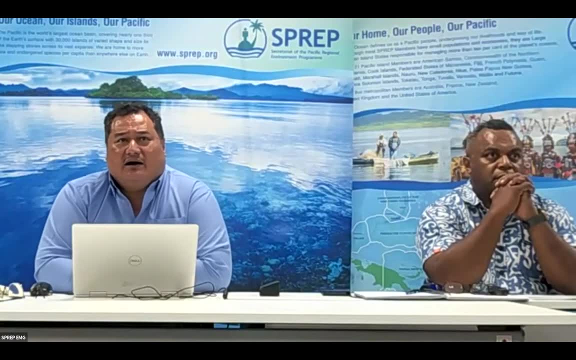 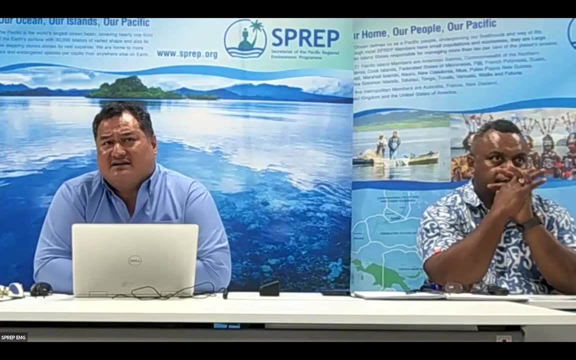 and make sure that it's that all the approval levels for that document has been submitted, and then they will provide their responses And make sure you document. I've got a comment from Nick. Nick, you want to come online? I think you have a comment there. 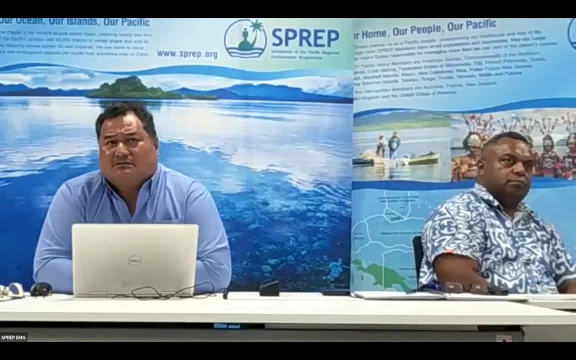 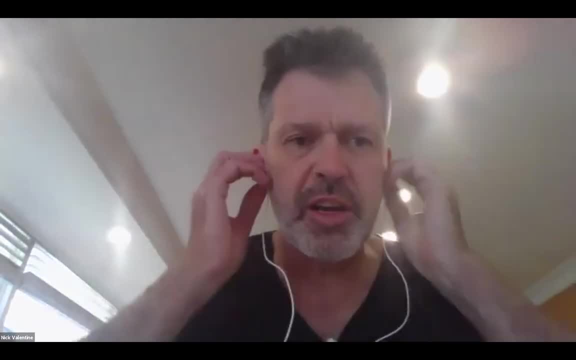 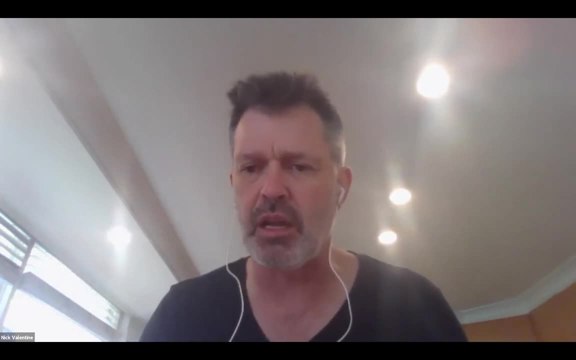 It's pretty good. Thanks, Paolo. Yeah, look, I just wanted to give an example, An example of how this can play out, based on an experience in Sydney on a major construction project. It was a tunnel underneath the CBD in Sydney called the Cross City Tunnel. 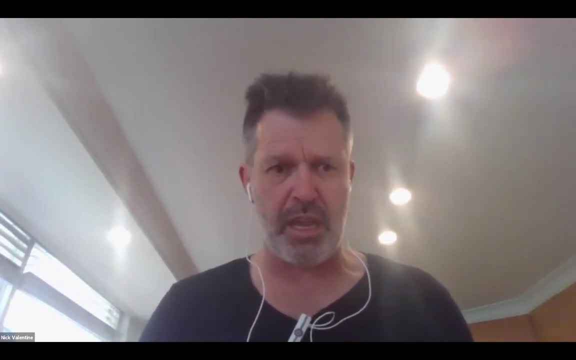 that some may know, During the course of the tunnel excavations on the western end of the tunnel they uncovered an old sandstone wall, and it turned out to date from the early 1900s, So it was a heritage site that was unknown at the time of commencement. 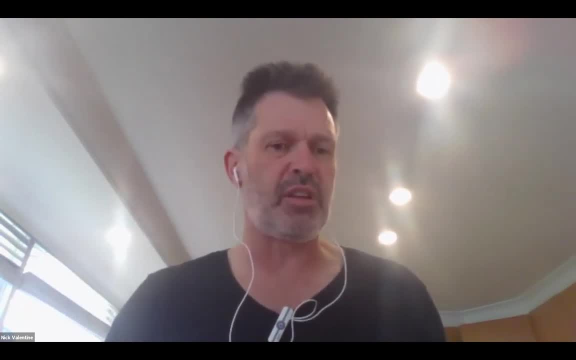 of the project and it was of significance, But it was right in the middle of where the tunnel portal was going to be, so it had to be removed. So what the response there was was initially to contact the regulator, as Paolo suggests or Joppa suggested, the heritage office. 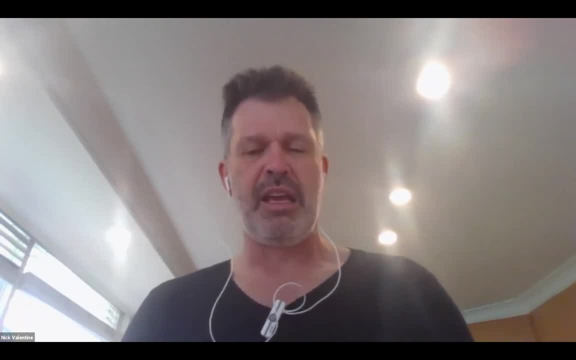 and what they resolved to do was to get a heritage advisor in and then they carefully excavated the remains and then they put them on public exhibition, if you like. So they allowed the public to come and view the historic remains and they had the heritage advisor do a photographic. 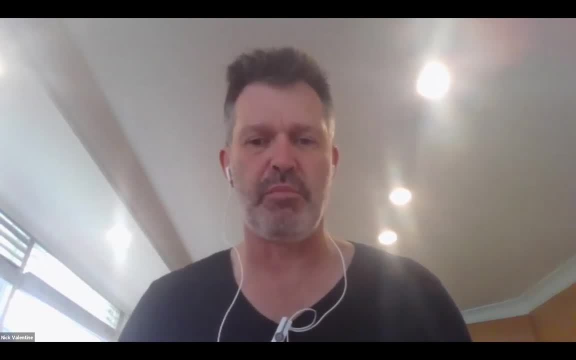 and a written interpretation of them, and then they were removed. I can't recall if they were relocated or perhaps put in a museum somewhere, But these things happen. You uncover literally, particularly when you're doing earthworks. you, You uncover things and that's why we have for heritage. 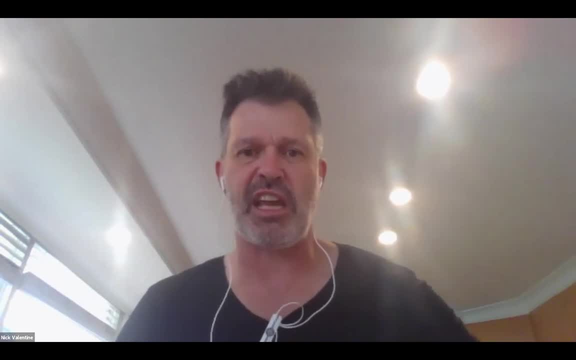 we have a chance finds procedure, because there literally is a chance that you may come across something. And in that instance, on that project in Sydney, the work stopped. So obviously the risk was that if they continued to excavate they would destroy the relics. 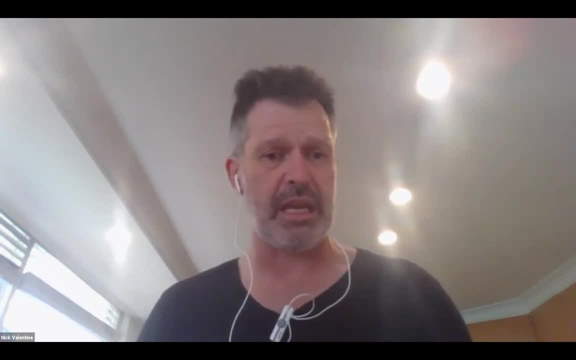 So that section of the project stopped for a period of about four weeks, I think, and that was. That's just the way it goes. right Now the contractor has recourse for a claim there, but these things arise and we just 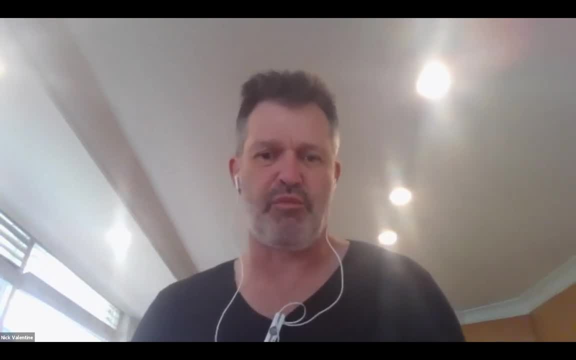 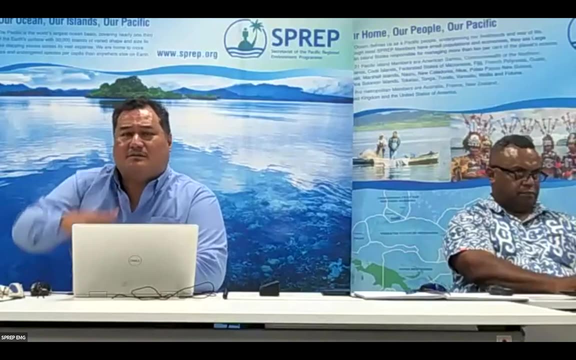 The nature of EAA. it's going to be imperfect and we respond as best we can Over. Thank you All right, let's continue with our presentation. There's a few comments, but I think we're pressed for time. 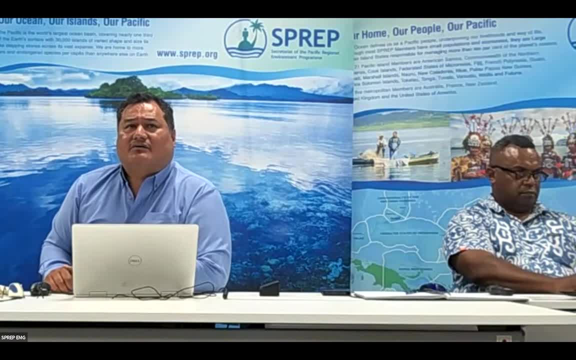 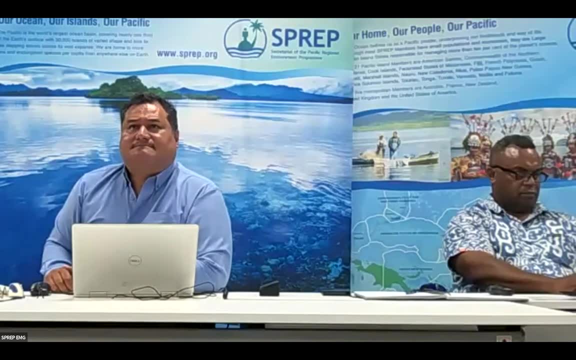 Over to you. Back to you, Greg, please, if you can take us through. Greg, you're on mute. Greg, you're on mute buddy. Sorry, I'm just scrolling through. Are there any actual new comments? I'm just looking. 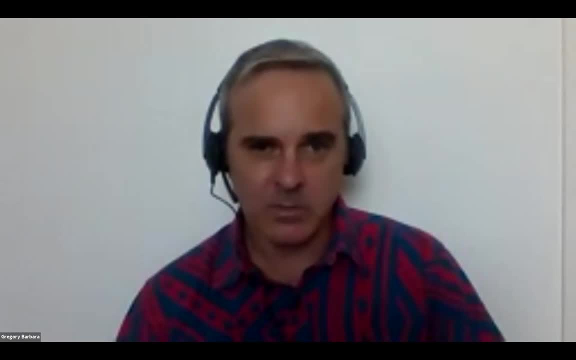 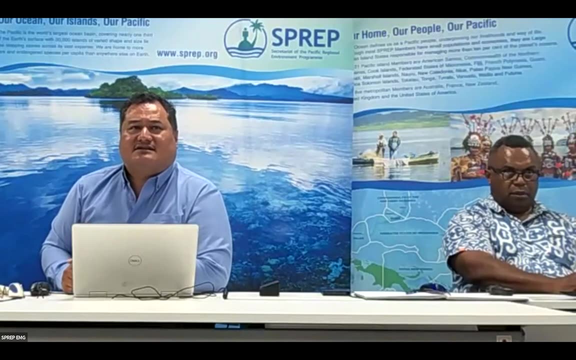 There's the one from Nick to everyone. What have we got? No, I'm pressed for time. If it's all right with you, you can just continue on your slides and then we'll come back and pick on that- The slides. I think Joppa actually wrapped up the slides. 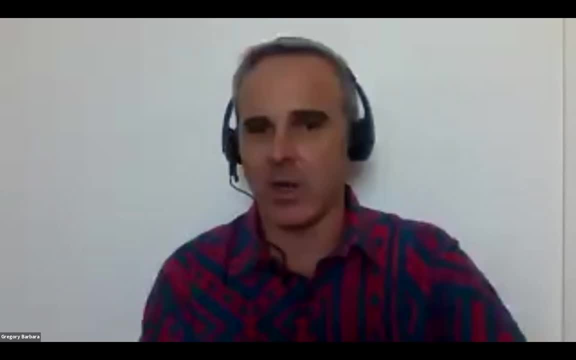 So, yeah, the slides were just really to cover early on and then to launch into the Talanoa, So I was anticipating- I don't know if Gene's online- She was going to be talking about some case studies, but if you're not, I'm really glad that Nick's here instead. 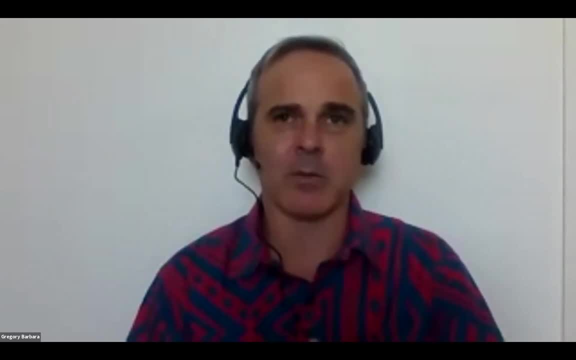 so we can hear about the World Bank projects and our experiences. Excellent example, by the way, Nick, with regards to the chance fines. And yeah, it's, I mean other parts of the world, in Europe and always in Rome. 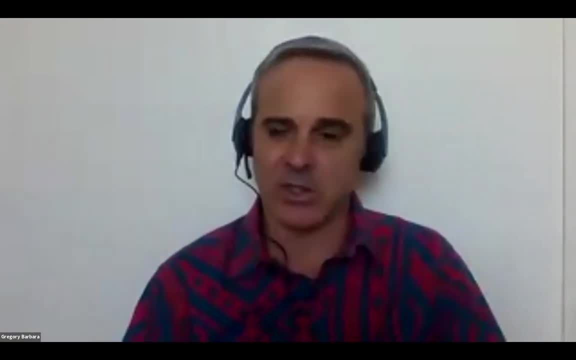 it's basically a standard procedure. You know you're going to hit something when you're digging through the ground, So yeah, they stopped. Yeah, They stopped works, They photograph, They document everything It gets. 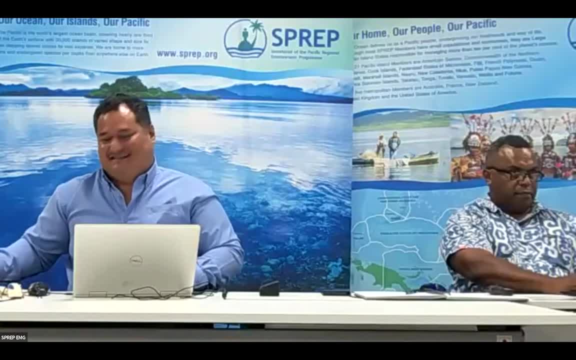 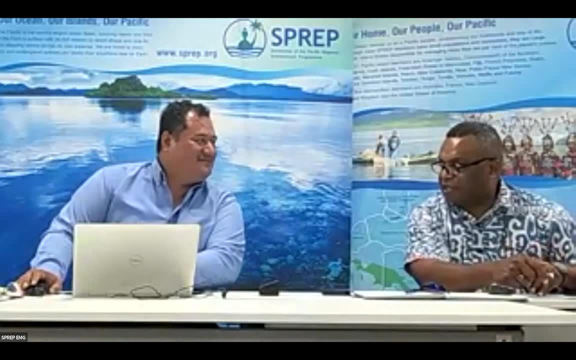 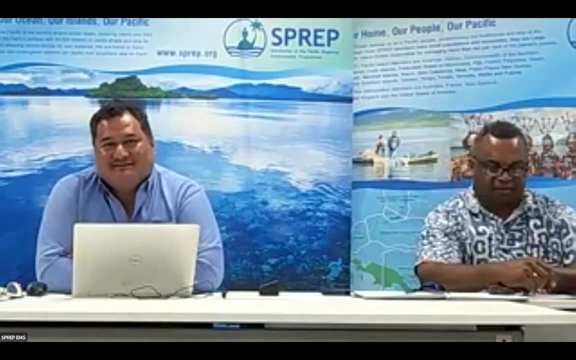 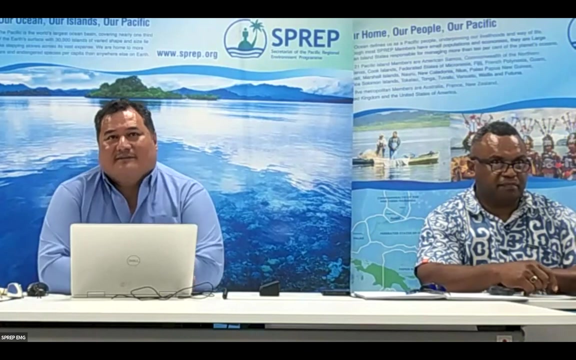 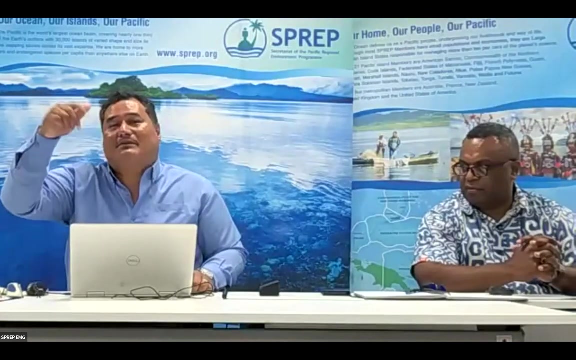 Yeah, and things like that. Thanks, Greg, Listen, my apologies. We're experiencing some technical sort of audio issues from Greg. 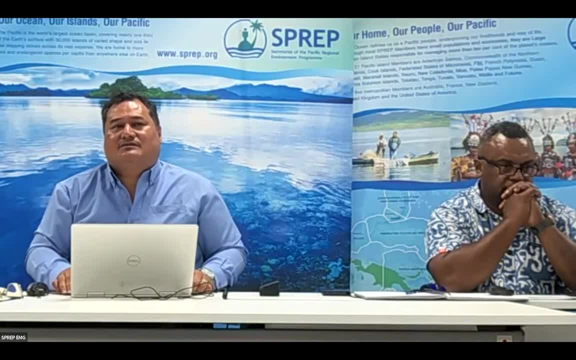 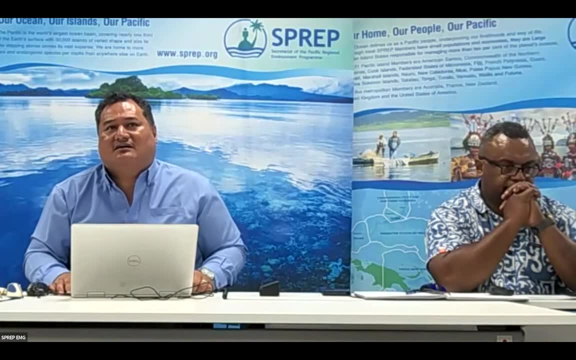 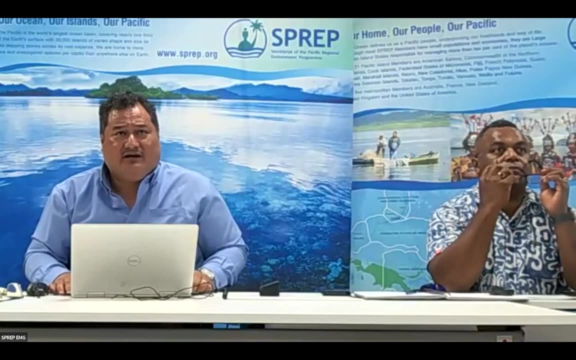 Greg is in a hotel in Brisbane linking in, so perhaps that's where the connectivity issue is. But you know we can make out what he's saying. so thanks a lot, Dr Greg. dr greg, let's go on to the next uh question by now may toward: how can a regulator ensure that? 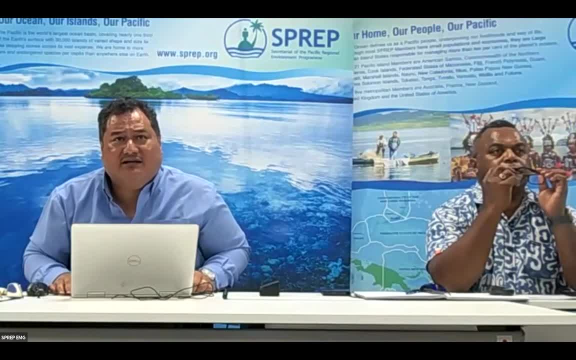 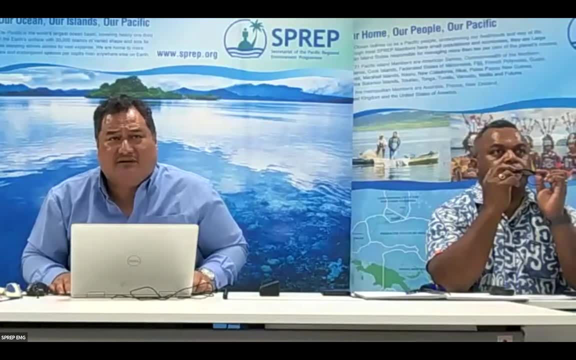 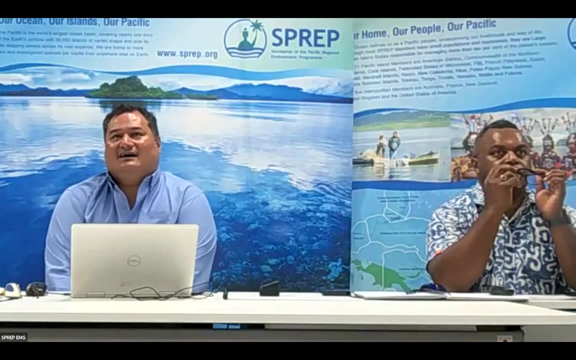 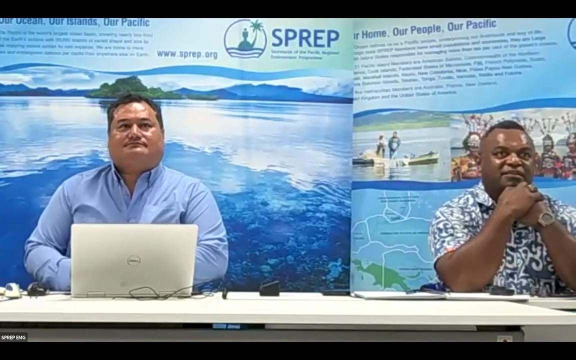 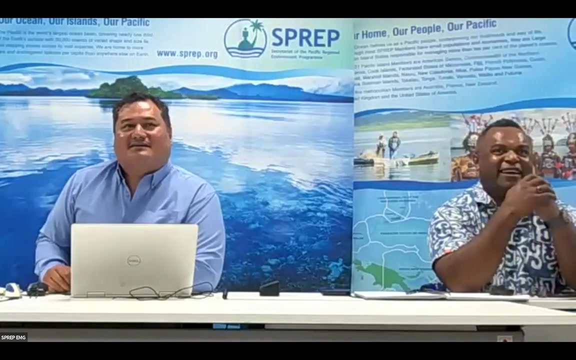 the environmental monitoring management committee is always ready and available and will actively participate in a meeting on a particular development if the committee is not catered for under the environment act. uh, good question. um, any takers have any thoughts on that? all right, we've got. uh hi, uh nick. thanks, uh, uh nicks. uh can jump. 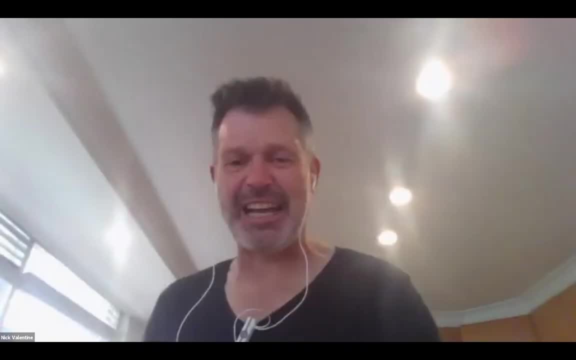 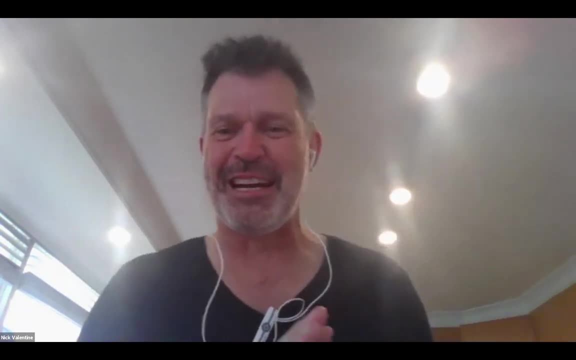 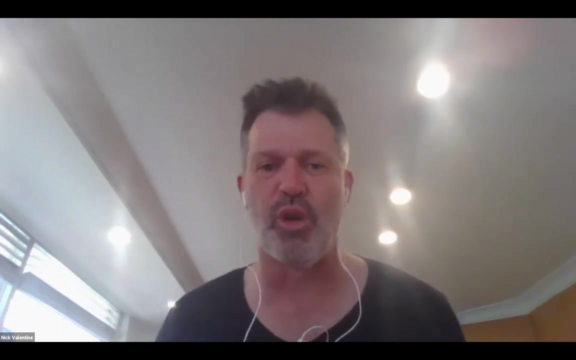 can jump in now. hello, i was gonna say, um, provide catering, provide, provide some morning tea, and maybe the committee members will come, i think, yeah, look, i think it's uh, it's uh making sure that there's resources available and time available. um, if they're on the committee, um, that's a condition of their 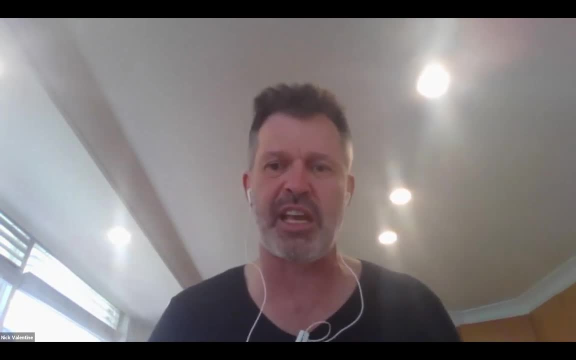 participation on the committee, that they have time available and perhaps there's a, a stipend or something for them to participate. i mean, i, i, i think that's, uh, that's the way to go about it when you establish a committee to make the, to set those ground rules rather than have the expectation. 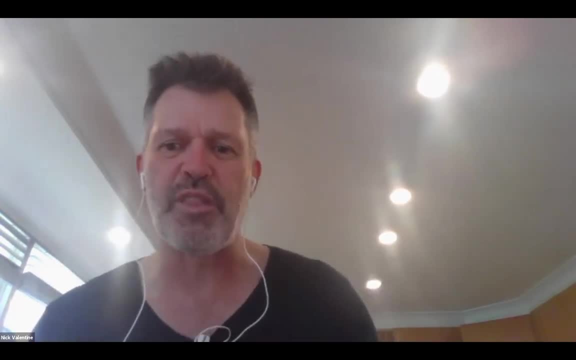 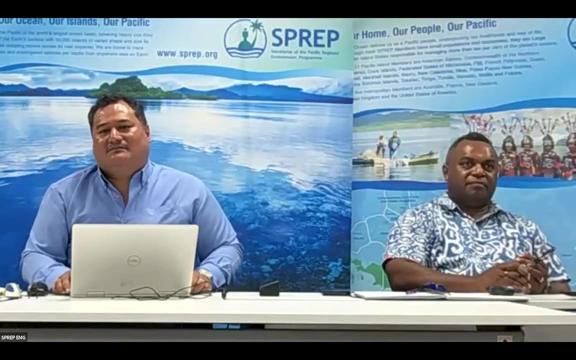 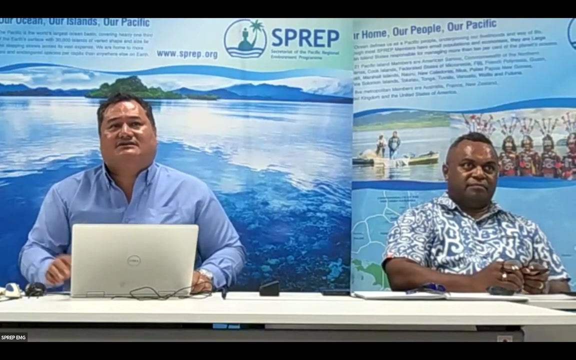 down the track because everyone's busy, right, so not sure if that's helpful. their morning tea is always helpful, listen, uh, you know, it's um, every, every department had their own way of unique way of doing things. uh, it varies across the region, but um, i i think the answer would be, first of all, the commitment. 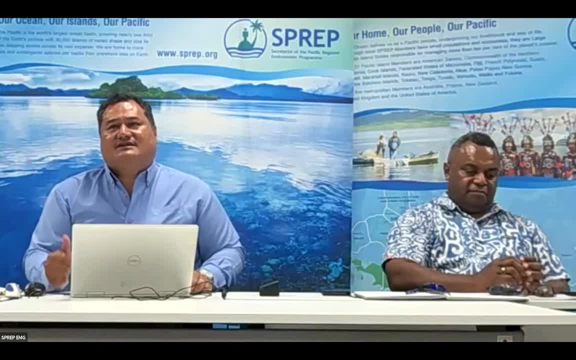 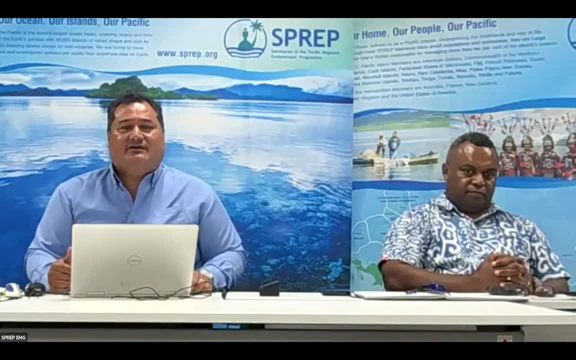 inside the department is there. number two is that there's resources for the committee to support the committee's work. uh, some of these things like uh secretariat or paperwork support. secondly, planning uh ensuring that uh, you know uh the meeting, the committee is regularly meeting on a scheduled. 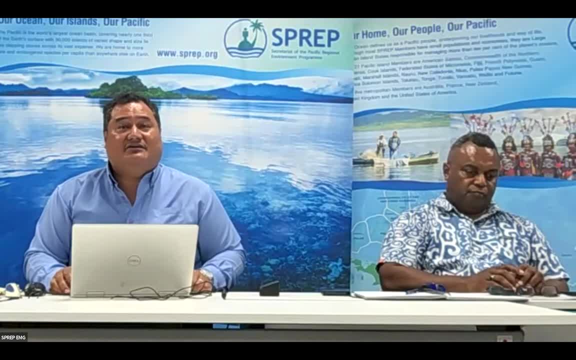 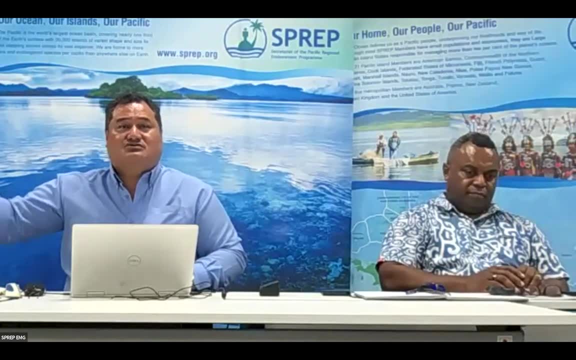 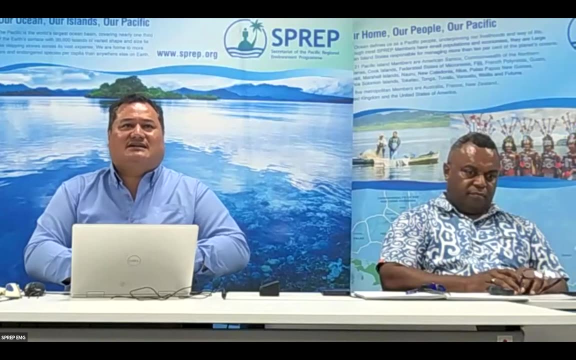 uh time frame so that people can plan in their time, and this is particularly true if, if you're requesting staff from other ministries, uh, to join you. so it's really uh, it's really about. it's really a planning and a commitment, sort of uh a question, isn't it? um, unfortunately it also you know. 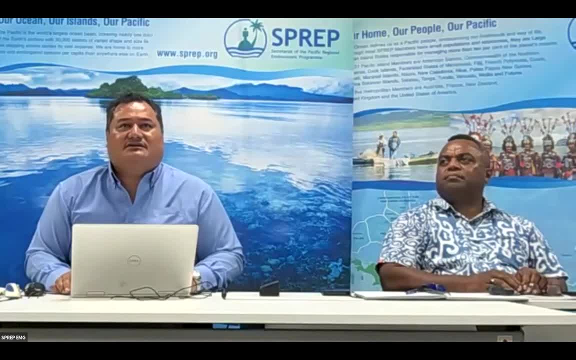 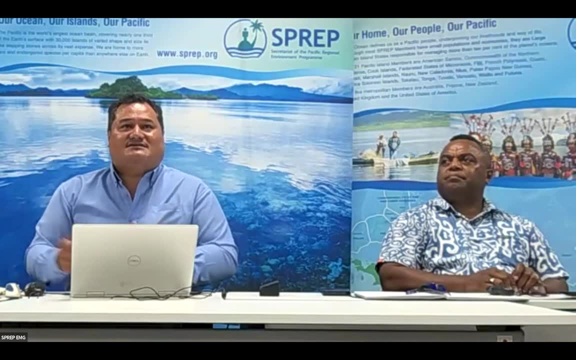 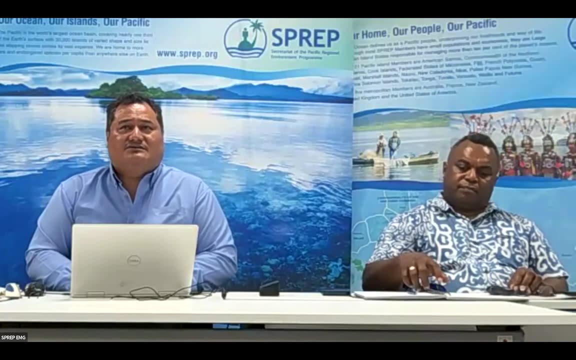 countries. they're the, the, the committees are actually uh are included in a policy or or in the regulation or law, which means that it should take place um more regularly. but that is really at the discretion of the ei regulator um uh to do that. so, um, if i may please uh. thank you, mr. 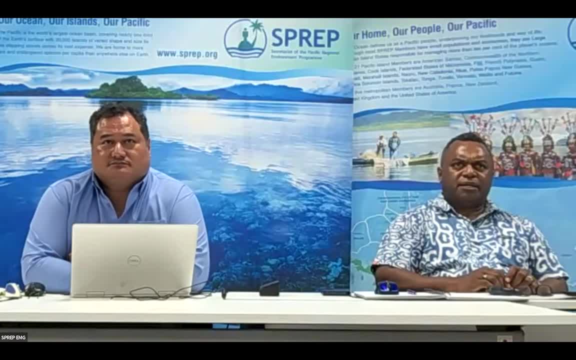 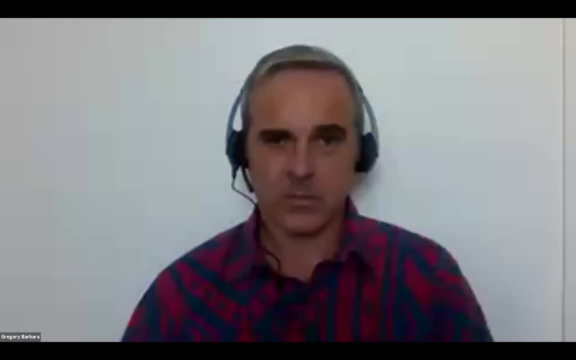 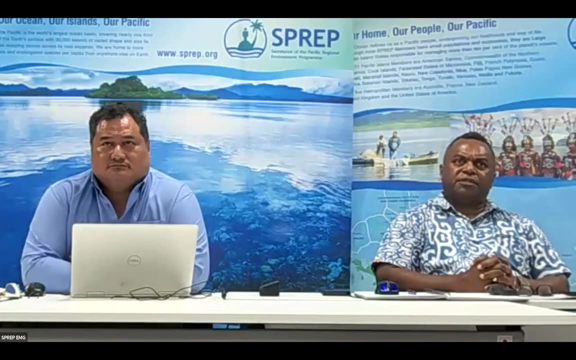 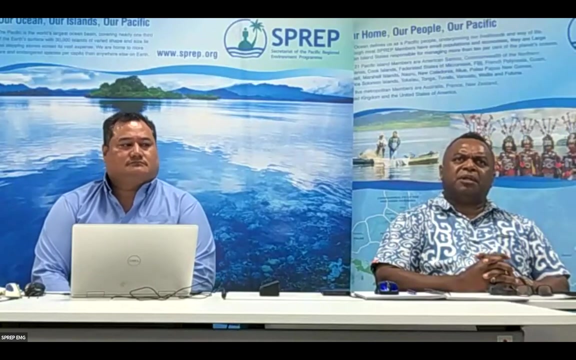 moderator and uh, yes, that is again an excellent uh question by uh, by neomai. i am i normal to you, ma'am? and uh, yes, excellent question, excellent question. uh, well, i'll refer back to my experience and, as stated by the moderator, putting it as a condition is something that i i always apply. and then 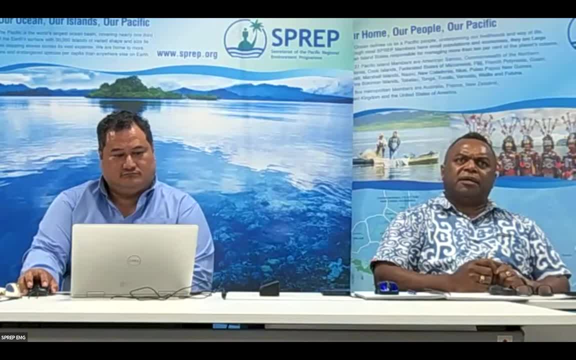 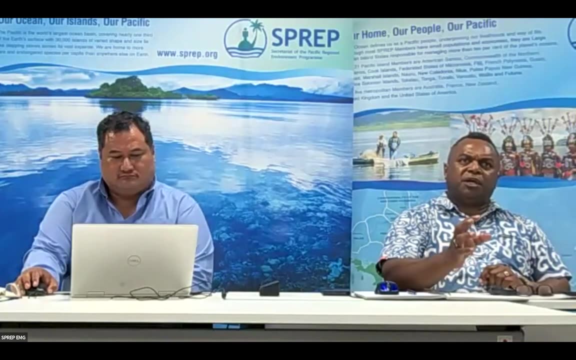 um growing up in terms of reference and uh selecting the, the chair, the chair of the committee and, once that is formed, and the regulator, always remind the chair that we are to meet on this so-and-so day so that we can review and vet some of the the necessary uh issue. or 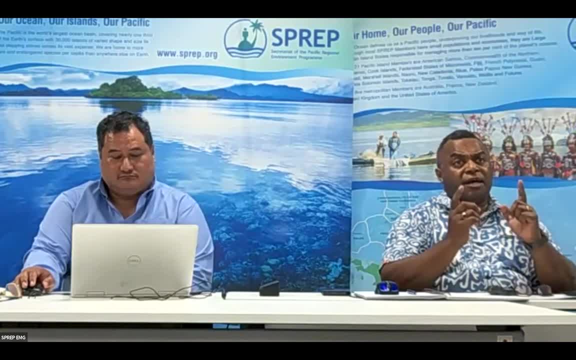 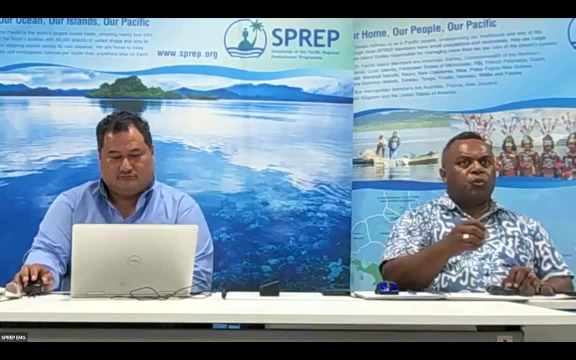 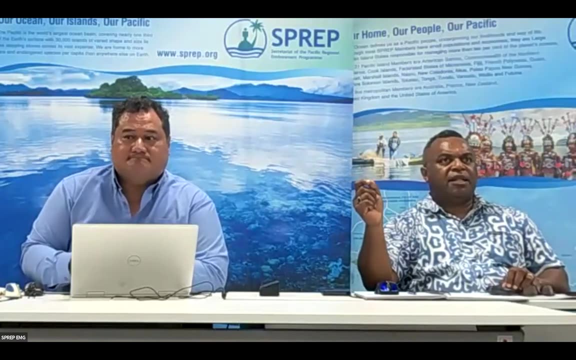 error that may be addressed under the environment management plan. and one thing i noticed: why is it working? well, because if a particular agency is uh slow in the that response and that will develop the delay, the delay in the particular project that take, for example, if it is a government. 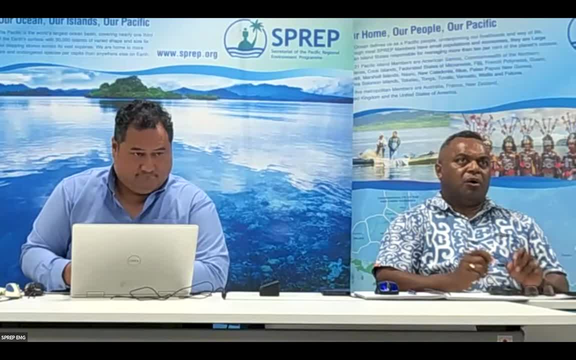 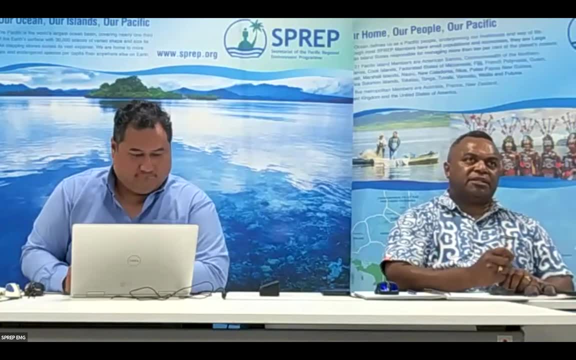 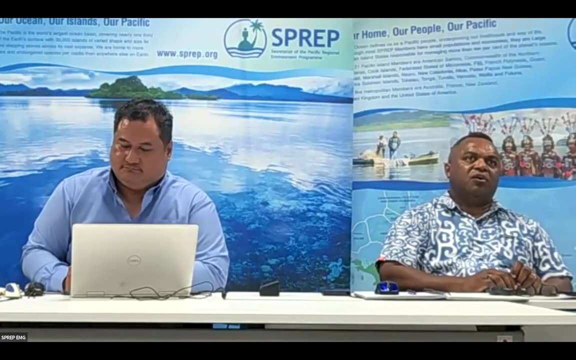 project if it is a government initiated project. so all the committee members must be stand by and on alert to come and meet and address certain issues that needs to be addressed by the monitoring committee. it's placed as a condition of approval. uh, that is one, uh, one area that i can share with you, norma. 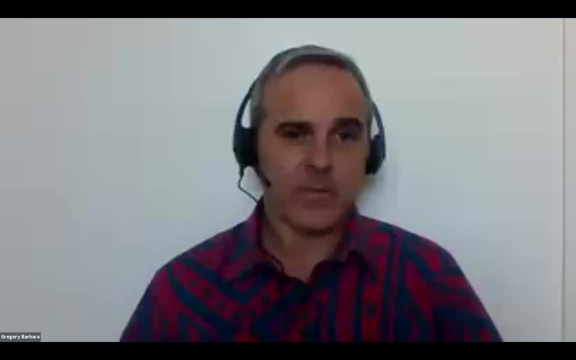 thank you, yes, craig, that's correct. everyone um thanks, norma ex. excellent question, as as the other um panelists have all said. um just thinking, and i know you're talking about- if it's not mandated or if it's not legislated under the environment act in your own country. um what i 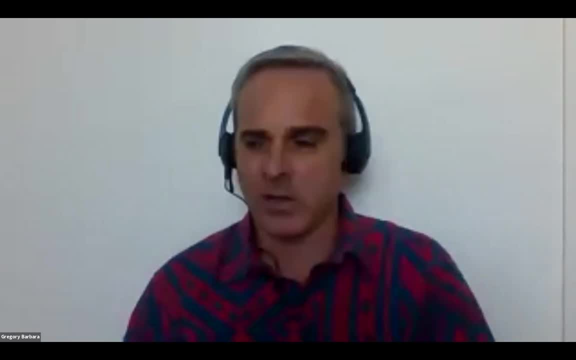 know we we've done with tuvalu. they they upgraded their um, their regulations for eia, and in there they put a provision for activating what they called a task force- a task force or committee um, and we helped them develop up a number of template letters which they issued to the 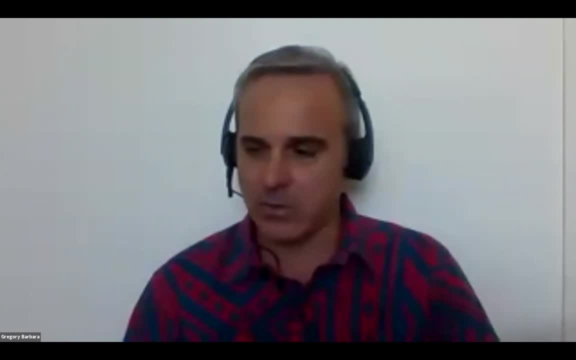 different ministries, to the um, to the uh. well, yeah, to the different ministries to activate and request their participation in those committees. so you could do a similar thing where you have a template letter that you send off to the ministries to say you're going to create this advisory committee and that you're going to need their officers participation. 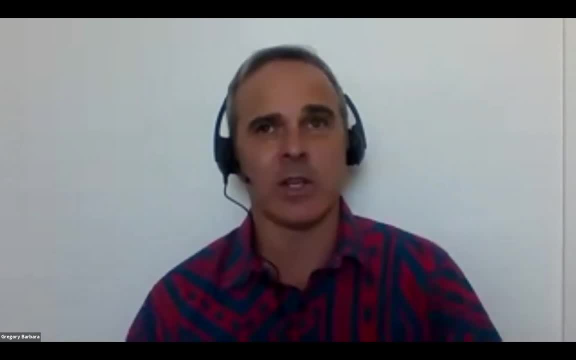 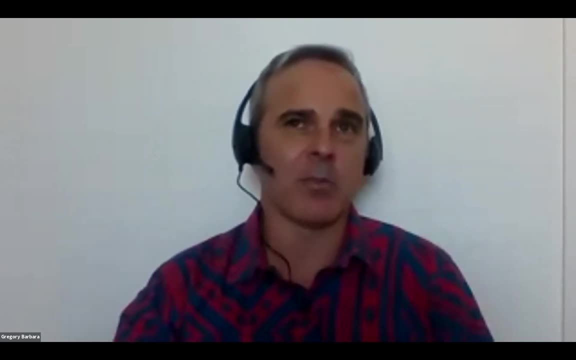 and that could form part of your planning and agreement when you're you're undertaking the eia and review um, just so that everybody knows that what's going to happen, and then you can then start the planning and scheduling um and at least advise them that you were going to call upon their 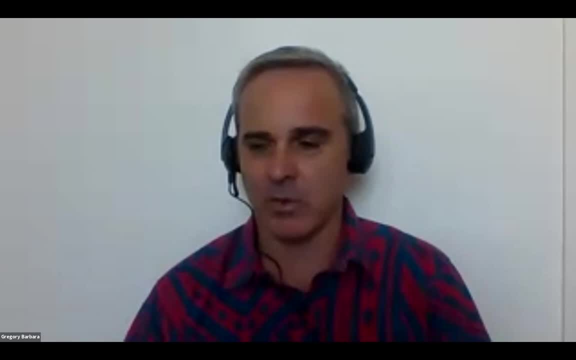 services throughout that process. yeah, yeah, i think, i think i think that's a really great point, um, i think that's a really great point, um, and, and i think that's a really good point. and i think that's a really good point because, you know, most ministries come in sort of out of the blue to them because, as we all know, everybody, 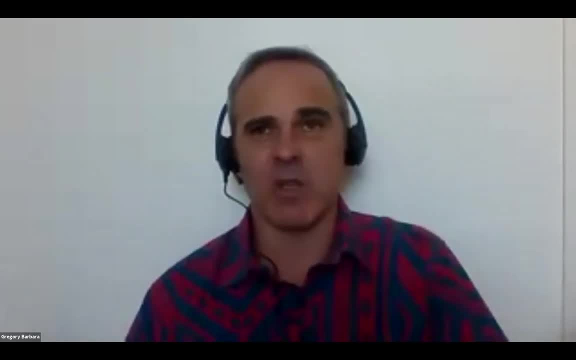 in government has usually spinning multiple plates, doing lots of different projects and lots of different roles. you know you're an environmental um officer. normally you know how many different things you're doing, so, um, when you're dealing with the other ministries, it's just: yeah, maybe have a plan in place, request a formal letter to their supervisor. 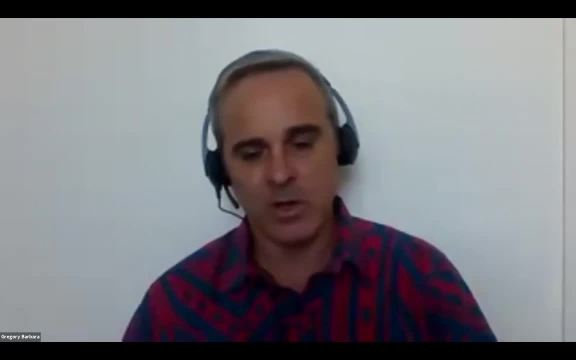 chain, get, get your superior, get your director to issue it. so there's a formal, formal line of communication and the committee gets set up. even if there isn't legislation, at least you can get an agreement going between the agencies. did everybody hear that, or did i drop audio again? 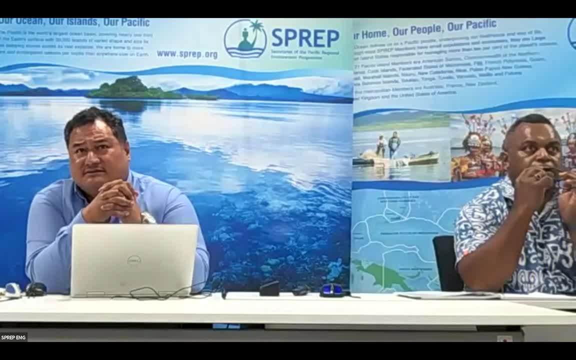 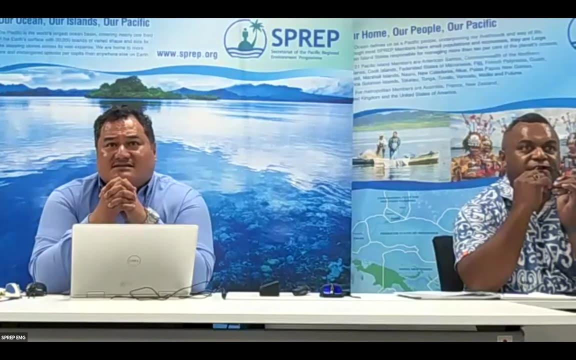 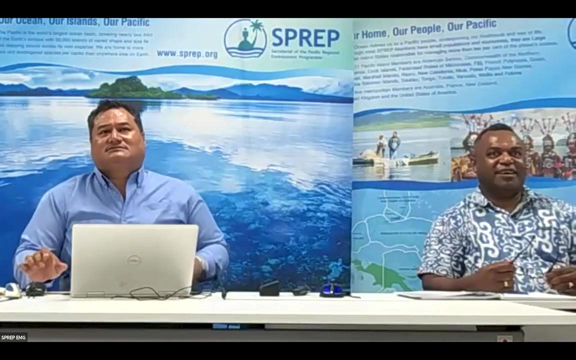 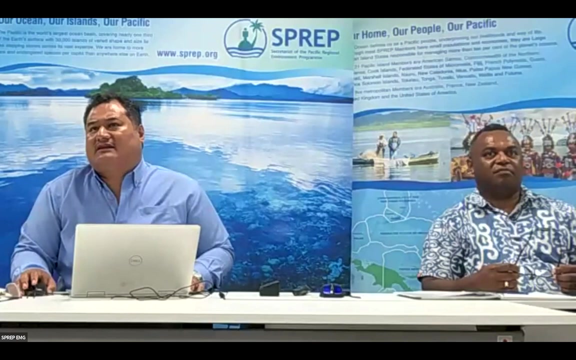 no, that's good. do we have any other questions popping in? we've got a, i think. okay, now me and the door. i mean yes, yes, do you have a question? be good, i mean, i see, that's. uh, that came online. no, okay, got a final comment from nick. i think now may undertone. 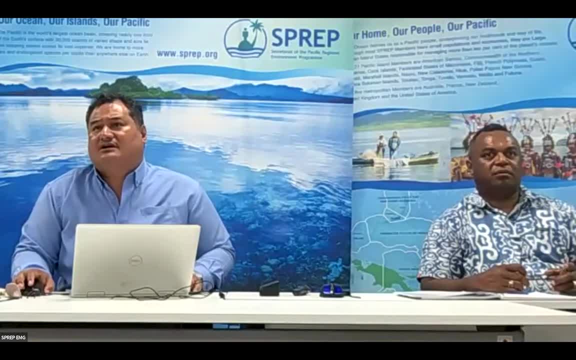 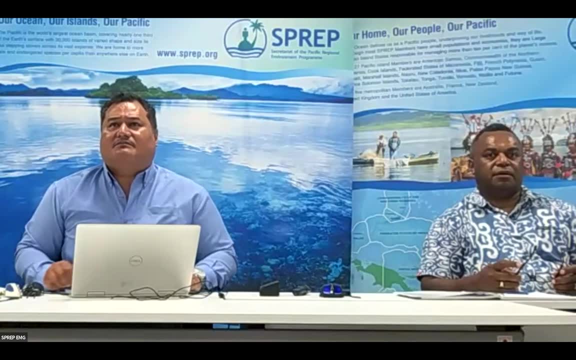 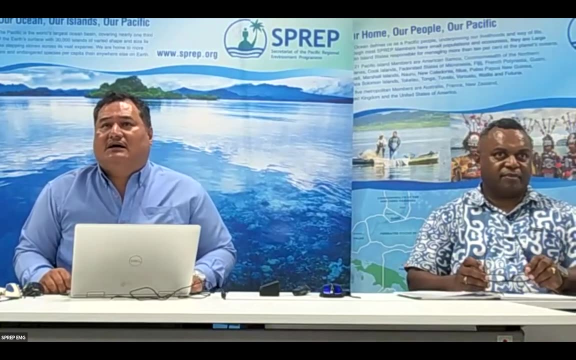 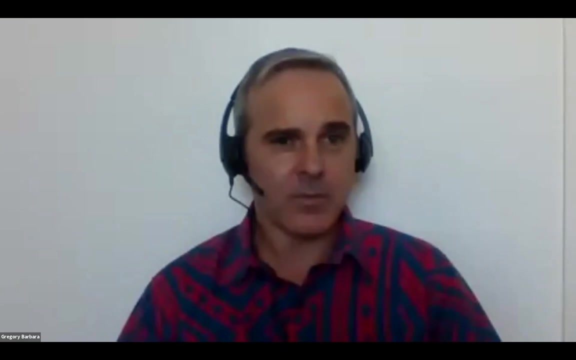 finance projects. we, or you, should ensure adequate budget and resources in the pmu and, okay, in a design and supervision console. uh, thank you very much, nick, for that. um, uh, final uh call for uh any questions? uh, before we wrap up, um, if it's just, mr moderator, break here, yeah, go ahead, all right. um, apologies, i don't think we've got a lot of questions. 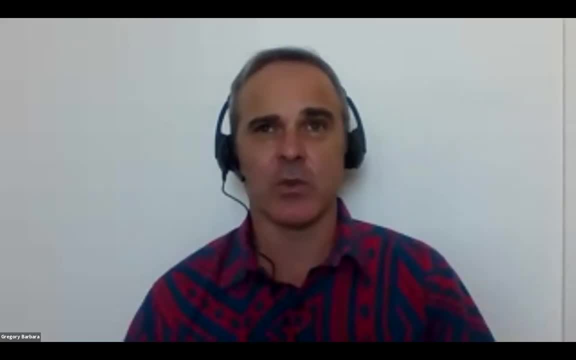 i think we probably really got into one of the other objectives of this, which was talking about selecting appropriate consultants. um, maybe nick can can chime in here if he's still on, if he's still listening. um, there are processes within the donor banks for selecting the correct type. 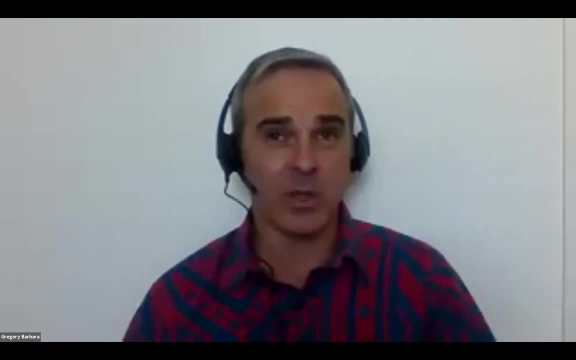 of consultant for your project. but, just like with scoping, understanding which studies need to be undertaken, you need to identify the appropriate consultant for the types of work you're going to be doing. so, um, i know, within the pacific, we have a limited pool of consultants in many countries and we have 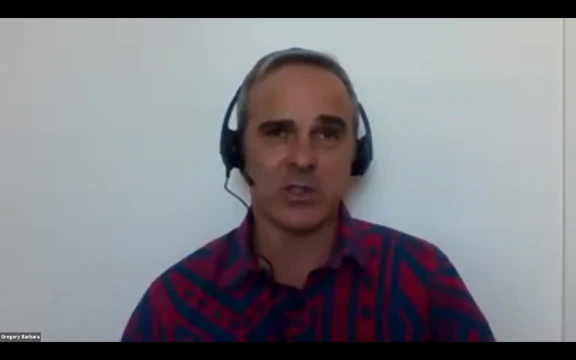 seen as a result of that that we've getting biologists writing up geotech reports, um, or geologists doing social engagement. this, under normal circumstances, is not really appropriate. so, um, when selecting your consultants, it's really important to try and look for the people with the right skill sets, the right qualifications, the right skills, the right skills, the right skills, the. 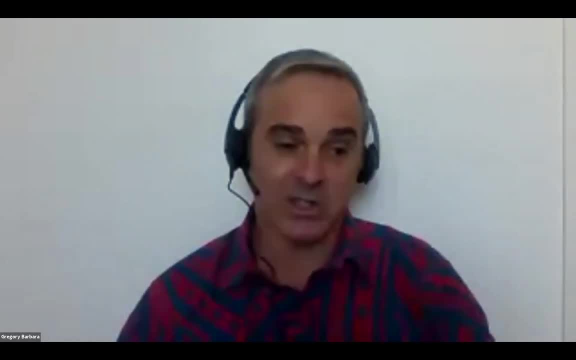 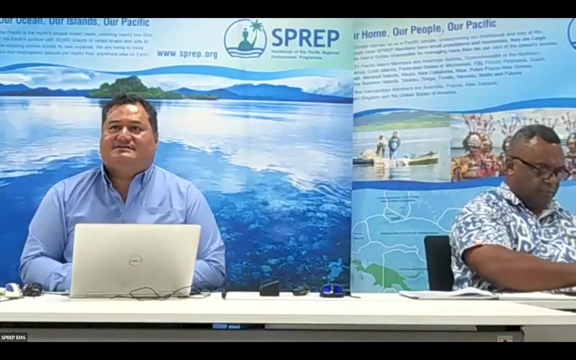 right qualifications to undertake the specific specialist studies, because, ultimately, you're relying on their advice to um to do a good eia and to provide you with the appropriate mitigation measures. yeah, so just to from from my side, you know it's uh, you know when you're, when you're um. 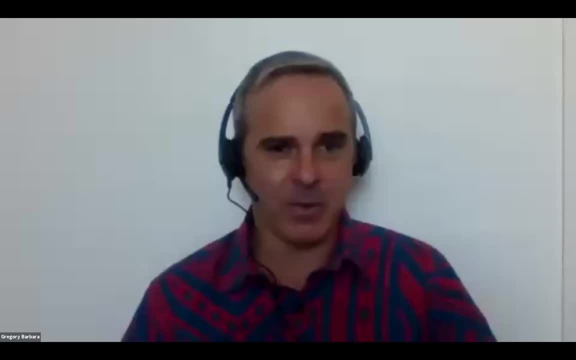 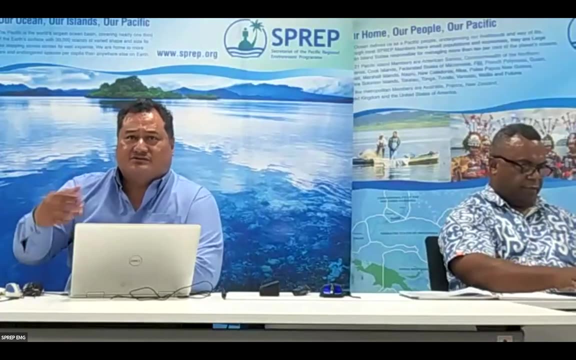 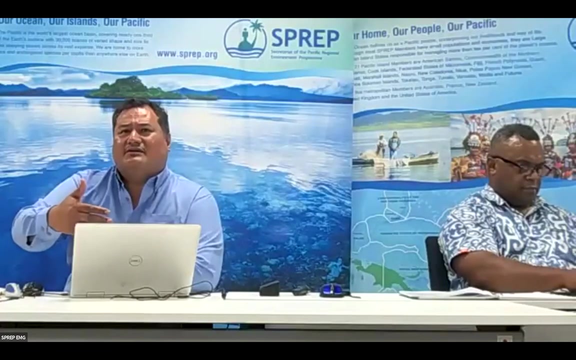 that's why it's very good to develop my mic, because i'm getting feedback. so you know, the idea we've been talking about is how to prepare a responsible terms of reference. so the word is responsible. what exactly does that mean? it means that whatever project, uh application, can we have someone? 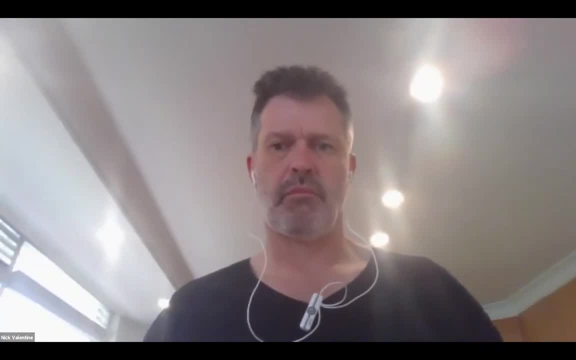 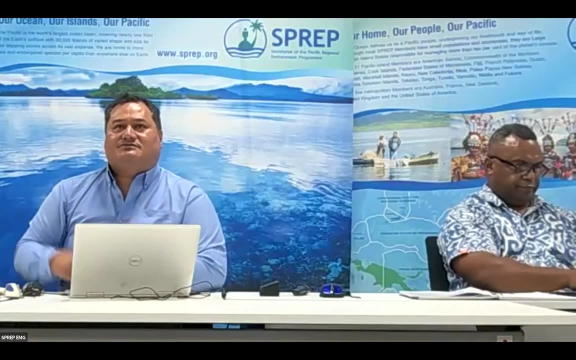 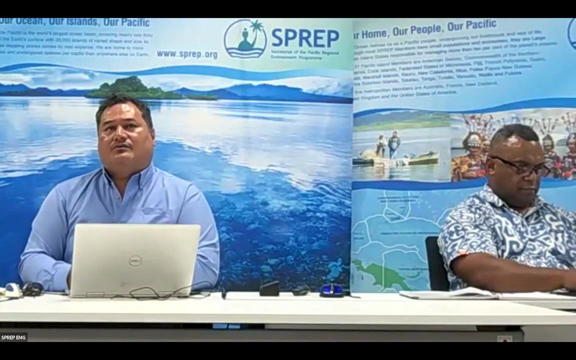 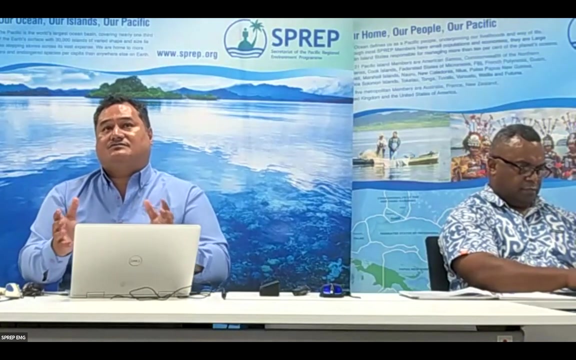 can you mute? oh, thank you, thanks. so once, once you've developed a responsible terms of reference, it should, you should be able to identify the key areas of expertise that are required to prepare the eia report. so that's why we there is that insistence um for for a proper multi-disciplinary team to sort of convene. 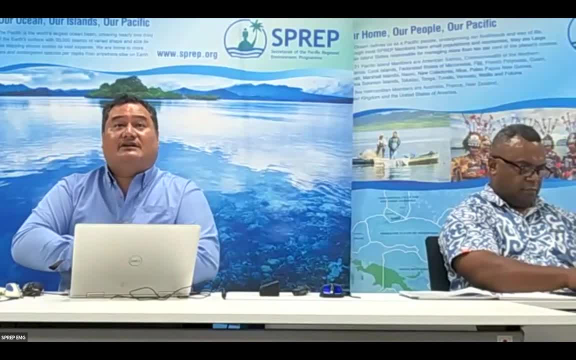 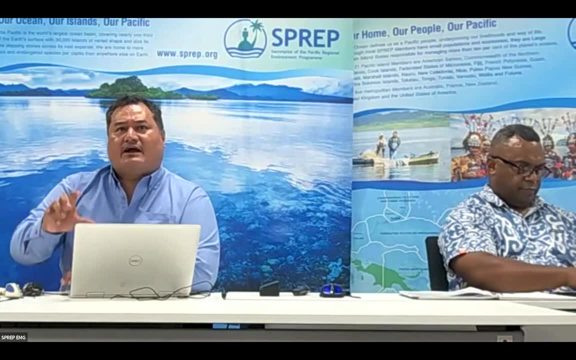 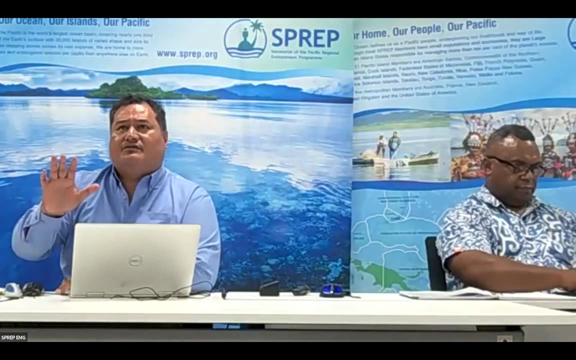 and discuss what sort of areas that should be included in in terms of reference and because that you know, and then the developer will be able to identify their team or the right set of consultants. uh, to do the the job, like, like greg said, if you got, if you got, if you, if you receive. 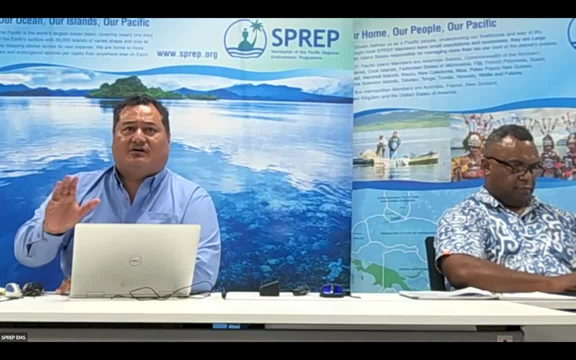 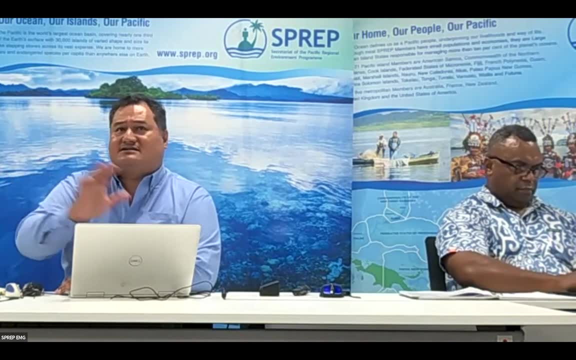 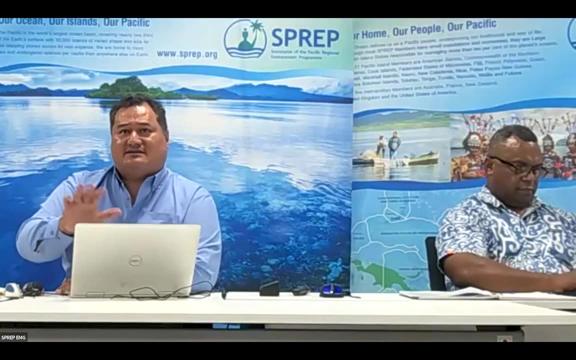 a, an eia report, you must insist on the correct credentials. that report should highlight the credentials of those who prepare the report Or, even before that, discuss it in the beginning with the developer who is hiring the consultancy firm to ensure that the proper team is in place. 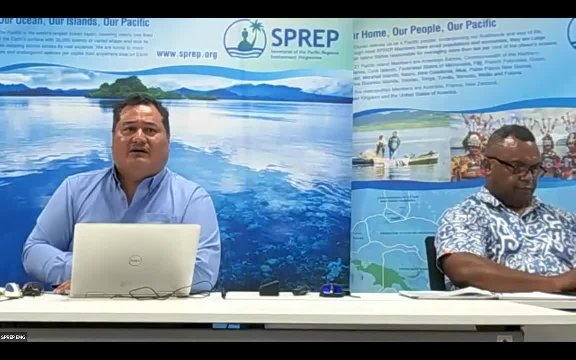 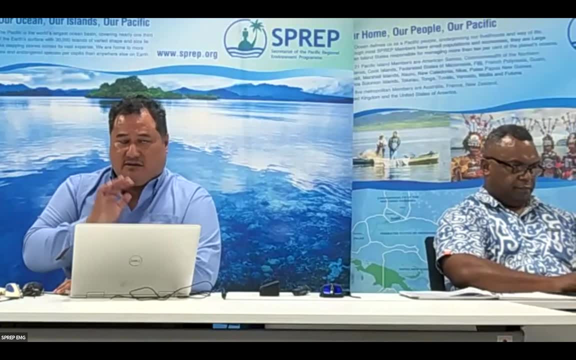 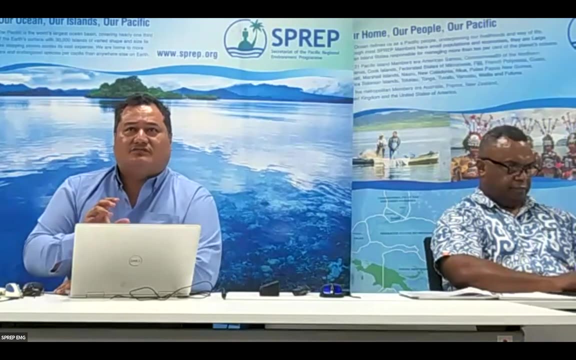 And so that would take care of having the right, suitable and qualified consultants. In many cases- and I agree with Dr Barbaro, in many cases that I've seen, there are consultancy firms with qualifications and experiences that do not match what the terms of reference. 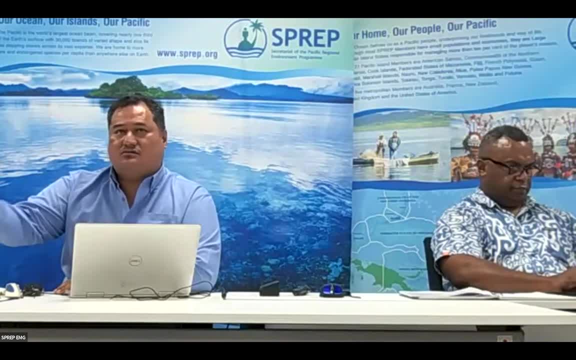 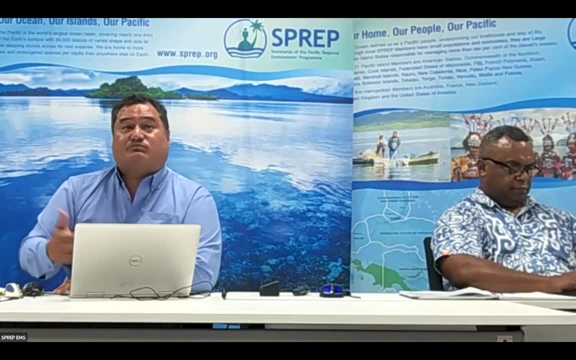 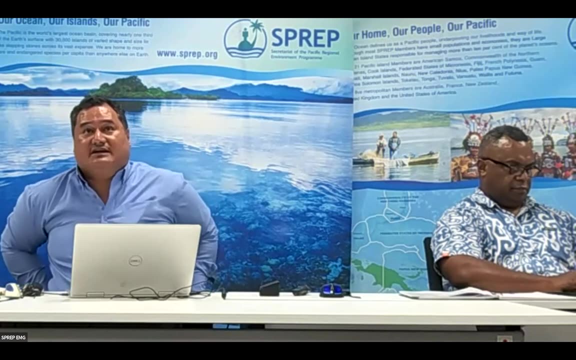 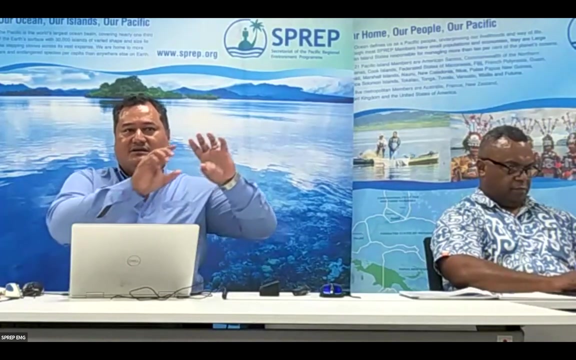 are saying- And that's a clear sign to the regulator or to any other agency- that the report is probably not going to be accurate or reasonable. Responsible is the word that we've been using, So I hope you can understand the connection between putting together in terms of a proper. 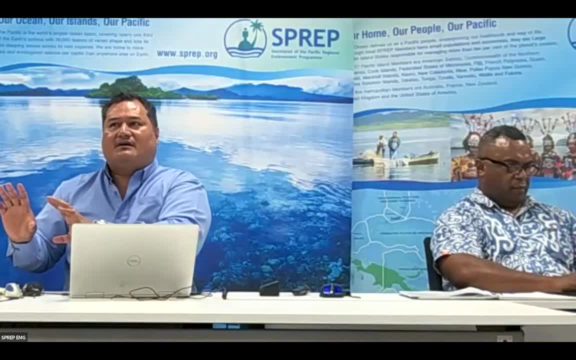 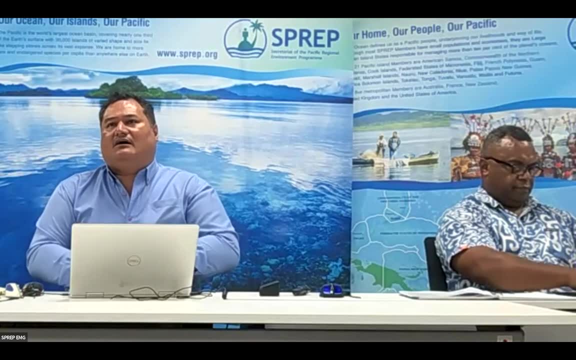 terms of reference, with how it sort of matched the design of the EIA firm, consultancy firm that's going to prepare the EIA report. All right, Do we have any other comments? No, No chats, Man. hello, It's Rachel here. 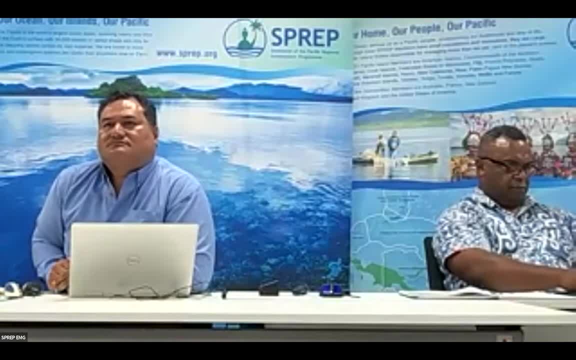 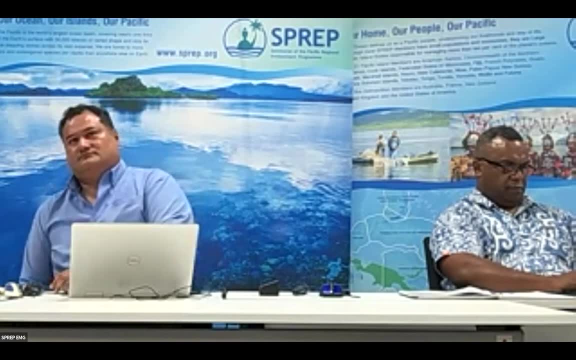 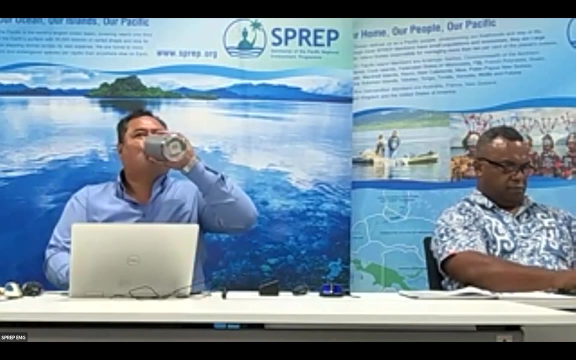 Hi, Rachel, Go ahead, Thank you. Thank you. I think I don't want to make things sound more complicated but, building on what you said, I'd say we are doing more and more complex projects in the Pacific, And I'm particularly talking about donor funded things, but anything in the outer islands. 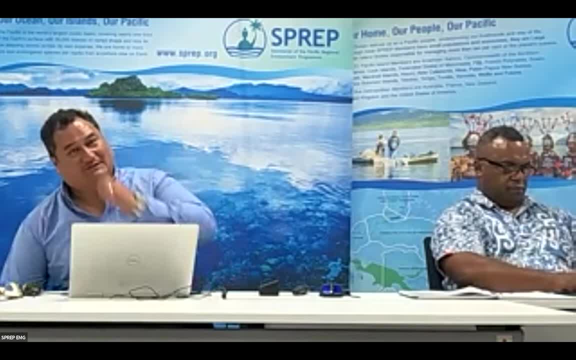 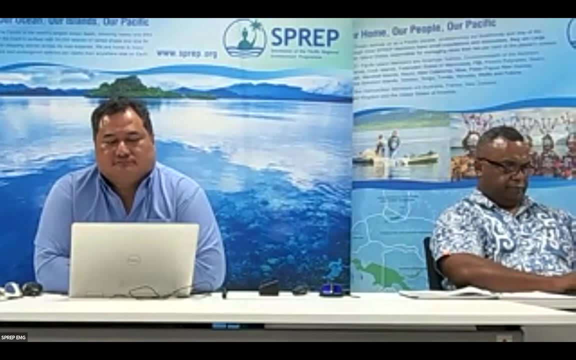 for example, that any of us are doing, it's more complicated than doing things in main islands and the issues will be different, So it's pretty unlikely these days that a single consultant will be able to do that. Yeah, I think that's the key thing. 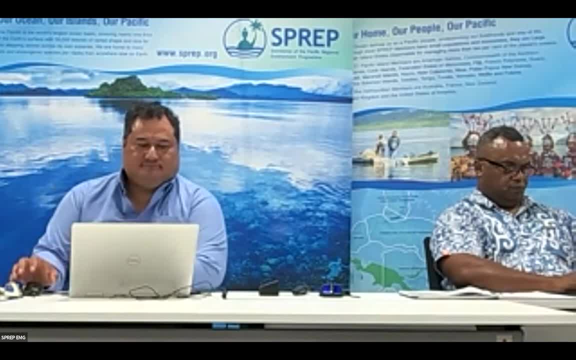 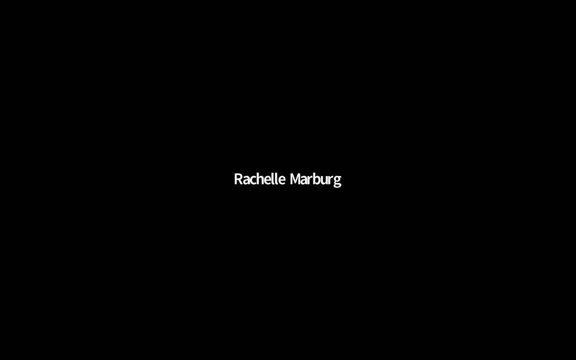 It's not a big deal. I think that a single consultant will be enough because of the kinds of expertise that you know the projects that are ongoing need to be using, And if you appoint multiple individual consultants, please think about how they need to work together. 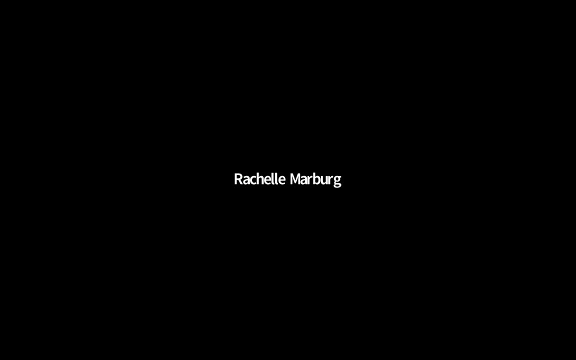 because all of the issues. a classic division, for example, would be the environment and a social consultant, but obviously they have to work together because issues around water or fishing or forestry can easily be environmental issues, easily be environmental issues. they could be health issues, they can be social issues. so the 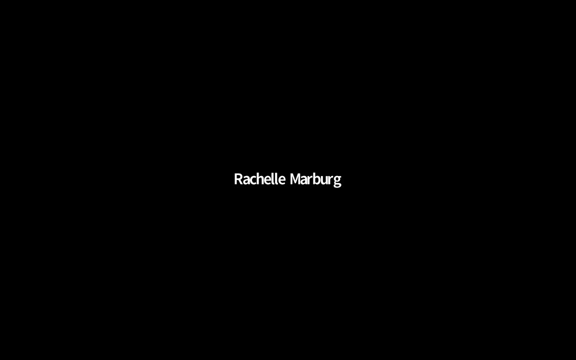 consultants need to be able to work together and it's really important to think about that from the beginning so that you put the right contractual arrangements in place. and this can be complicated and it can take a little bit of thinking, but I'd really urge you to think about that up front. 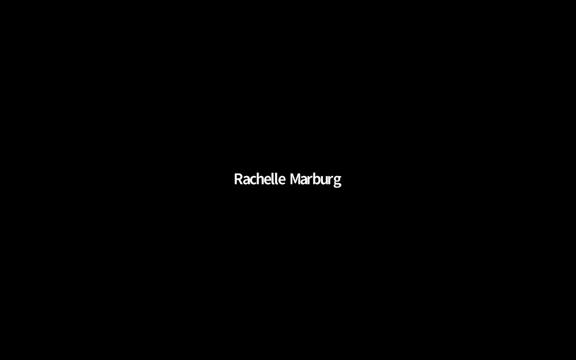 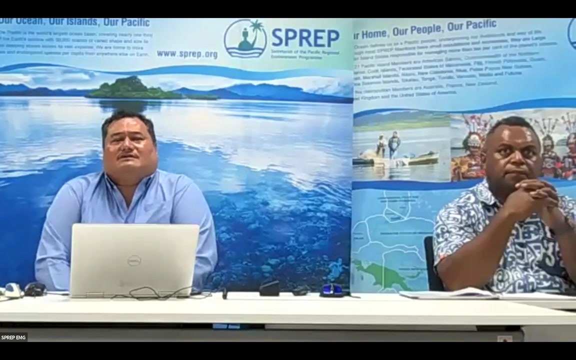 because that will really help you get the good outcomes that you're looking for from the reporting and the preparation process, but also through to delivery, implementation and delivery and and the whole objective- meeting the objectives of your project in the first place, thanks. thank you, Rachel. we've got comments from Amin Yassi from Fiji. it's a precautionary approach if this is. 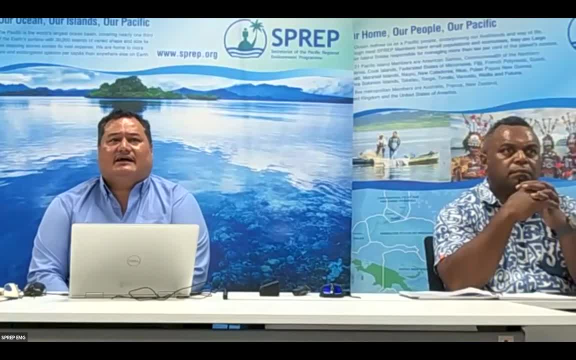 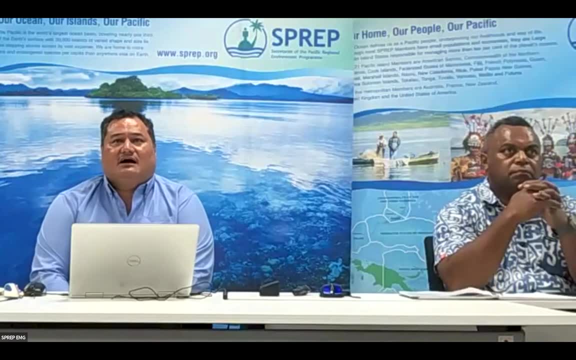 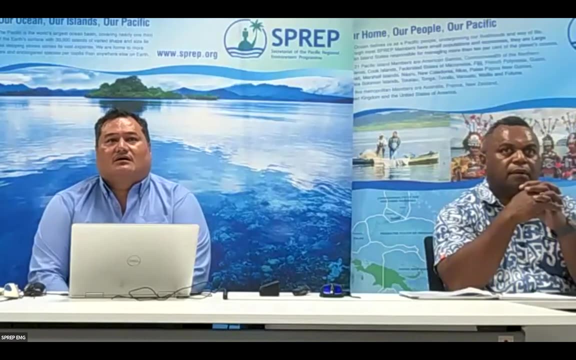 not carefully carried out, this can cause delay and variation to the project. so, okay, that's part of the terms of reference. thank you, Amin Yassi. any other comments? any other comments from the floor? okay, well, I don't see any more chat and I think that's probably. 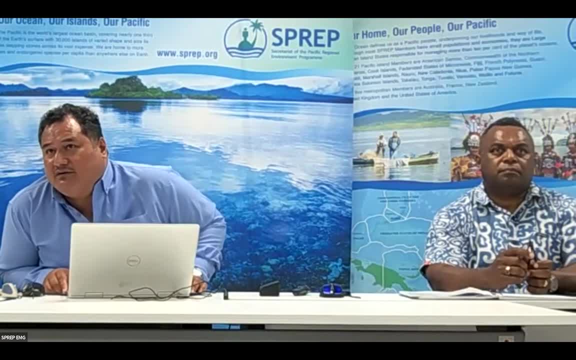 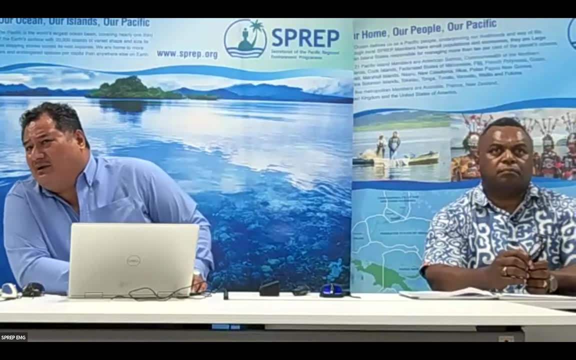 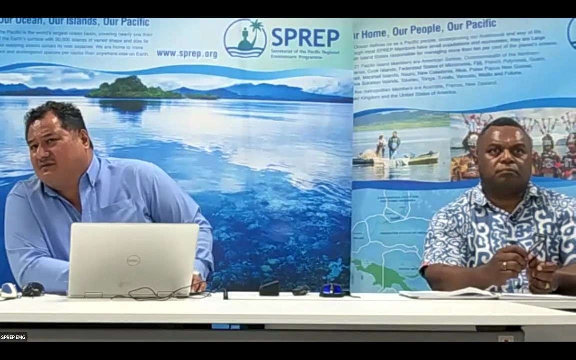 a good sign. oh, we got a question from: what about projects that does not require an EIA but only requires a CEMP or construction environmental management plan? from my experience, get it from Fiji roads authority. the approving authority does not give us in terms of reference for a CEMP or construction environmental management plan, so we, as the proponent, will. 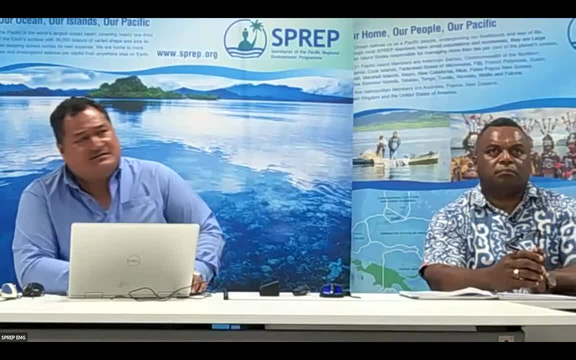 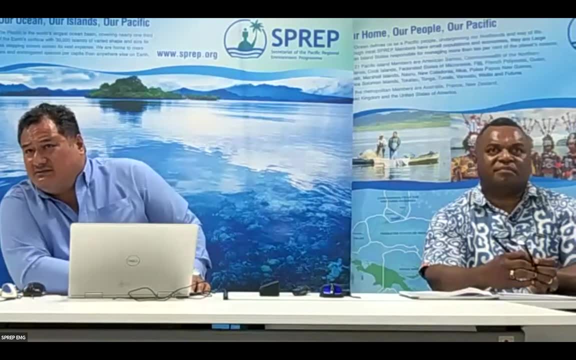 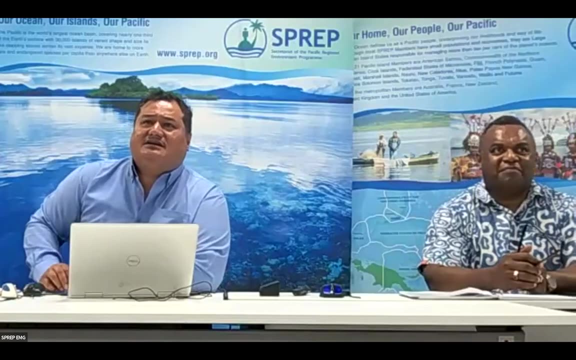 have to formulate our very own CEMP. so this is from Fiji. any takers on that question? do we have any comments from the board members? thank you, thank you, thank you. have anyone from fiji uh, the department of fiji uh, joining in? just uh curious. 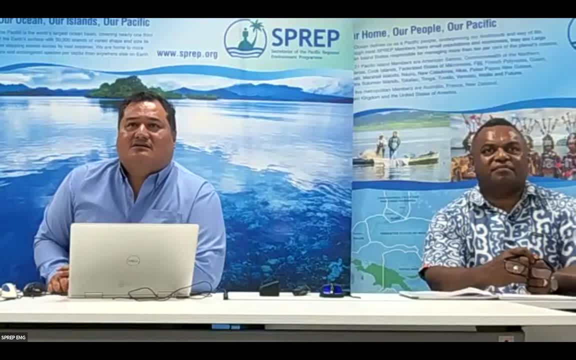 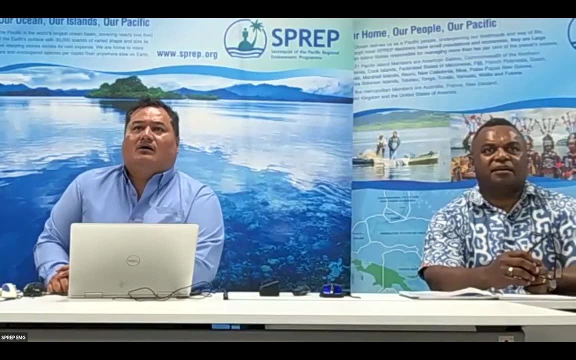 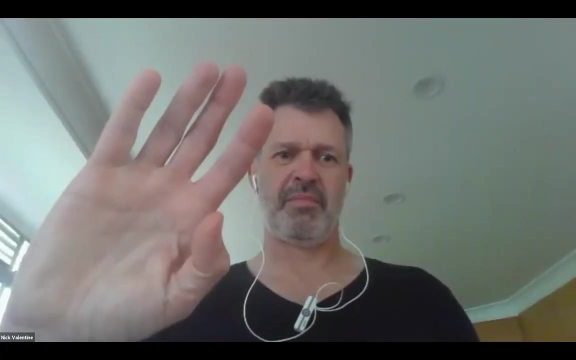 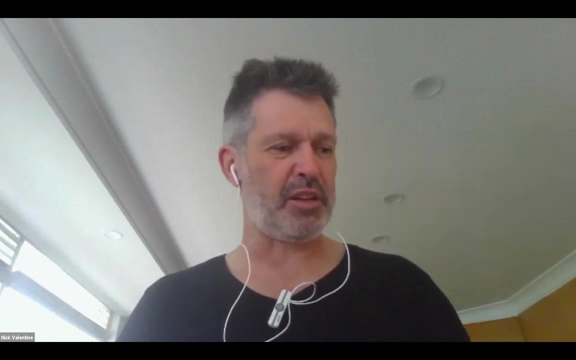 perhaps you can provide us with uh, with an answer, or a response. no, did you say anyone? all right, uh, listen, we got nobody. but from: okay, all right, nick, you go ahead. yeah, look, um, this is uh. this is uh an argument i have internally in the bank, actually. um, 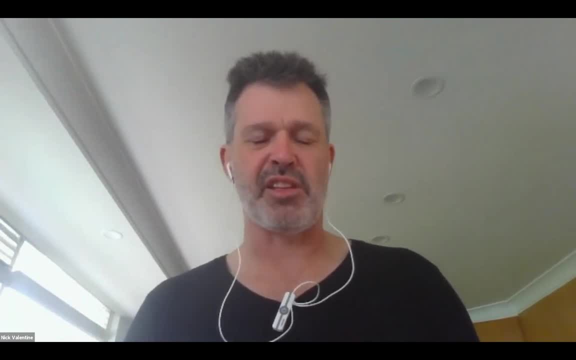 i think any, any project is going to have a potential environmental and social impact needs an assessment. how else do you know? you can write a cemp to manage impacts, but what are the impacts you're trying to manage? so i i don't see logically how you can just have a cmp which is a, just a. 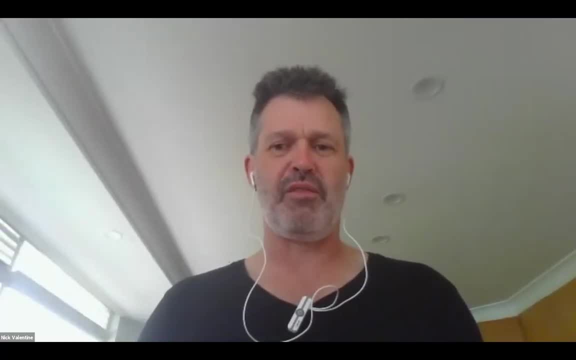 collection of mitigation measures. what do you try to mitigate? so, even if it's just, i think you just take the principles in the in the spread bi guidelines and you expand them and contract them based on the complexity of the project and you and you go back to the principles of screening and 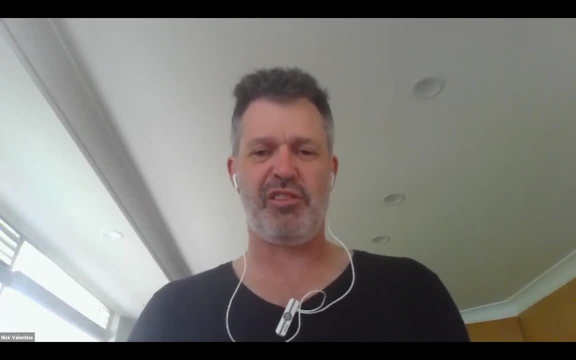 scoping, you say, okay, we've only got a two or three little 20 issues, just as i've done for a very small project in kiribati which is only really installing a bit of cable and and a- uh, a data center. you know it's very small scale, but we're still prepared. 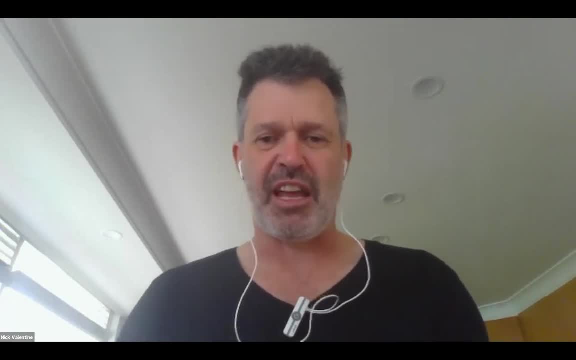 an environmental, social uh impact assessment. it's a. it's just 20 pages rather than 200 pages, so i think if there's civil works, it has to have an environmental assessment of some sort, and that environmental assessment includes a management plan. yeah, so that's that's why i'm going to do that. 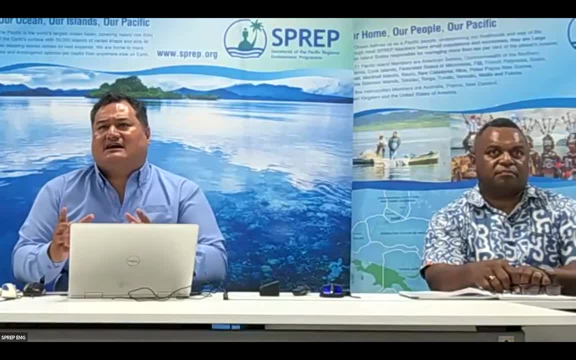 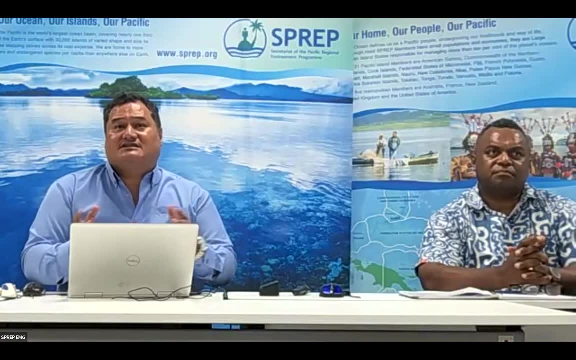 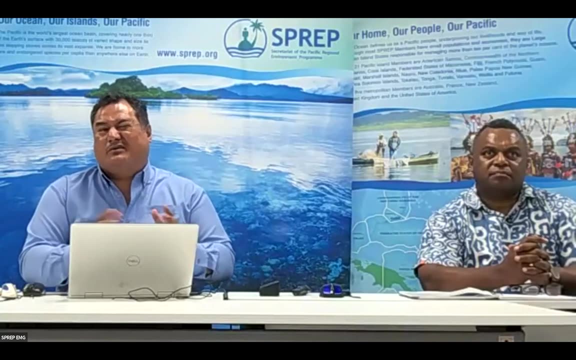 thanks, nick. like i know, in samoa there's two types of eia. just before i hand over, they say: um, it's what they call preliminary environmental assessment report, which is a pair, and then there's a comprehensive environmental impact assessment report, and so the preliminary report. 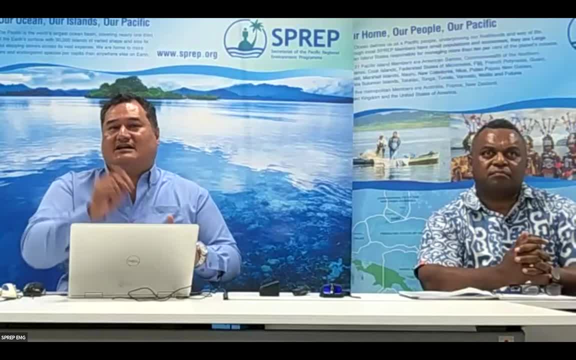 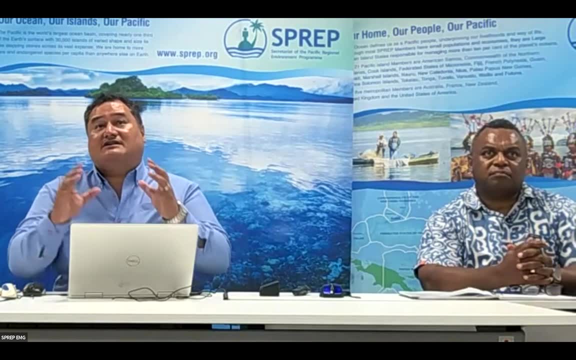 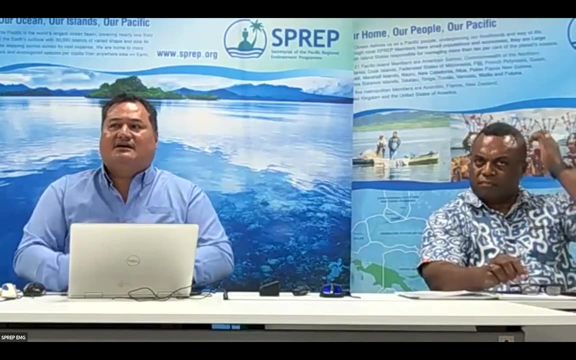 is just sort of more of a screening, going through the screening checklist and see if it's, if there are sort of adverse, identified adverse impacts or just impacts that may not necessarily be adverse or significant, but the, the, the use of the pair is just as a first stage to see, uh, to see what they. 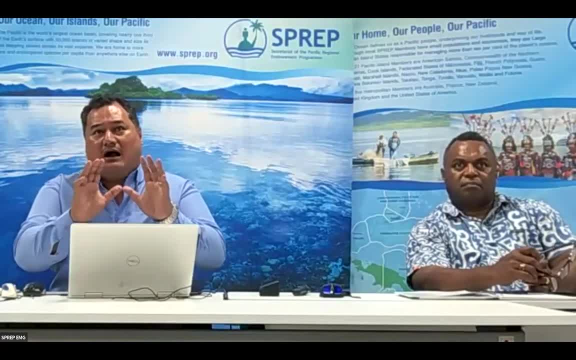 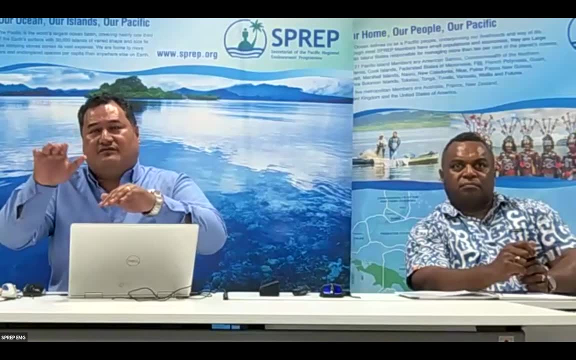 are, and if that is enough, if an eia is not required- because that's what the pair is supposed to conclude, whether an eia, a comprehensive eia, is required or not, if it's not, then they'll just sort of, uh, have a, a, a like this, an emp that's based on those, on those risks that nick alluded to. 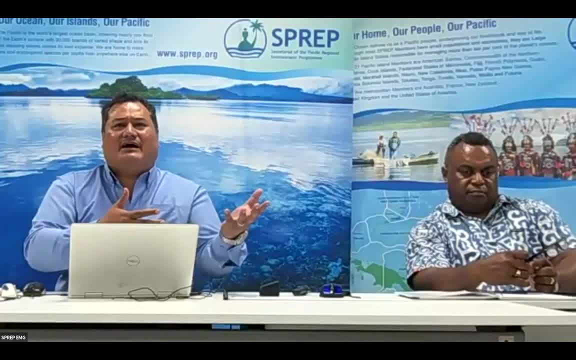 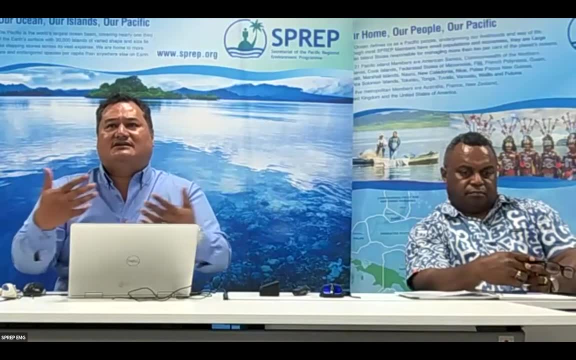 the there. there has to be an assessment of impacts to guide a mitigation plan. you can't just. you know that that is the connection, and if it's not, then then there's a missing piece there. i'll go to that topic, thank you. thank you, nick. thank you, uh. 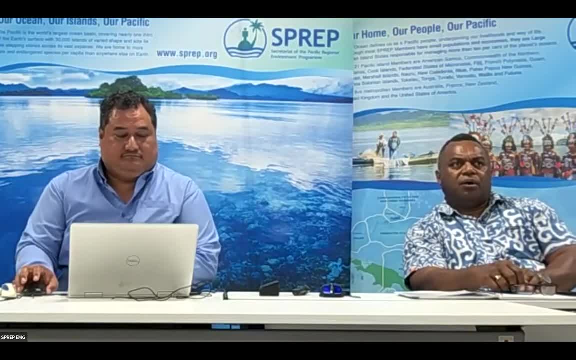 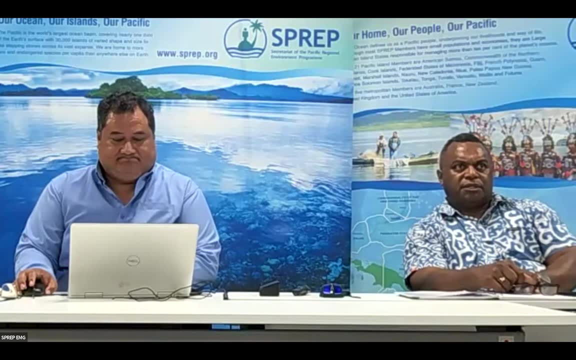 mr moderator, yes, uh, thank you to our colleague kelly from fiji in raising that. and uh, yes, uh, you know the question raised is uh really a valid one. and, um, i agree with you in, in some instances, some regulatory agency. they don't assist in the development of terms of reference of cmp. 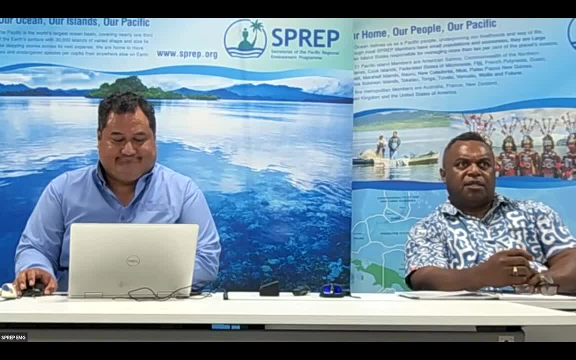 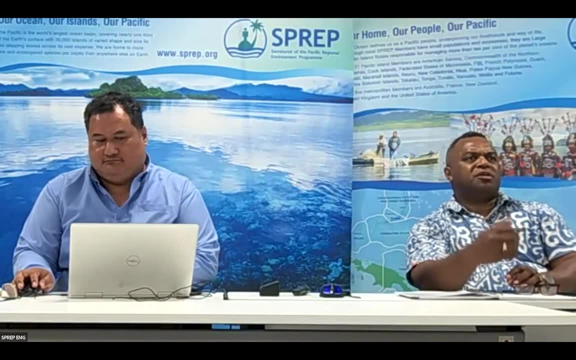 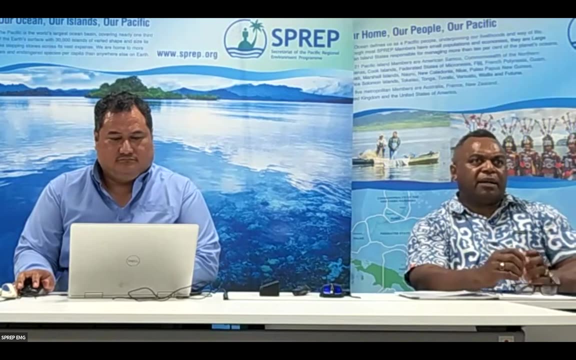 and again, it depends on, uh, the, the, the type of development once it's screened, when it's screened and if it doesn't require an eia. but what will be the question to us? what will be some other management tools to assist the regulatory agencies and and partners in monitoring that? 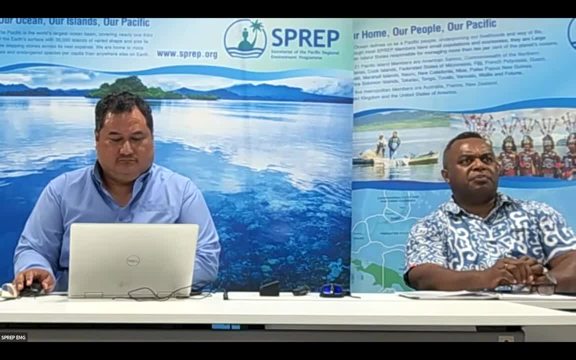 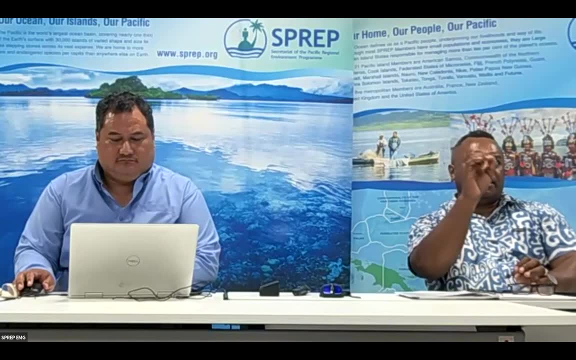 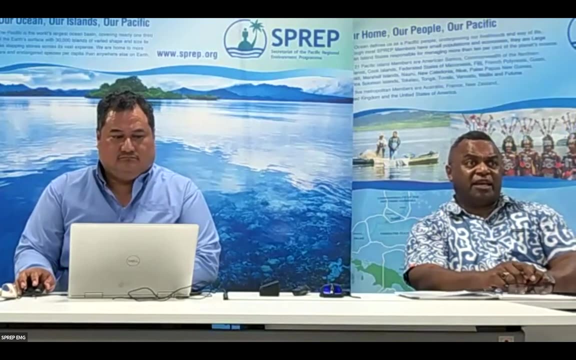 particular development. that's why uh, for in my experience so while working as a regulator, we always assist developers in guiding them on what should be a t-work or a cmp or emp should be about, even though it doesn't need a full eia, but still we need to guide them. so, again, 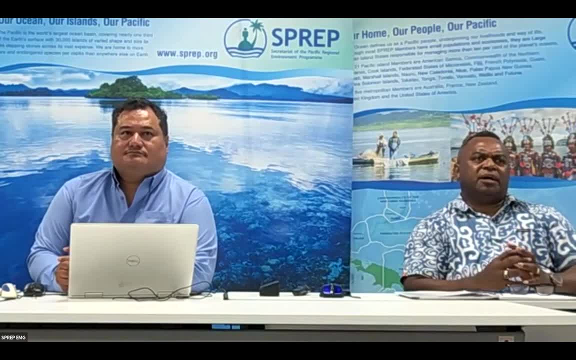 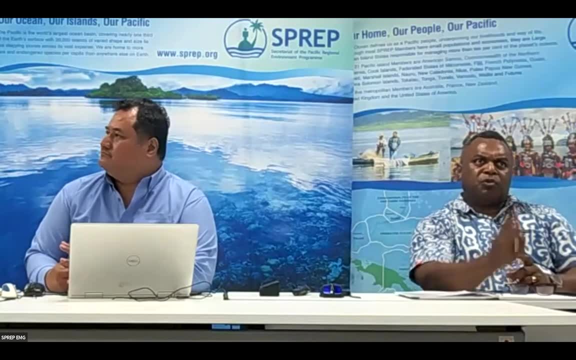 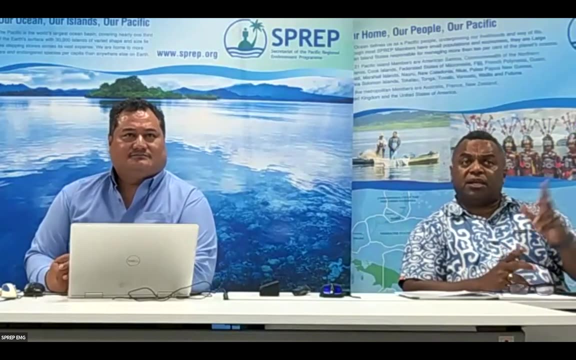 colleagues, it comes back to how we work together as a team, um, and how we, we, we- assist each other in protecting that environment and also promoting economic development. so that is, uh, my, my take my contribution to that, and there can be lots of discussion around this, because there in some 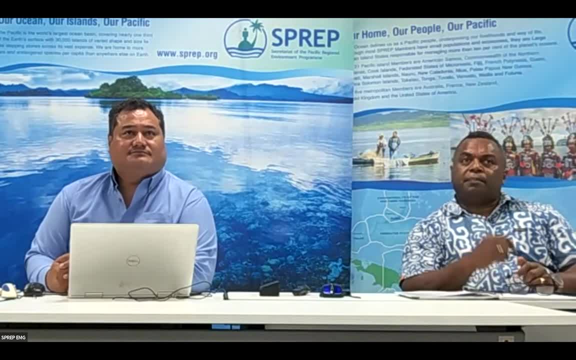 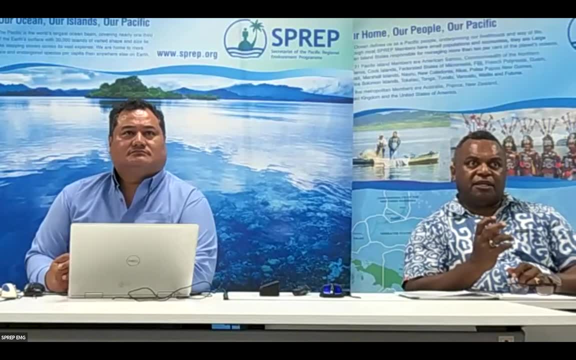 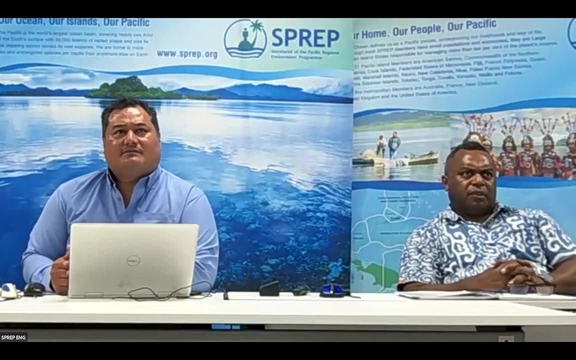 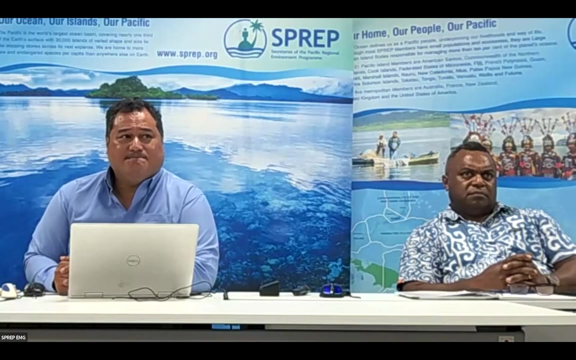 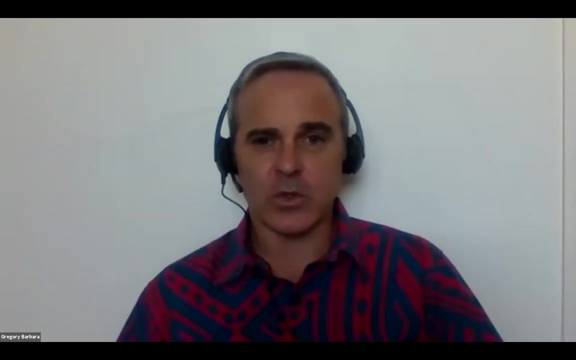 countries. they don't. this is not regulated. again, it's a management, a management or planning, planning activity for the regulator and the applicant. thank you, i've got a question from immaculate. does the regulating agency decide which project needs an eia? greg? um, do you want to respond to that? sure i did. i responded in the in the text to uh, to joyce there. 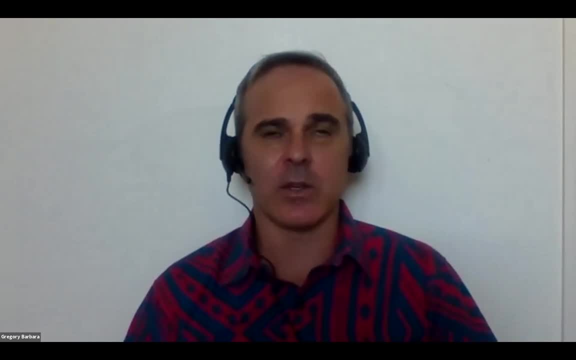 but, yeah, happy to verbalize: uh, yes, it's the authority, the regulator. whoever the authority is that receives the development application, they screen it and determine whether or not an eia is required for that project. so basically, they look at it, work out whether or not is it likely to be. 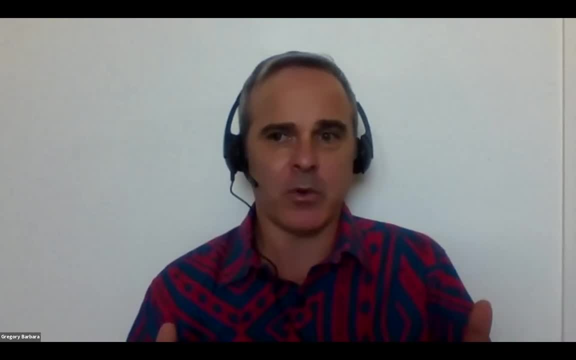 significant impacts, or if it's an unknown type of project with new technologies that have never been been done before on the island and they don't know how to manage it, then that would be another trigger for sending it through to an EIA. so, yes, it's the regulator who decides whether it needs. 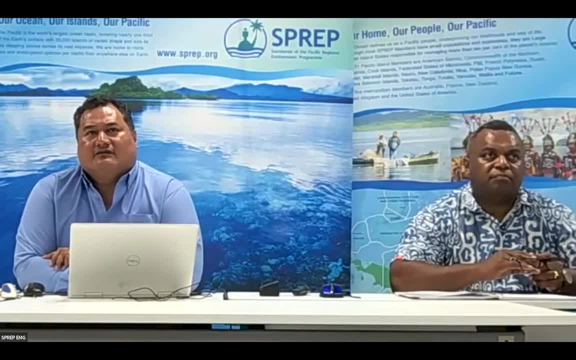 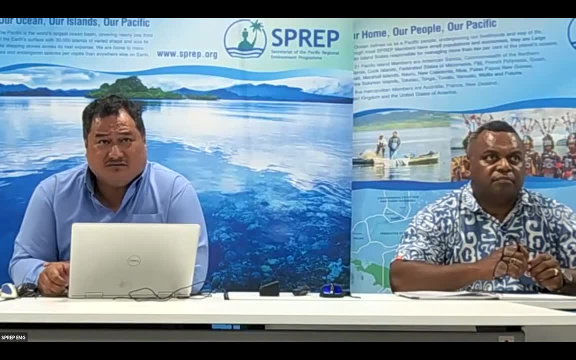 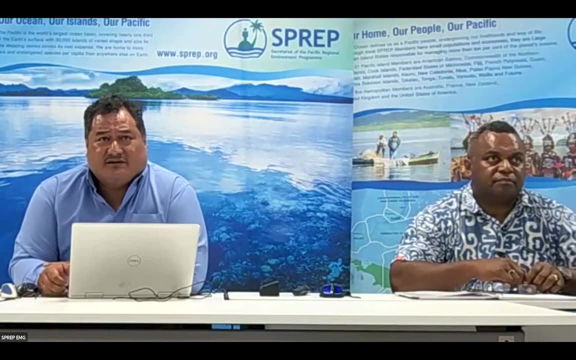 an EIA. no thanks, I've got a comment from Kisa Cooper from Insamoa: essential that the EIA consultant consults the regulating authority before starting at work, especially major projects. there may be updates to the requirements unknown to you, to the consultant, and also they can. 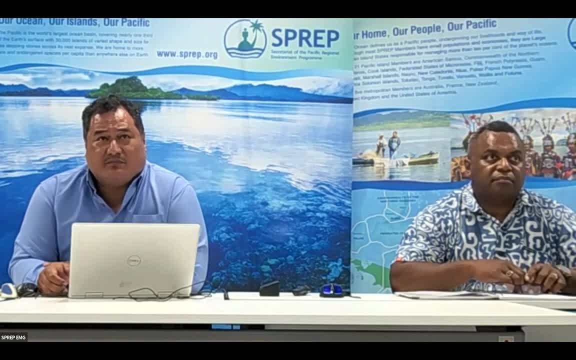 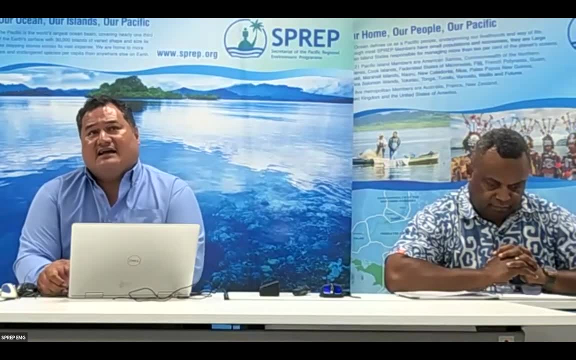 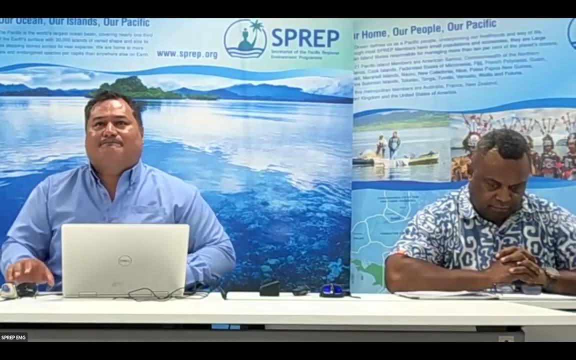 determine whether a preliminary environmental assessment report is required or a comprehensive environmental assessment report. cost and time saving. that's an excellent comment, Kisa. uh, yes, that's that. that's, that's very good. um, it's a it's a great point. yeah, it's a very great point. 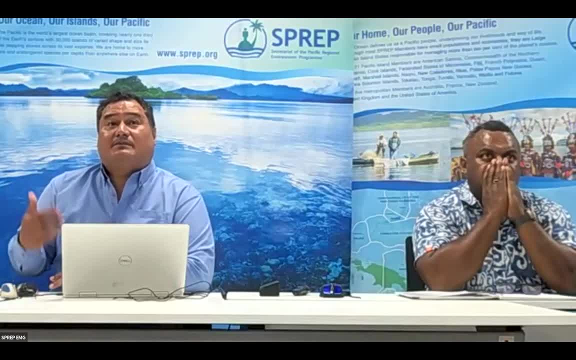 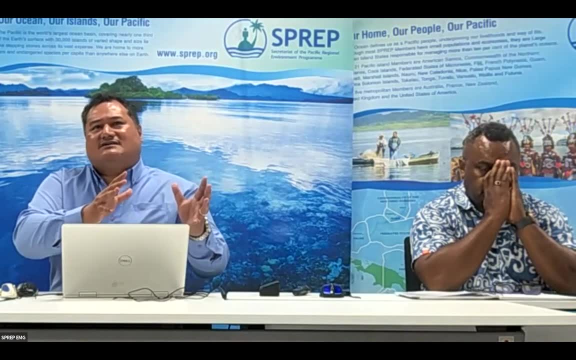 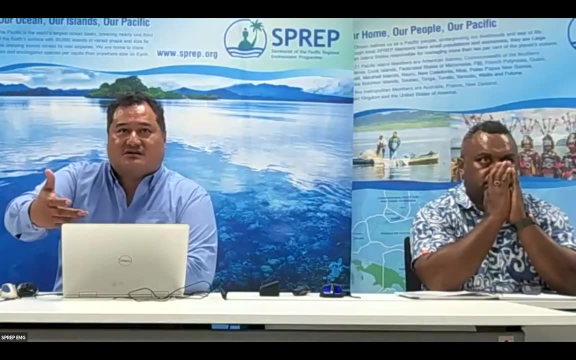 on risk the onerous. the onerous is on also developer to seek out the EIA uh regulating authority and ask questions. sometimes they think that it's the regulator coming in and there is that role. but you know, I think as a best practice for every developer, please do consult the EIA regulatory approach. it saves a lot of. 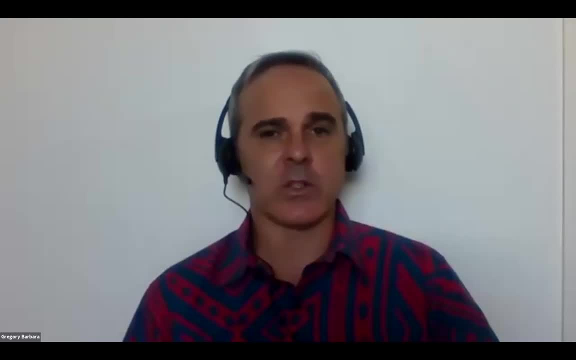 time going back and forth. if you don't, yeah, do it, do it as early on as possible. um consult with- I mean, we're all people when, um, the regulators- and I know most of the regulators across the Pacific and we've worked and I work with them- they're they're good people. 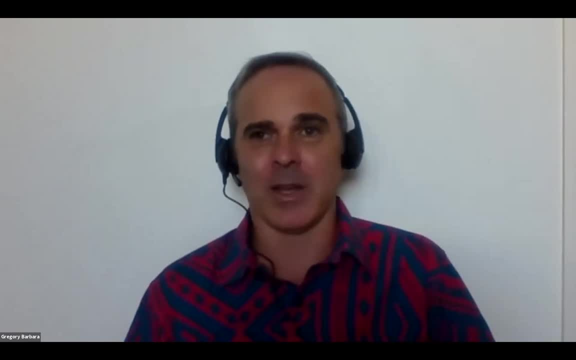 they don't want to make you, they don't want to make your life difficult. they, they, they want to know about your project, they want to help you do the right thing by your project. so, uh, consult with them early on. we've seen time and time again: in some of the countries the consultant tries to 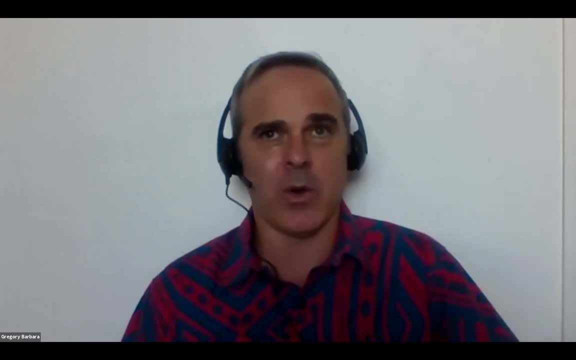 preempt what they think is going to happen and they go and write their own TOR or they produce an EIA without even submitting the development application. we've seen that and we've seen that happen in the Solomon Islands, unfortunately for a mining application, um, and then it's had to all go. 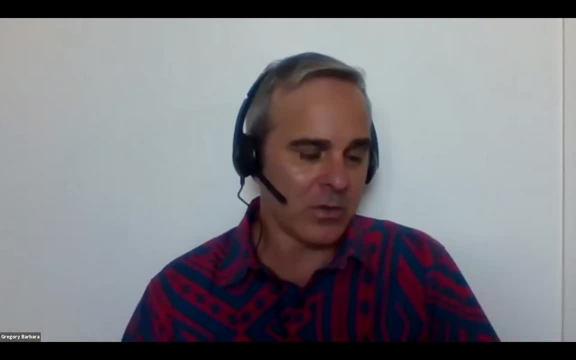 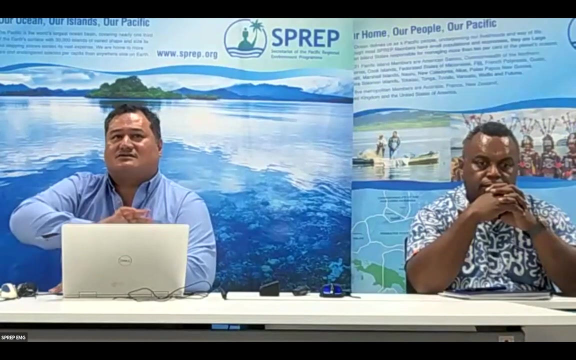 back and start from scratch again. so, yes, go and consult as um, as you said, go and consult with the regulator early on and they'll tell you what type of EIA or what type of approval pathway you're most likely to need for your project. yeah, one common thing across the whole EIA process is: 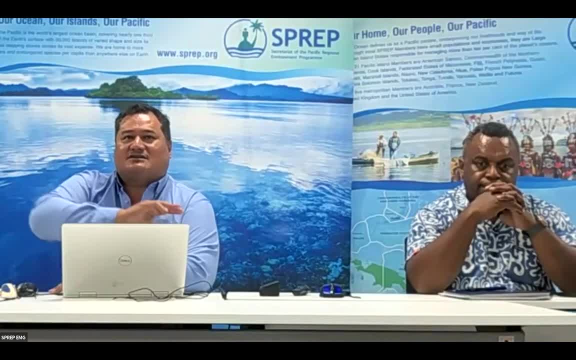 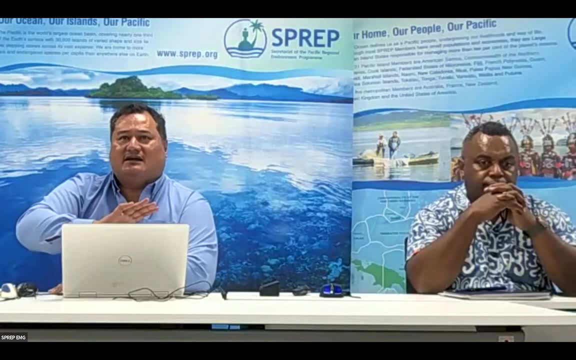 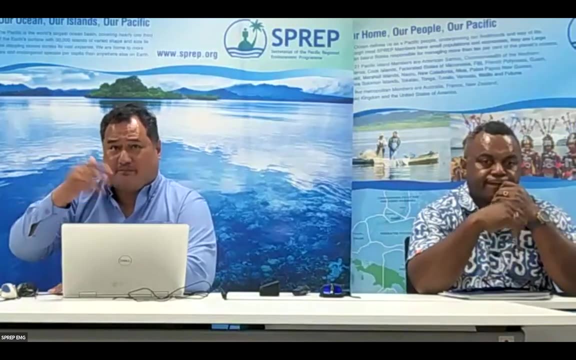 consultation. it's consultation with the EIA regulators. it's the consultation with other government departments. it's a consultation with local communities and local stakeholders. that's a common thing in a in a very healthy, very effective EIA process and it is a bit to benefit the developer, the, the, the, you know, the, the proponent. so you, you know. 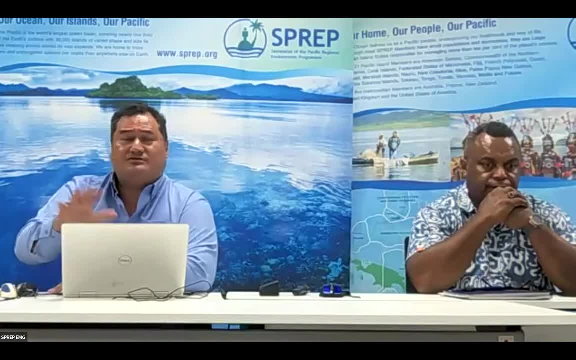 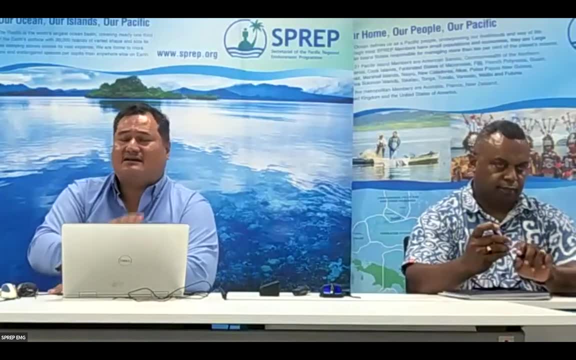 consultation reveals a lot of things that you need to know to make sure that you do not have to come back and readjust and and make changes. you know that you didn't plan for because, like I said before, it costs money and too much time. yeah, if you get it wrong, it's very expensive. yeah. 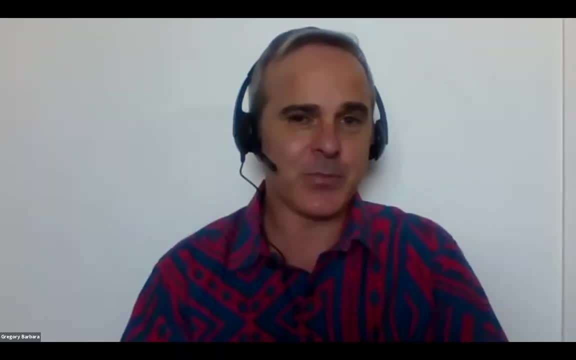 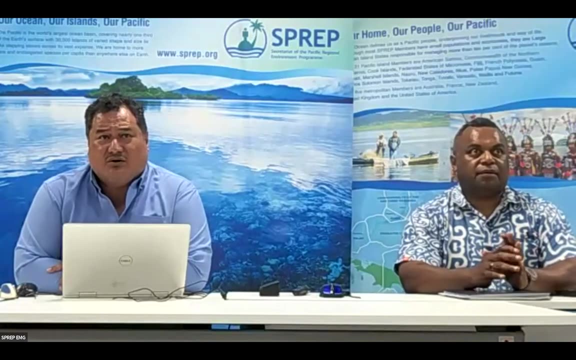 as Joppa. as Joppa said, consultation can save you money. all right then. uh, I'm looking at the chat box and I don't see any more comments. so, and I, and I think, in terms of time, we've uh come to the to the end of the allocated time. 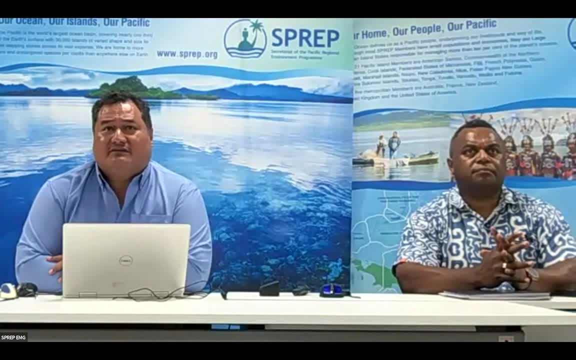 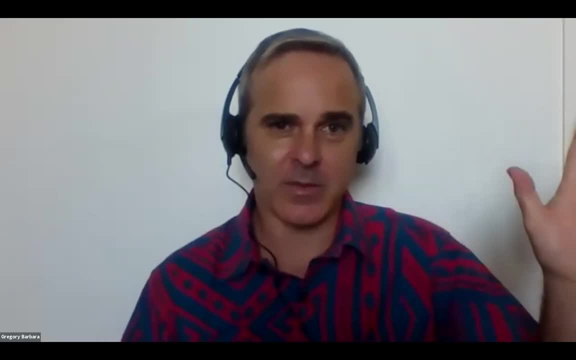 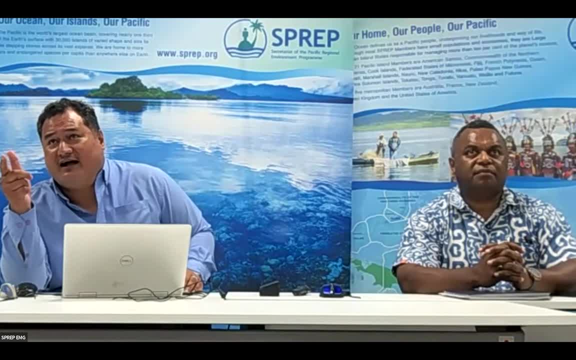 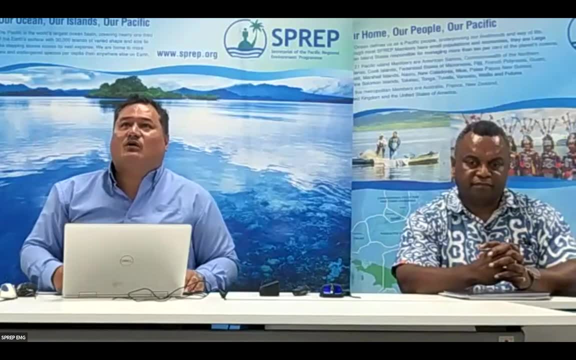 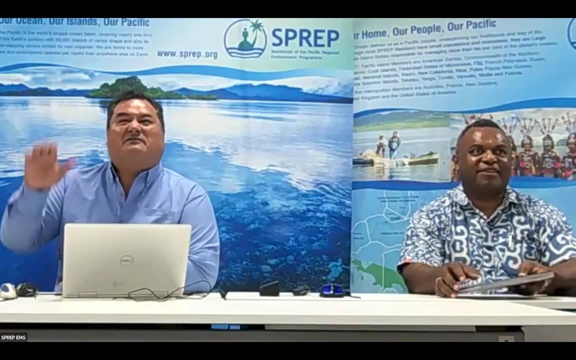 just see if we can brief. we broke the record. we've got 55, uh, today, sorry. so yesterday was 61. so we're shy by six people. so let me find out, maybe, maybe next week we'll find more, six, more people to hop on. but I think 55 is an excellent. you know, it's all right. 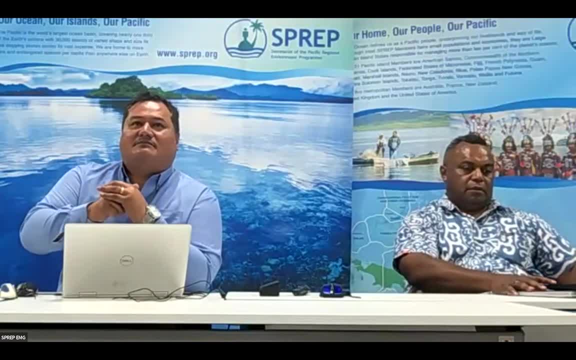 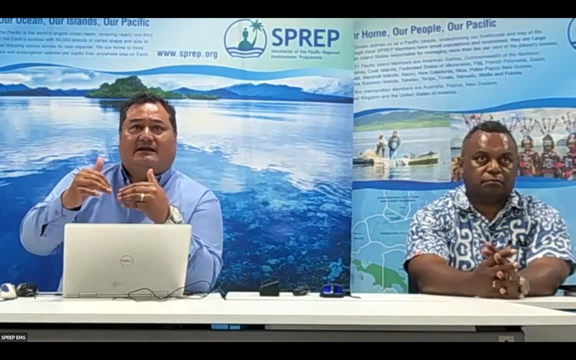 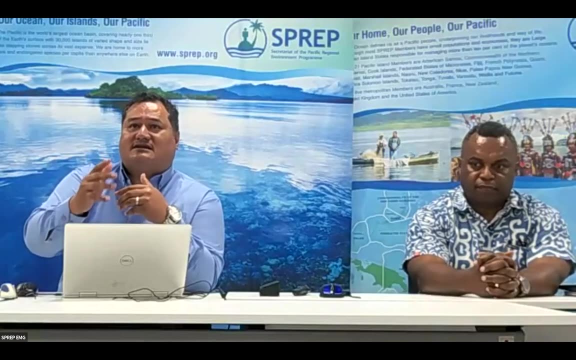 it's really great. so I just really want to thank all of you for taking time, uh available, enjoy, yeah, and uh. you know, having you here makes this more worthwhile, if and and meaningful, and we it gives us all that. uh training topics that we're designing here for you based on your comments. 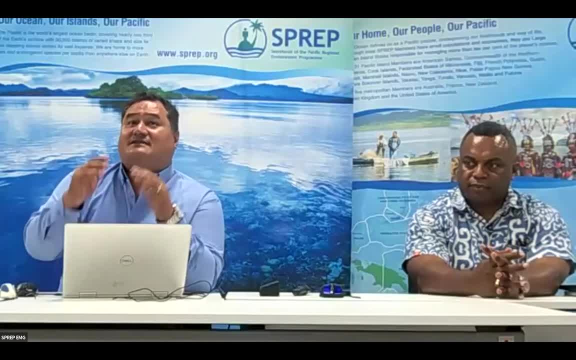 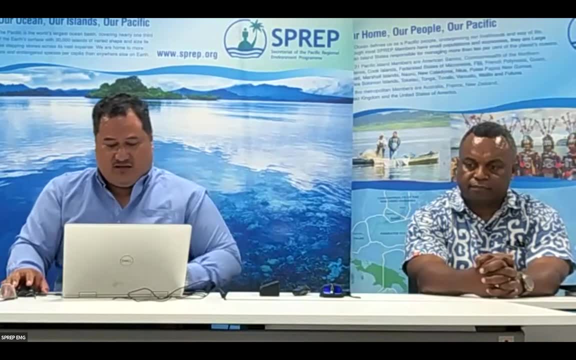 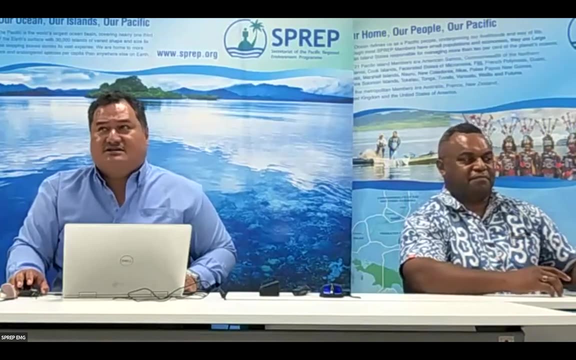 is exactly what you are asking for. you showing up, tells us that's that's the case. so I want to thank you all for that. we will continue this webinar. uh, next week we have module eleven and twelve. so So for next week, which is, I think, Wednesday and Thursday, the 27th of October, the 28th- 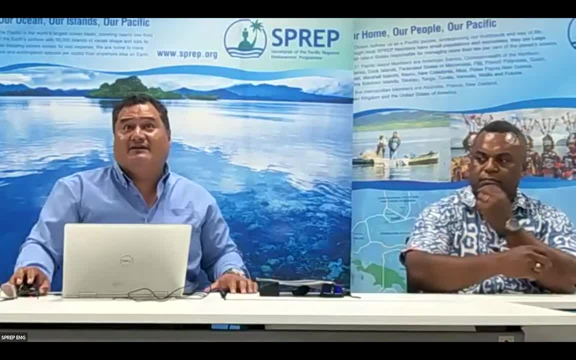 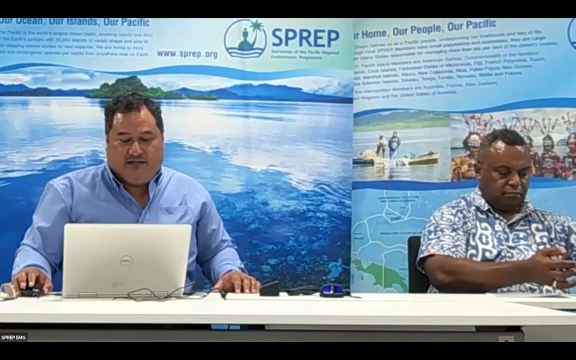 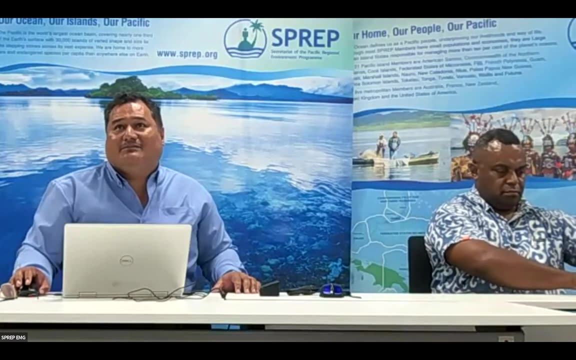 So let me just So. next week we have module 11. That's environmental and social management planning using the mitigation hierarchy and severity probability matrix for sustainable development in the Pacific. Well, I have my team leader in the base in Sydney, Miss Rachel Marburg. 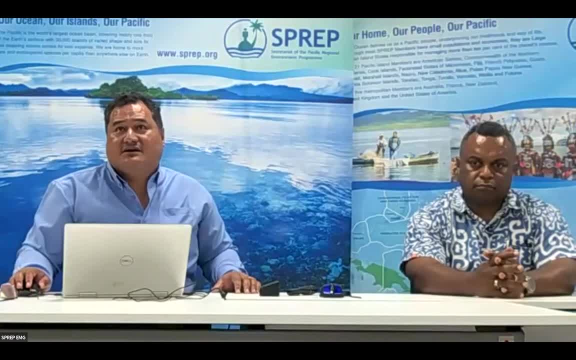 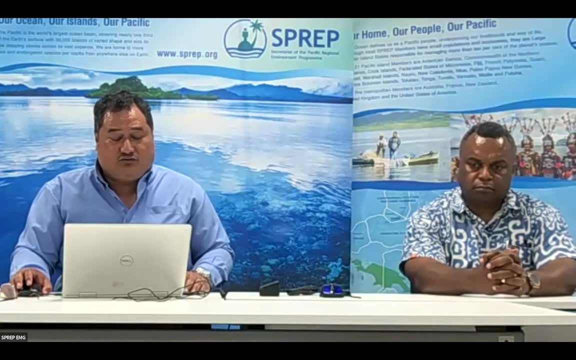 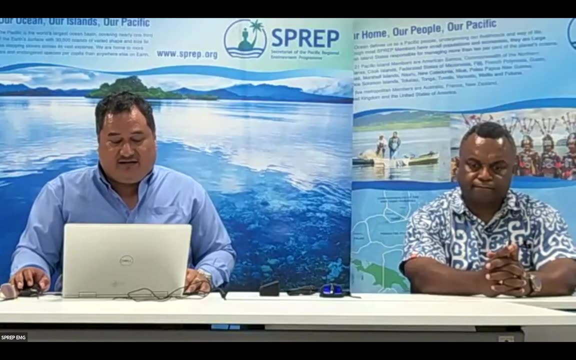 She will lead that presentation and hopefully others in the partnership will chime in Module 12, straight after Wednesday, Thursday: that is how to carry out a stakeholder mapping for engagement planning a case study in the Pacific. That will also be carried out by Miss Rachel Marburg from the World Bank and supported by Dr Hilda Sakiti-Wonga of the University of the South Pacific. 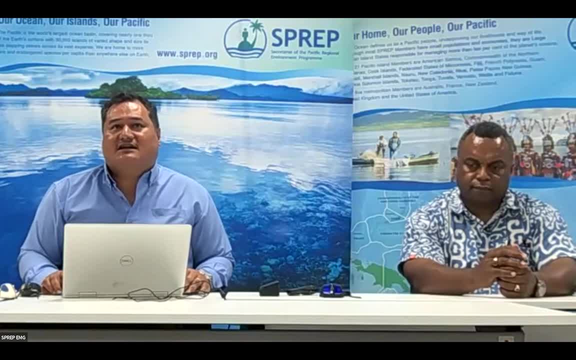 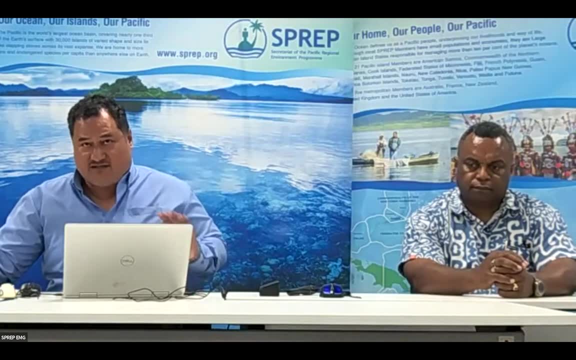 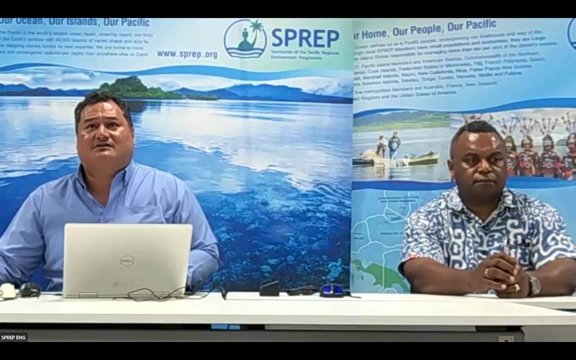 So please do tune in. We have some exciting presentations to show you. In the meantime, we will send out the evaluation for this module, together with the module yesterday- And hopefully please do take time to complete that- And we will send out training certificates for those who have completed them. 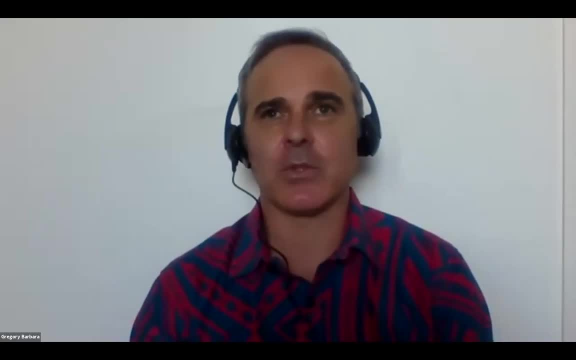 Do you have a comment, Greg? Yeah, just one more thing, And I'm sure you're probably just about to get to it. I know there's probably There's probably some questions that people will come up with afterwards and maybe we didn't quite address the question that you you had. 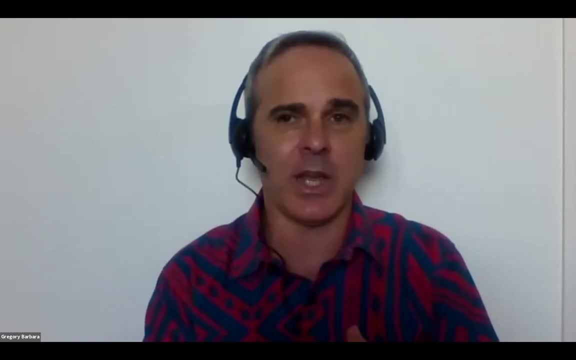 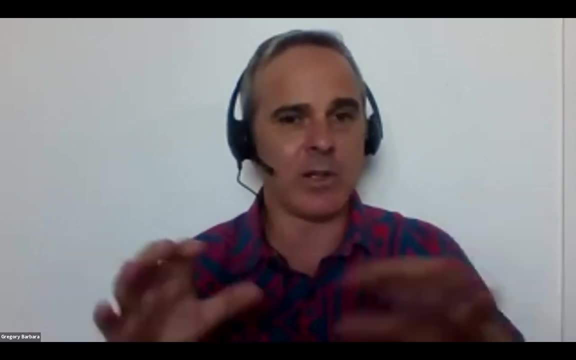 If you want to continue the conversation, log into the PNEA website, onto the Tullanoa, and put it in there and Ivan Joppe and myself will help to address it and as well as everybody else. let's continue the conversation in the Tullanoa on PNEA. 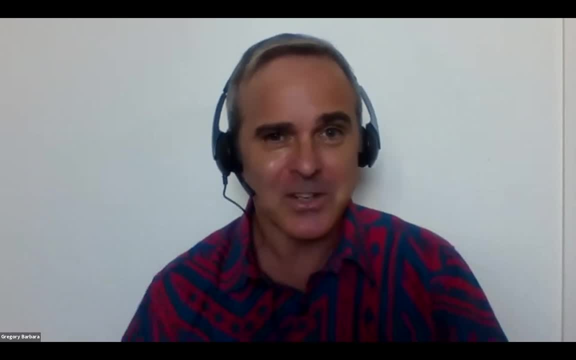 And if you're not a member of the PNEA yet, please register. Yes, please register. Good segue for my final point, which is the all the presentations. Yes, please register. Good segue for my final point, which is the all the presentations. 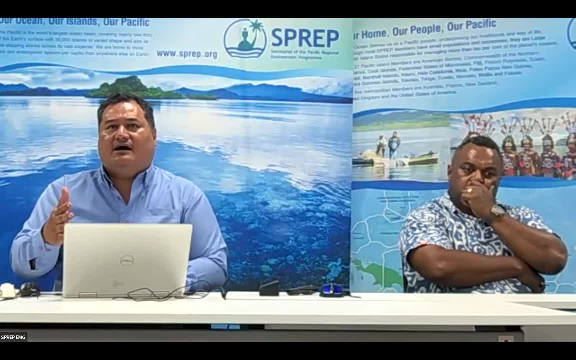 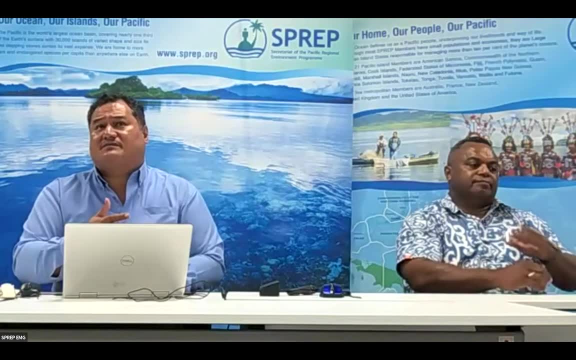 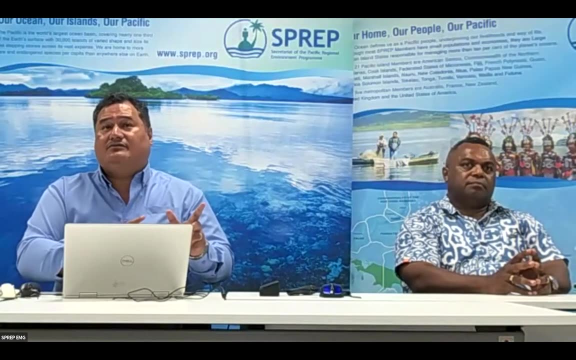 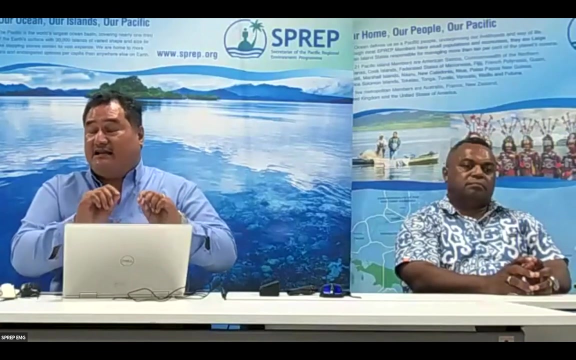 One of the presentations- The final presentations- Will be uploaded on the PNEA. They will be uploaded on YouTube. We have also the video recordings. Our Sprint IT comms folks are tidying it up and they will upload it on YouTube. and Ivan, who manages the PNEA- the key person here- he will notify you through the ENA, the PNEA email list, of the links. 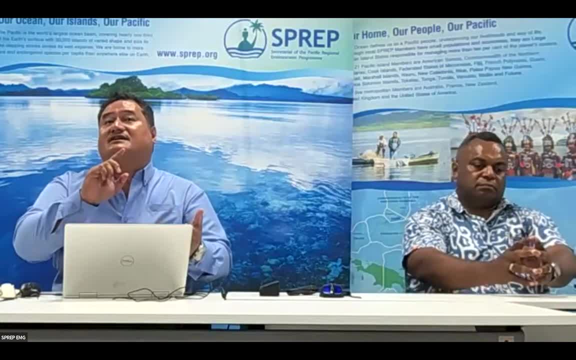 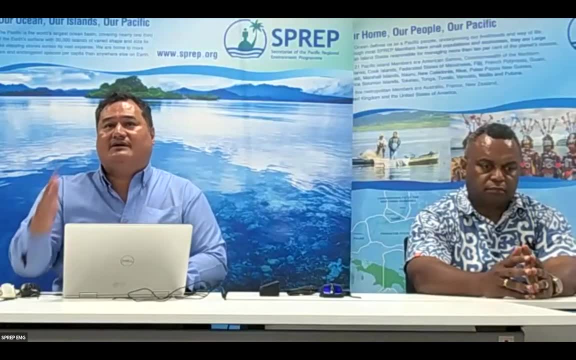 So you can go into it. Thanks, Greg, Thank you, Thank you. click on it so you get the powerpoint presentations and the youtube links. but if you're having problems, please do feel free to email me- ivan, joppe, rachel and others, greg, and we'll be happy.